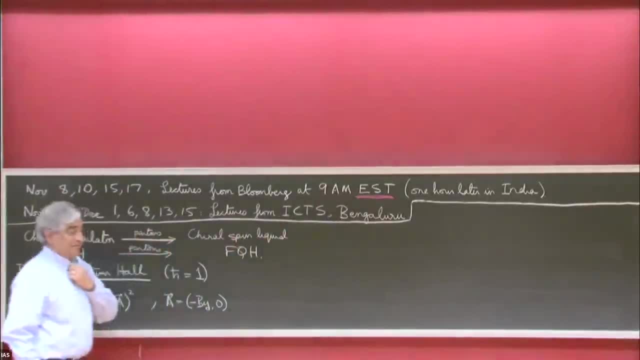 which is 9am Eastern Standard Time, which will be one hour later in India. So please be aware of that. Can you hear me, by the way? Yes, we can hear you. All right, great, Okay, And then so. 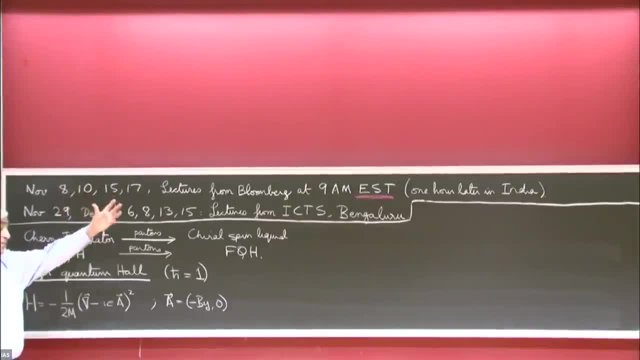 that'll be the next four lectures, And then there's a Thanksgiving week here in the US where I will not lecture during that week, And the week after that I'll be in India, in Bangalore, And I'll give six more lectures over there For a time to be determined- I'm not sure exactly when. 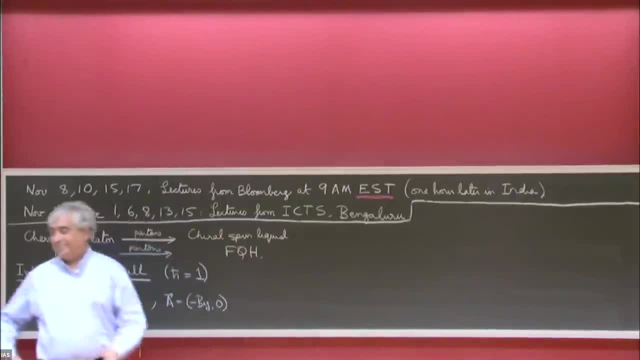 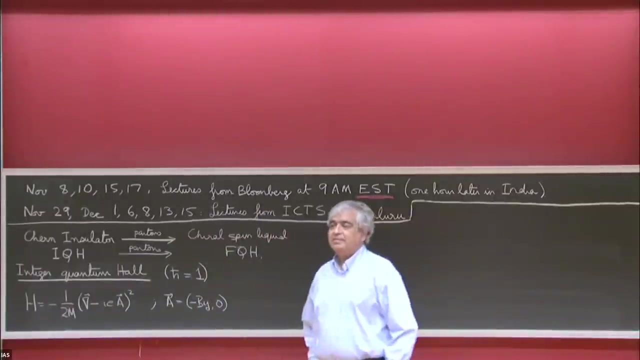 It may end up being quite early in the US, but you can be in here at home and watch it, Okay, Yeah, So in your previous lecture you discussed how you start from maybe some spin system and then go to the Spartan picture. Yes, For example, Chern-Simons description. 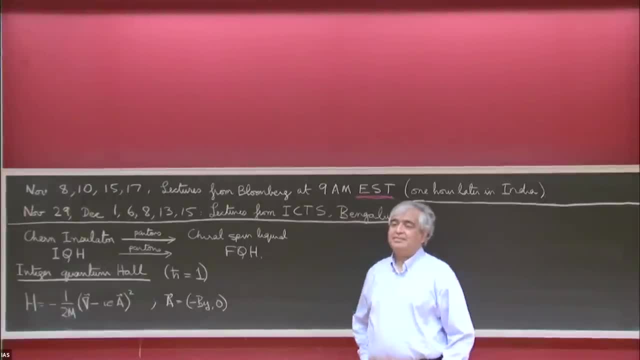 Yes, Yeah, And the chiral spin liquid, Right, Yeah, Is it possible to just go directly to the Chern-Simons description, Because that's what you really care about, right, The very known, actually, description, To go directly? I mean, you still have to solve the spin problem somehow. 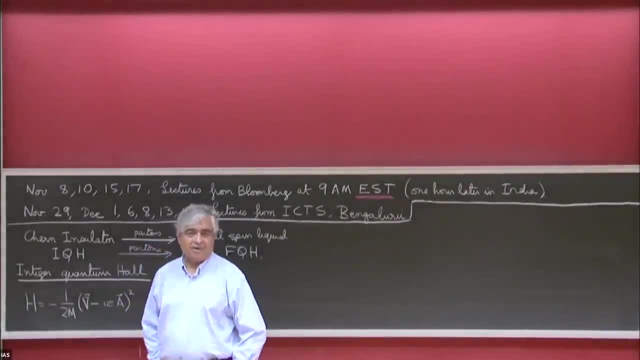 So another way to do it, which is, I guess, the way Laughlin and Karmar did it- you take the spin and you think of spin up as nothing and spin down as a boson. Then you can think of it as a. 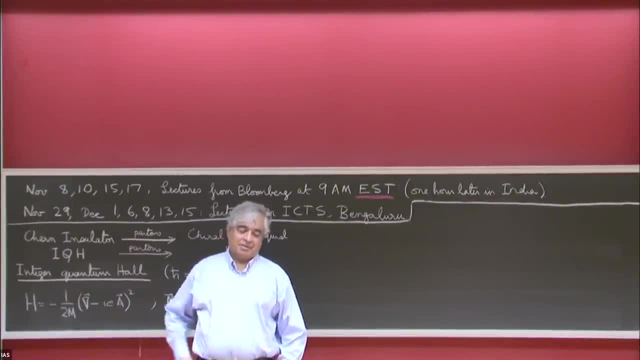 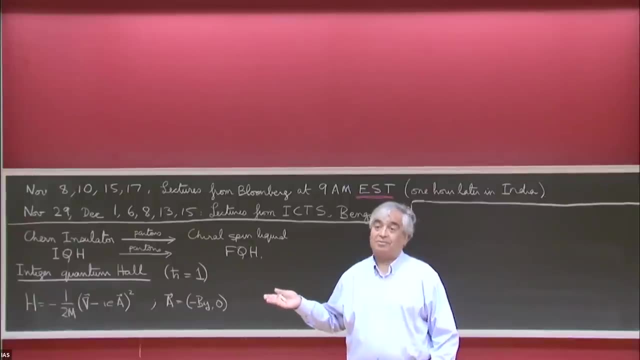 hardcore boson problem And then postulate it that the hardcore boson system should be in the nu equals one half fractional quantum holistic. Okay, Yeah, I'm just thinking of theories like, for example, the CPN model where you have an immersion gauge field, Right, 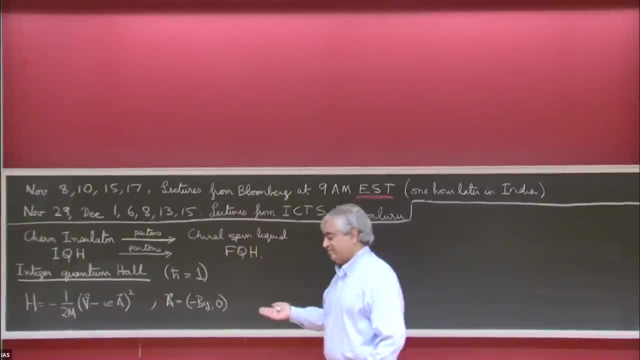 Well, that is exactly what we did, right. We wrote the spin in terms of fermions, Yeah, And I realized that there was the intermediate step of the partons. Well, anyway, Yeah, Well, the partons, I mean, the CP1 theory is also a theory of partons. 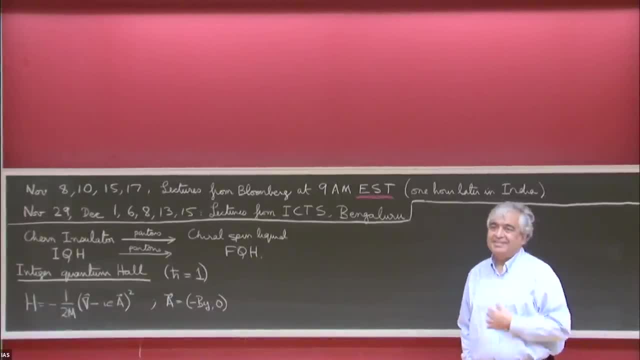 because the z particles have a gate charge. It's also a theory of partons, The physical operating, the CP1 theory. the gauge neutral operators are spins z, star sigma z. Those are the spins. Okay, So we're not doing anything different from the CP1 theory, in fact. 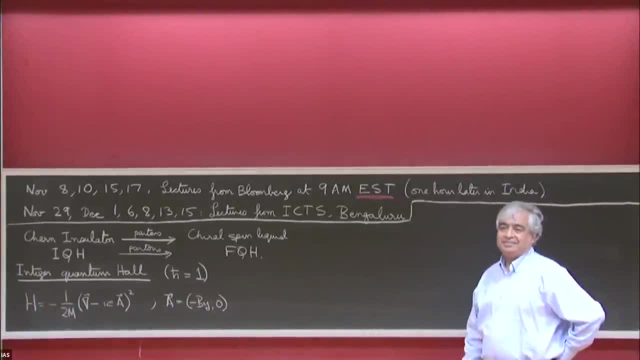 Yeah, There's no gauging. The z's are not gauging variant objects. So similarly here, the partons are not gauging variant. I had to put the partons in a churn bag to get the churn silenster. 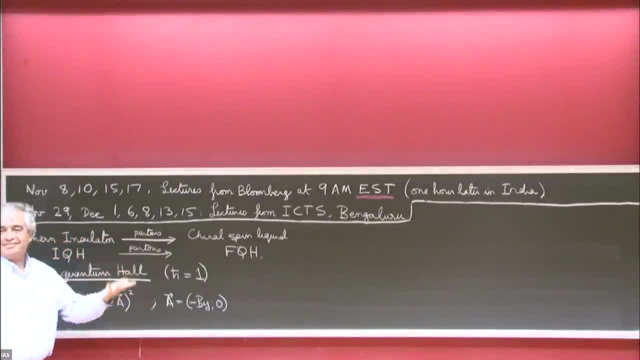 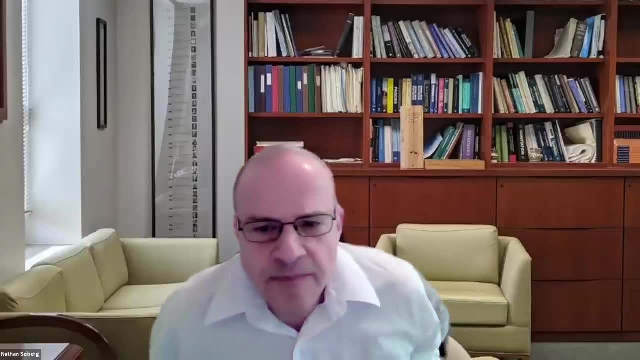 But, as we'll see today, you could equally well put them in a magnetic field, and it'd be very simple. I also have a question from last time. Yeah, go ahead. This is the role of time reversal symmetry. Was it there microscopically and then was? 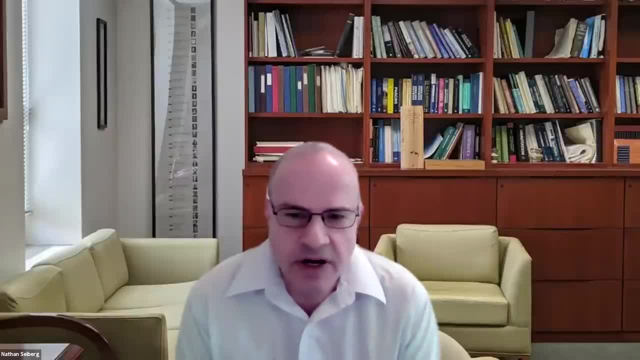 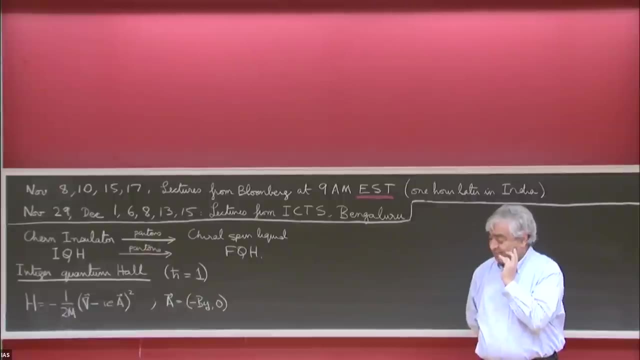 spontaneously broken or was it explicitly broken? And if it is spontaneously broken, are there any consequences of that? Actually, the first question is: it can be either. It can be either spontaneously broken or broken explicitly by the time. reversal symmetry: Yeah. 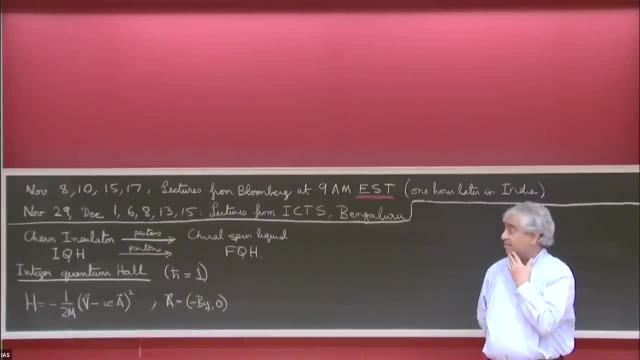 Okay, Yeah, Yeah. So if it's been broken explicitly by the Hamiltonian, it won't make any difference with the theory of the phase. That's the phase where you have of the chiral spin liquid. you get exactly the same theory in terms of the quasi-particles and all their properties. 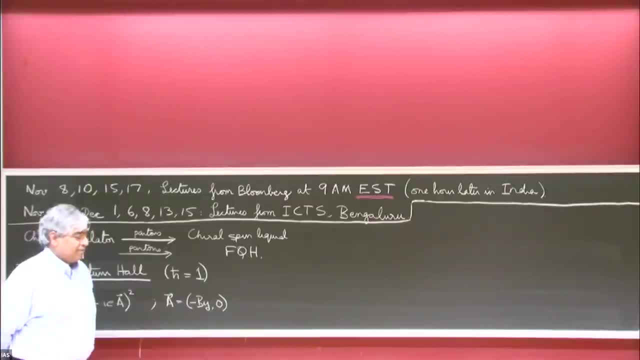 and the edge state properties. But if it's been spontaneously broken, well there is a scalar which is gapped, And that only becomes important near a phase transition. So suppose there's a phase transition where the Yeah symmetry is being restored, And then you would have to worry about the fact that the 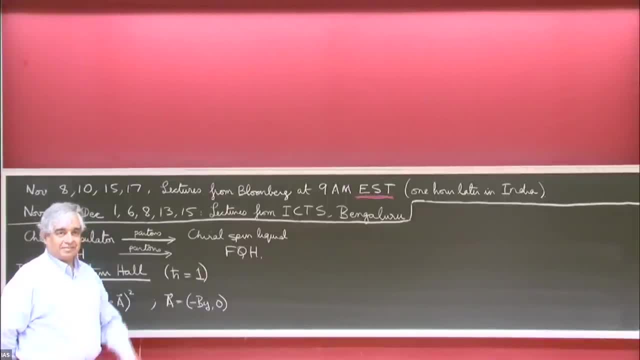 time reversal was spontaneously broken And there will be extra fields associated withlight fields associated with the fact that you're restoring the symmetry. So that would be an interesting point of phase transition which I haven't addressed. You first have to decide what. 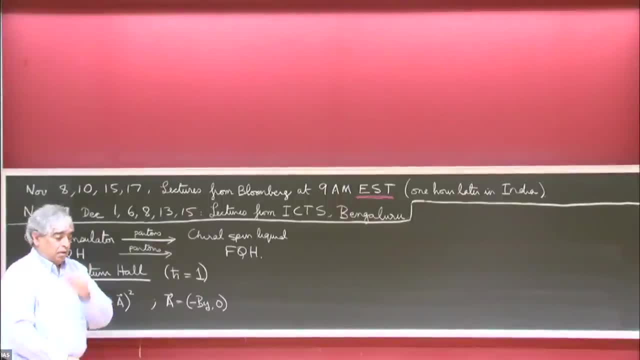 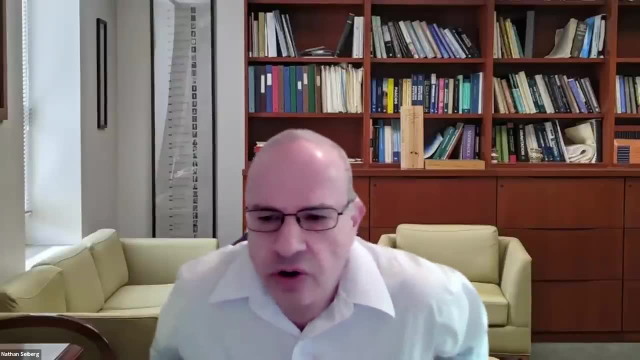 the other phase is on the other side that you're going to. Are there any? But if it is spontaneously broken, won't there be domain walls where you have the different vacua or the different The two sides, without going to a phase transition? 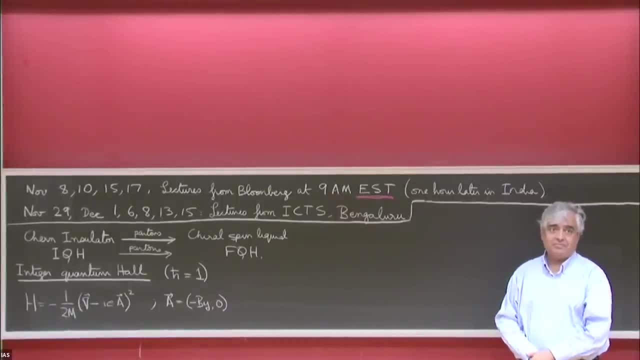 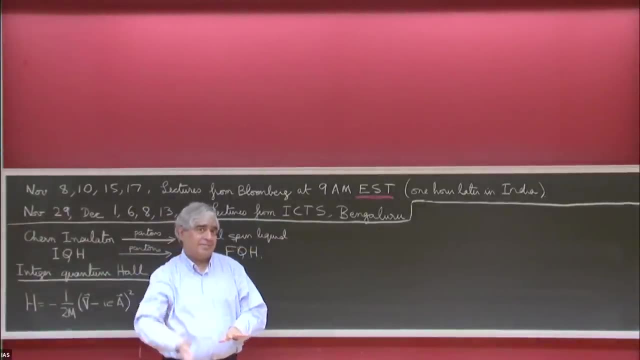 You're right. Yeah, there could be such a configuration. Yeah, So that would be like going from churn plus one to churn minus one, And yeah, then there'll be some edge states in the domain walls for sure. Yeah, Okay, Thank you. 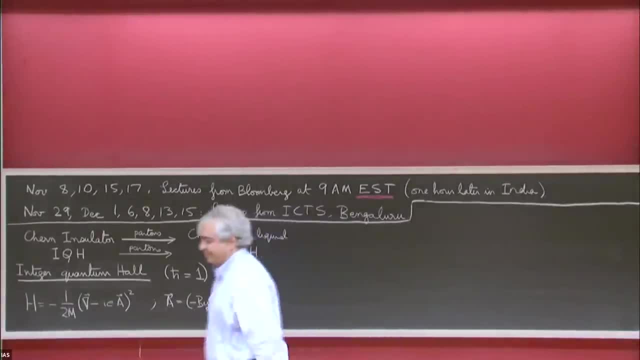 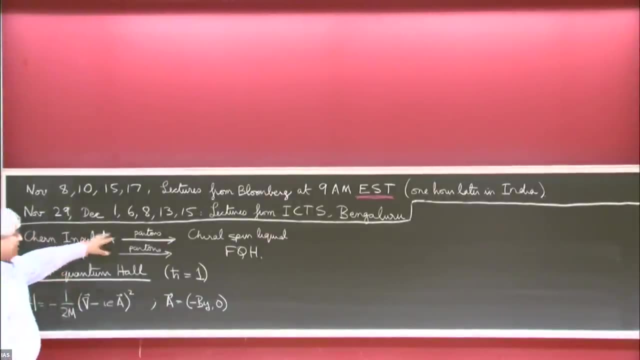 What were you saying, Tom? Exactly Okay, Yeah, All right. Yeah, That's correct. Sure, All right. So we talked about this connection and which we've just discussed. Are there any other questions? on the last lecture on the churn insulator and the corresponding liquid: 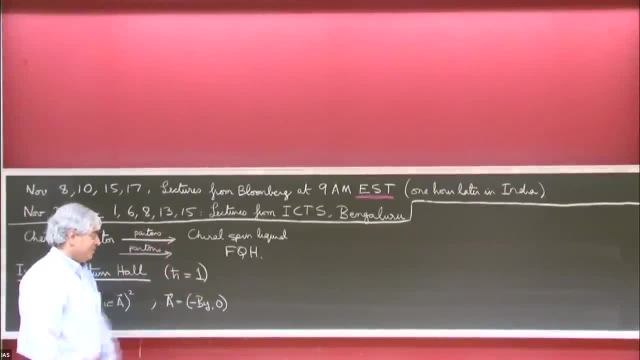 I've updated the notes on a lot of that on the website, So please download the latest version, and all the details on how the churn number is quantized and how it relates to the Chen-Simons term or the Hall of conductivity are in the notes. 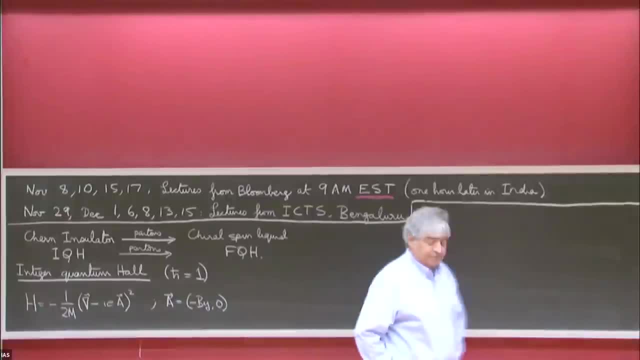 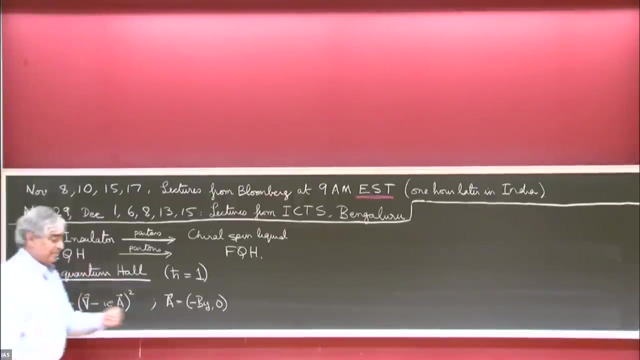 And the detail will be on the slide where we go into that in just a minute. Okay, All right. So today I want to establish the same connection but in a slightly different setting. This is the setting of the quantum Hall effect. So now you have electrons moving in two dimensions. 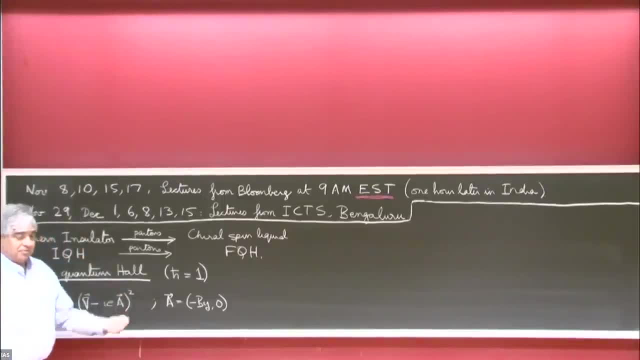 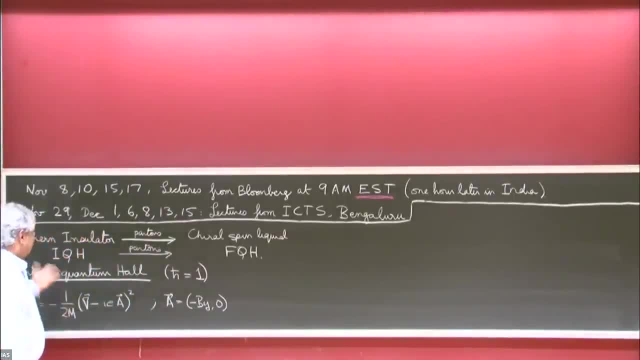 There's no such constraint And initially we'll just take three fermions moving in a magnetic field That of course leads to integer quantum Hall states, And then we'll do a part on description and describe a few fraction quantum Hall states And hopefully, given all the stuff we've already covered, 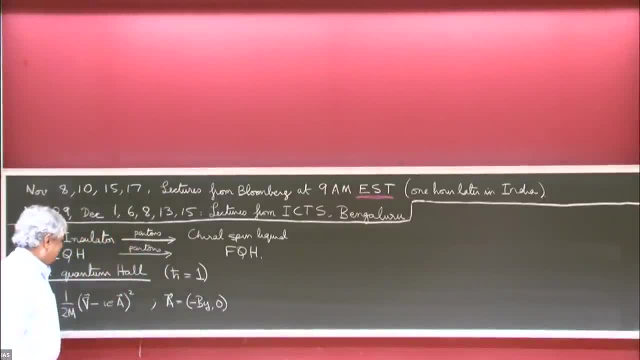 this will be relatively straightforward, as you see, I hope. Okay, so we consider the integer quantum Hall case. I'm gonna take h. bar equals one. This is important because many results are expressed in terms of h, not h bar, So always remember it's h bar, that's one. 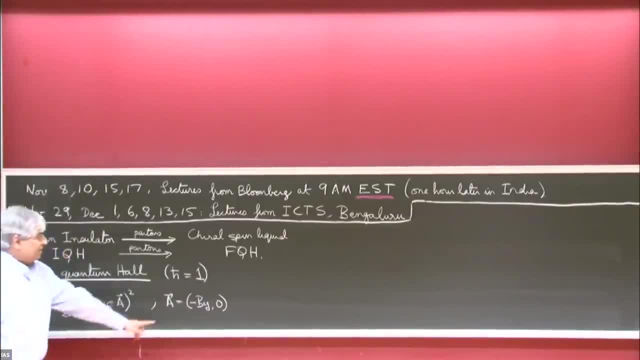 Okay, so this is just a free particle and a vector potential. I'm going to use this particular gauge because that will be useful when we look at the edge states. So that's what I want to do today is also explicitly show you, in this case, 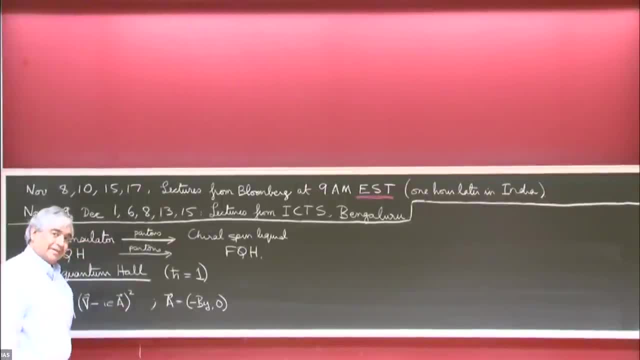 it's a bit easier, as was shown first by Alvaren- Actually before TKNN- that there are, you know, chiral edge states on the integer quantum Hall system. Okay, so now we just go ahead and solve this equation. I'll be very quick about it. 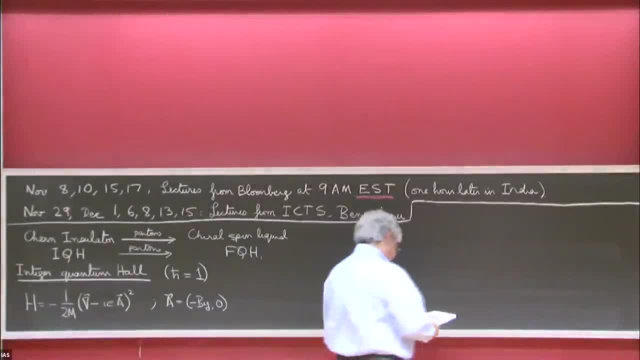 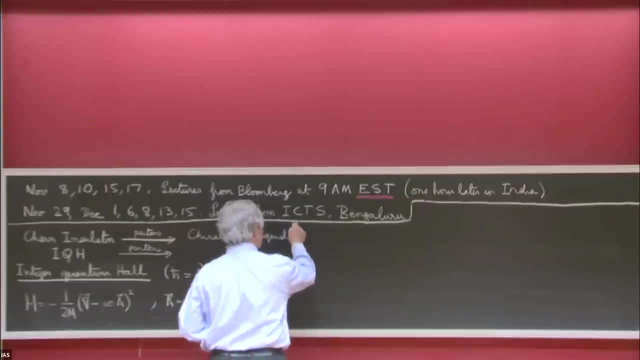 I presume most of you have seen it somewhere. It needs to land our levels, So let's put that with notation. We introduce something called one of the various quantities that you will see if you read papers on this topic. There's something called the cyclotron frequency. 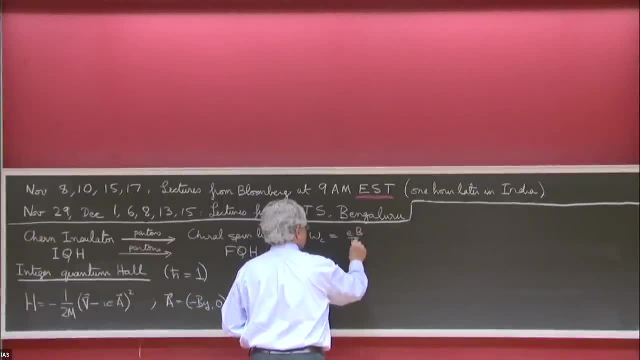 which, in these units, is E-D over N, and there's a magnetic lens which is one over square root of E-V and also one over square root of M over C, and then you can introduce a dimension that's coordinate in terms of the magnetic lens. 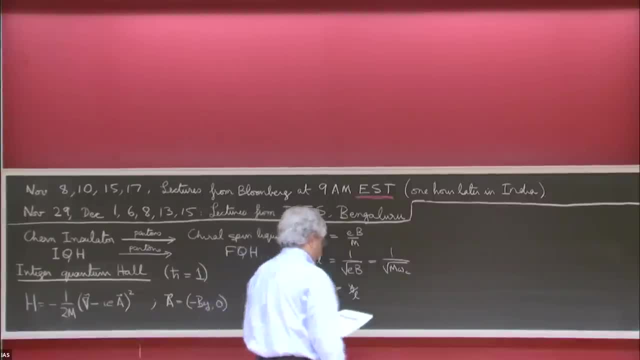 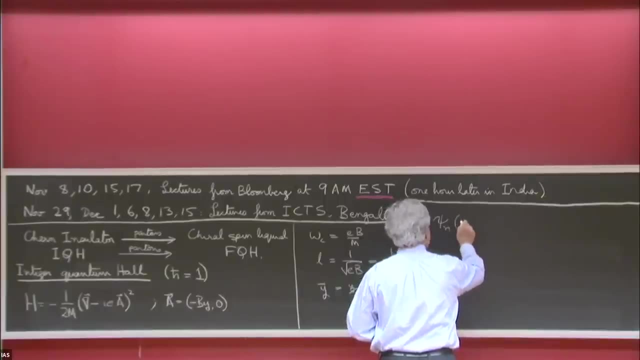 y bar is y over L. and then if you take your wave function- so I can have a little lecture on that, we're going to get a very nice- and the function of X and Y. Well, since you have translational symmetry, 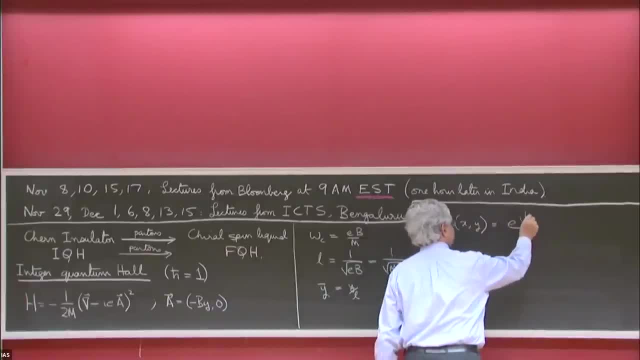 in the X direction. it can be a plane wave in the X direction And it will be some function Y of N and K which will depend on Y, And this function just obeys the equation of the harmonic oscillator. So in appropriate units, 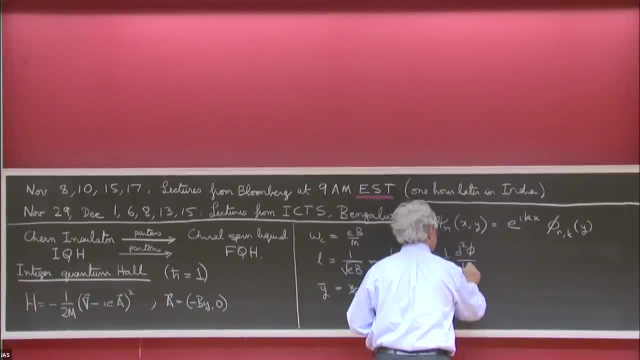 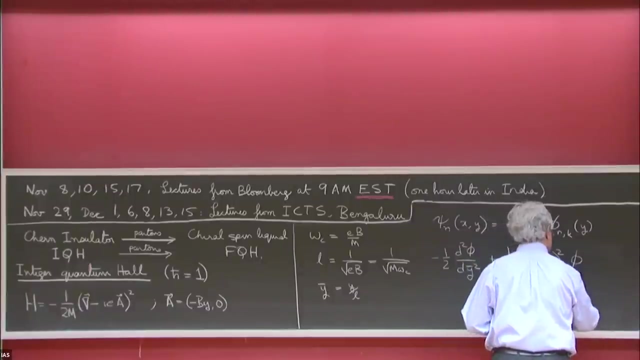 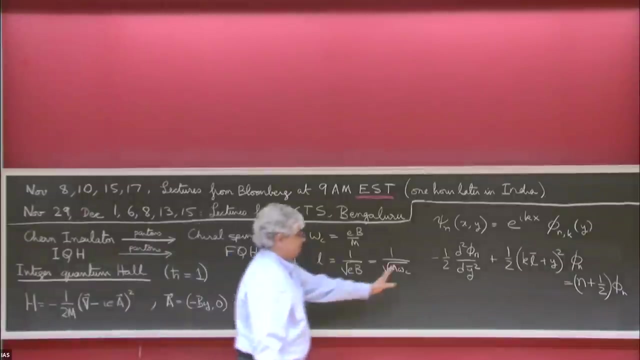 T squared by Y, bar squared. that's one. Okay, I've gone ahead and also written the eigen energy, because it's kind of clear. Okay, so we just insert this answers in this equation And this is what the Schrodinger equation becomes. 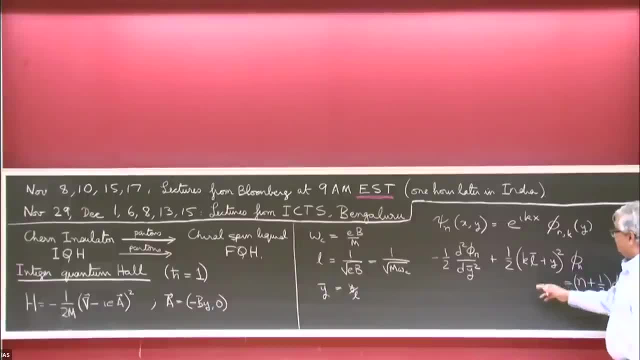 This is the Schrodinger equation of a harmonic oscillator, But the key point here is a shifted harmonic oscillator. As you change the wave vector in the K direction, the center of mass of the harmonic oscillator shifts with K. So momentum in the X direction is the same as coordinate. 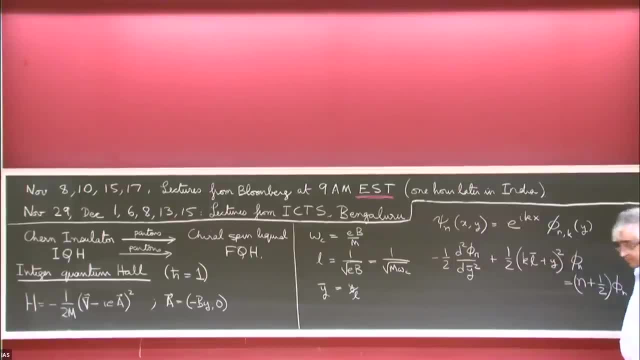 roughly same as a coordinate in the Y direction. So that's a very useful semi-classical case. So that's a very useful semi-classical case And it's a very useful semi-classical picture to keep in mind. Sorry, what's L bar? 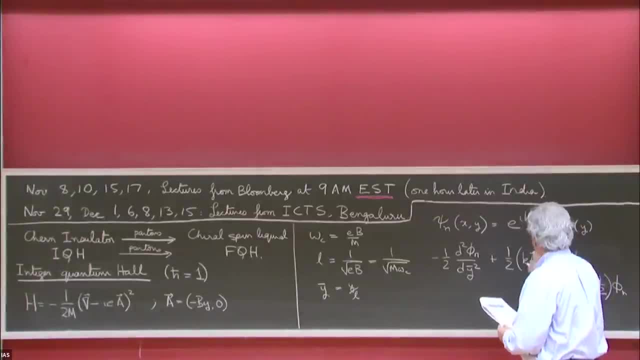 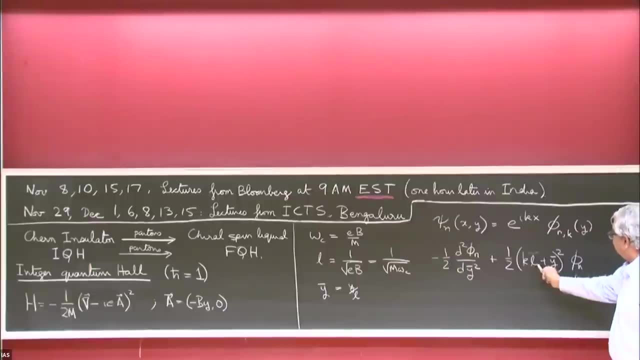 Maybe it's L squared, perhaps, Yeah, Or it's Y bar, Or it's K L. thank you, Yeah, so K here, K? L is dimensionless, Y bar is dimensionless, So it's all all right. Okay, so the very important property of this equation. 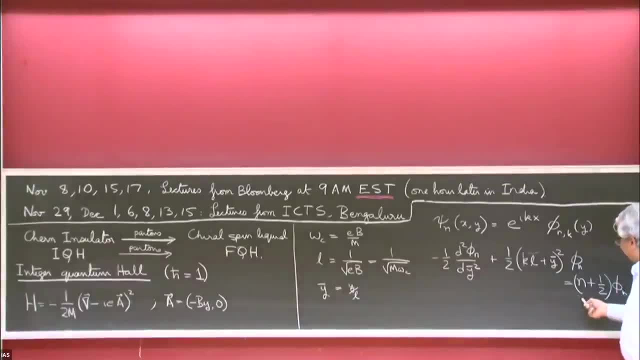 which is different from the channel insulator is that the energy, the eigen energy, that is a harmonic oscillator states, And here of course you can see the N: zero, one, two, it's an integer. The energy is completely independent of K. 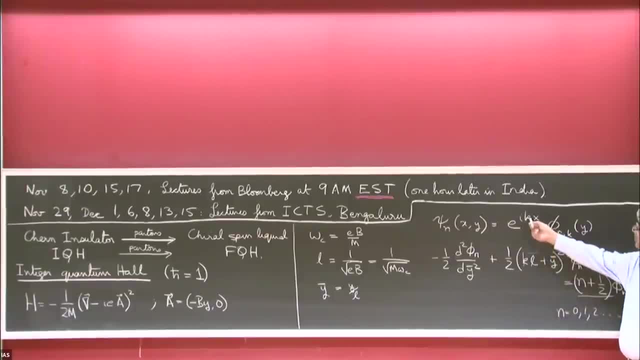 So we have a very large degeneracy of states. It's independent of K, there's no dispersion as a function of K, And that's very different from the channel insulator. But it's a simplified feature, but in many ways it's also a confusing picture. 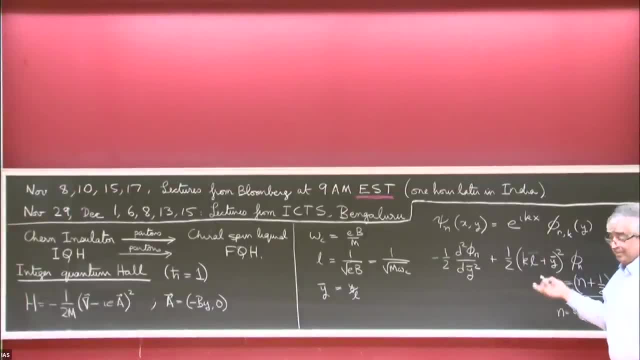 because it makes the band flat and things like channel number are not so easy to define. So you can imagine a more general problem problem that you added a very small theory potential here and then it'll become exactly the same set of problems that you solved there, but that the algebra becomes more complicated. 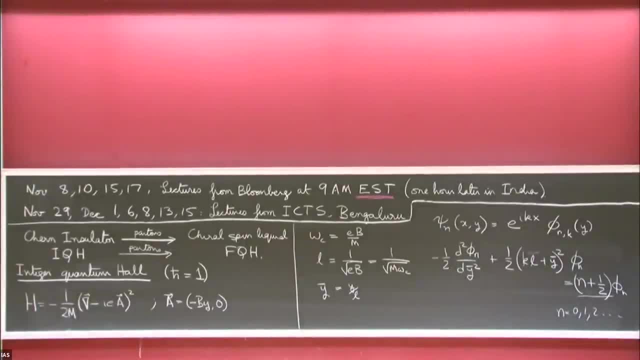 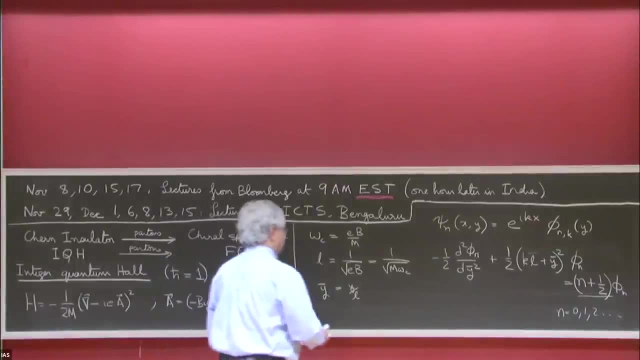 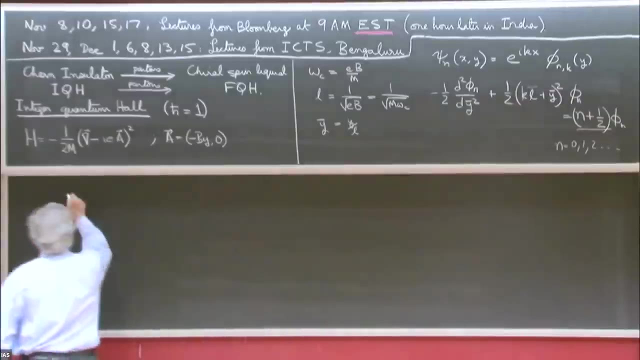 and you have to go and drop theorem and all of that, Anyway, Okay. so then the question is: what is the degeneracy of the states? So this is the other important point. So if you take a geometry there, so let's call this: make sure, okay. so this is Lx and this is Ly. 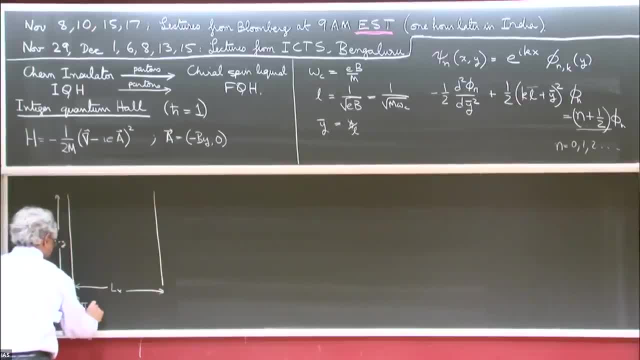 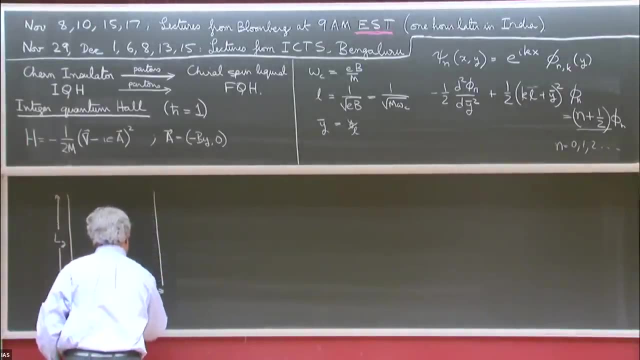 My k is some integer multiple x over Lx, And then the central mass coordinate here, y bar, is. so the average of y is of course then minus kL. So the way you can think about this is that you have a whole bunch of 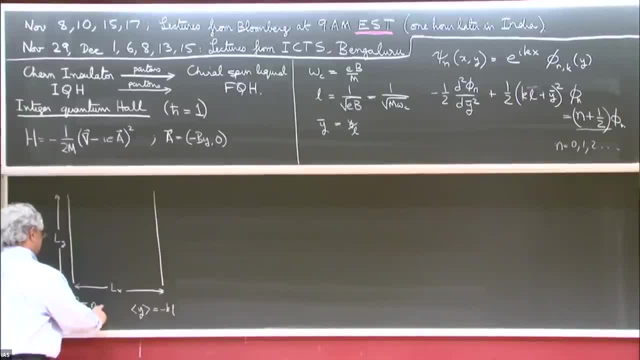 states, and then you have states where k is positive, then y would be negative. So there's a scenario that I've already solved. so you just need to love p sometimes and it only states that are running here with very large momentum, and then you have states with smaller. 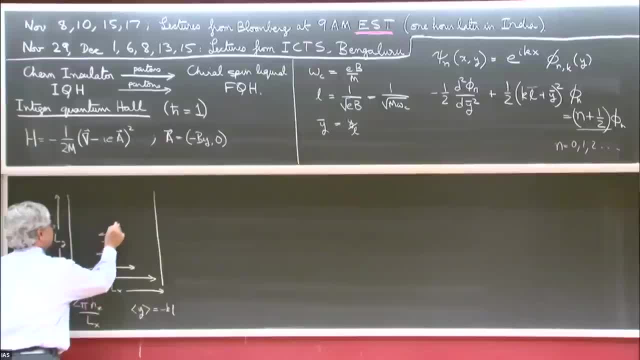 momentum, which, so this is just the basis of states. uh, the larger the momentum, the more the negative y coordinate and they're basically, uh, gaussian functions about in the y direction, harmonic oscillator functions in the lowest level of their gases. okay, um, so another important point is that 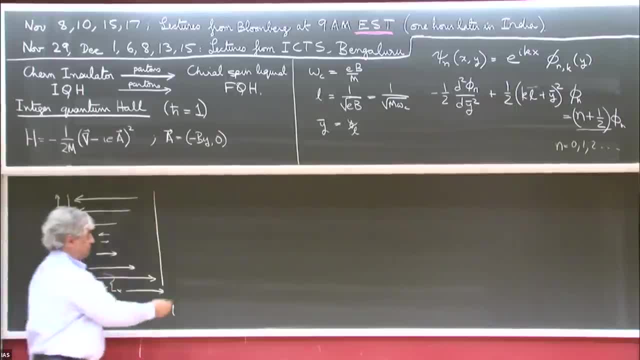 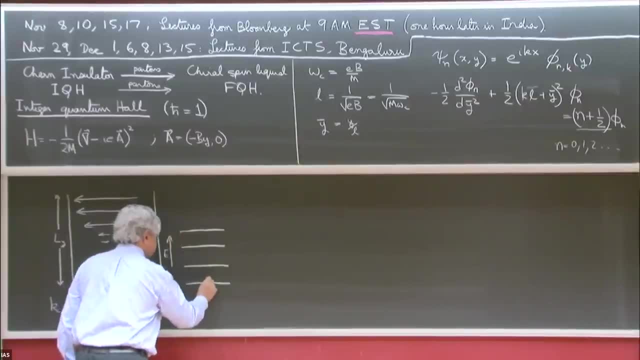 if you well occupy, say, the land level. so let's say: here are the land levels, this energy zero, one, two, three. if you occupy all states in the lowest land level, which is the most important case we'll be interested in today, uh, then you occupy all of these states and, in fact, 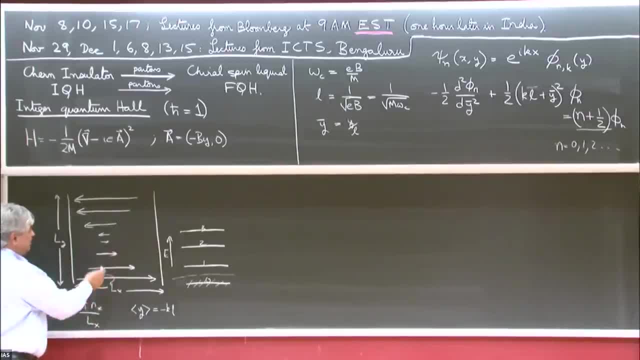 at any point in the center, the net current is zero. uh, if we just compute it carefully and start another, notice that there is no current. so, uh, if you pick a point here, you get a current from here and there and they all cancel out. uh, these are just. this is a set of bases that you've chosen to describe. 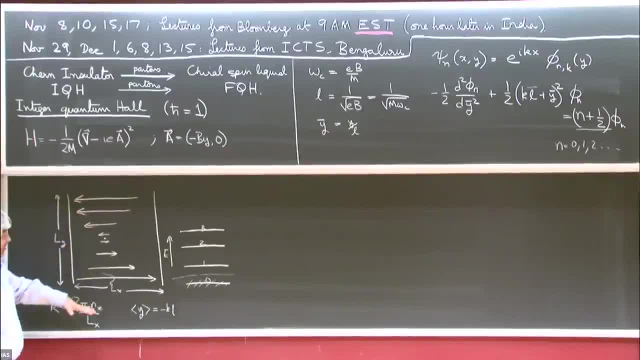 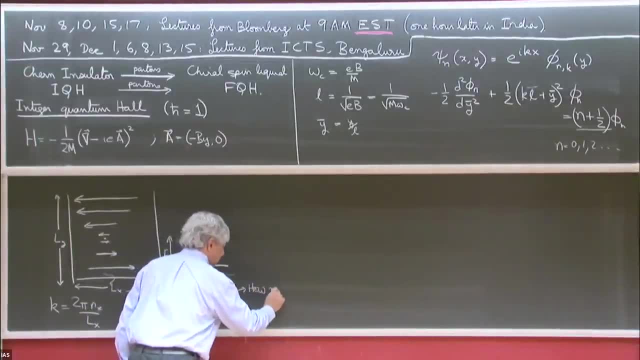 these states, all right. so this particular basis is very useful to figure out the degeneracy of states. so, first thing is: how many states do we have here? there's no more dynamic limit. well, so the number of states, it's easy to count. um, it's the number of, uh, uh, you know what. so the question now is: what is the maximum value? 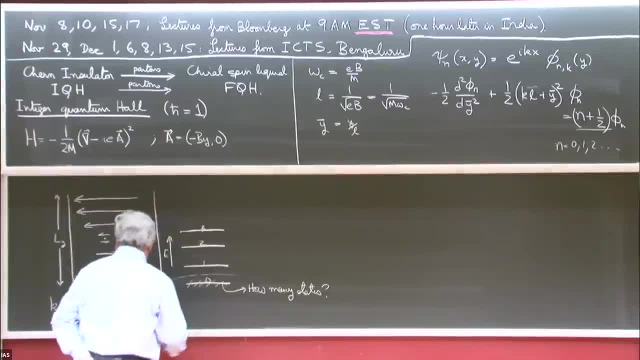 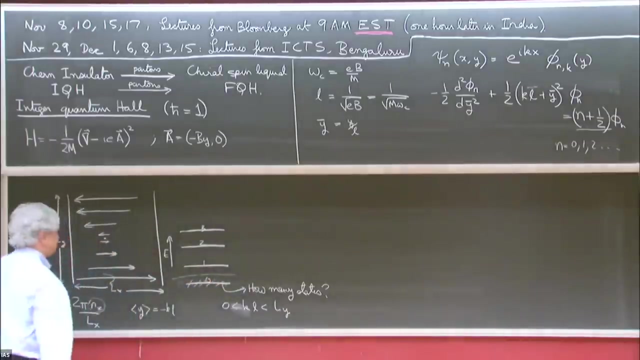 of n sub x. so how does how? what distance of n sub x uh? what are the values? a lot of values of n sub x. well, n sub x uh is given from here. so we know that k minus kl uh, or let's say is kl, is between zero and ly. so let's just call this uh. yeah, so this distance is ly. 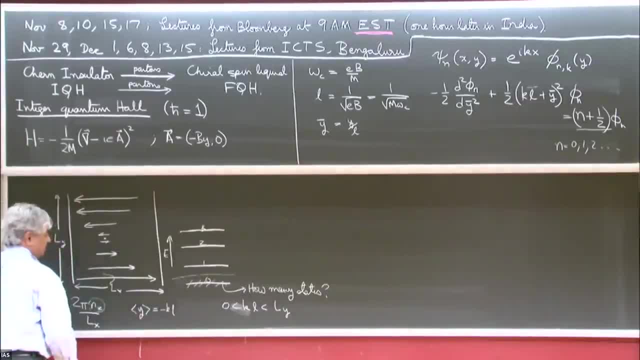 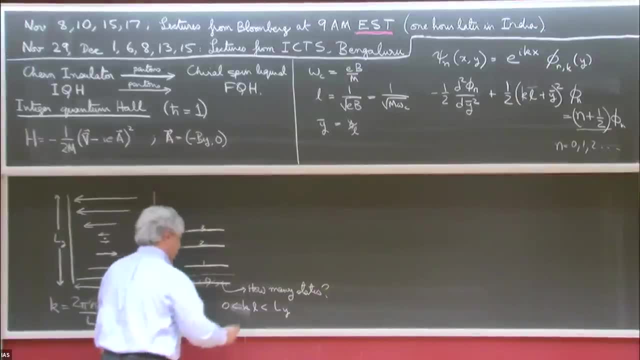 so the the range of y, which is kl uh square um. yeah, so this is y bar right, thank you, is that right? yes, thank you, um, all right. so then you get uh ignoring things in the boundary um, you will all get all of these states in this region, uh, and so this tells us that the number of states here is: 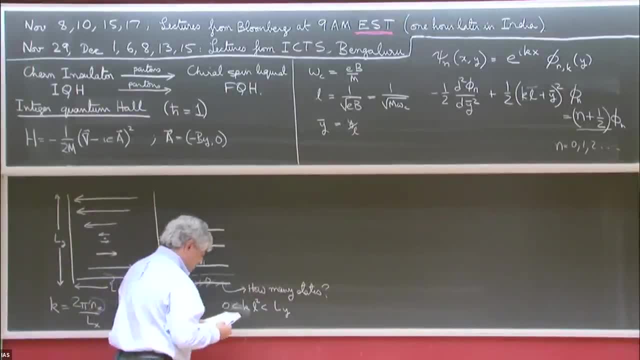 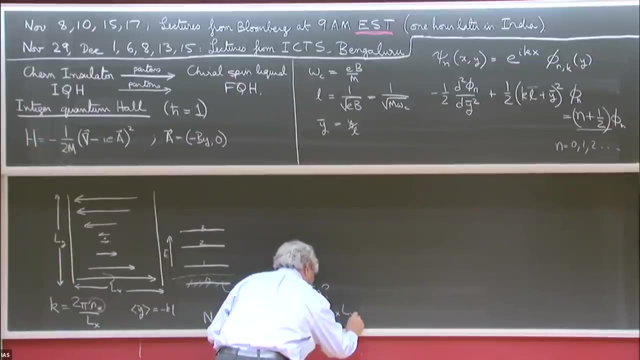 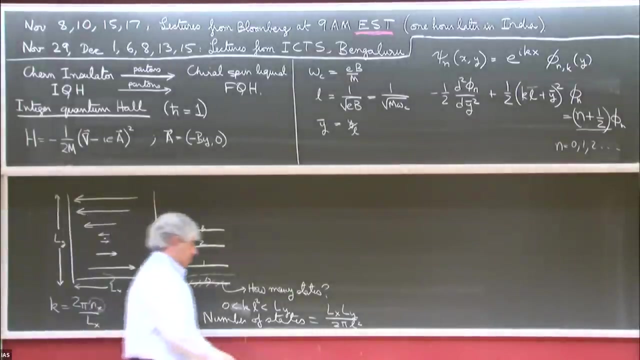 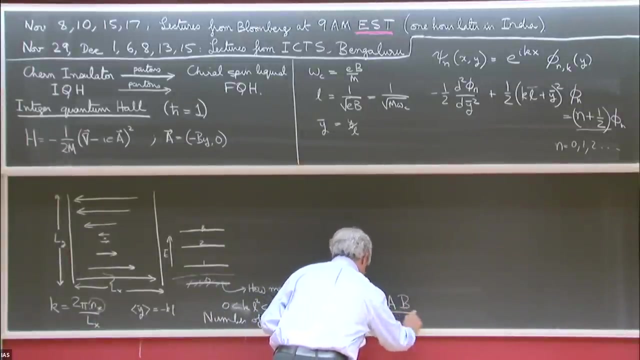 combined with this, which is actually degeneracy. so the number of states is equal to l x, l y over 2 pi l squared. and another way you can write this: in the original units is the area of the sample times b divided by phi naught, and phi naught is the flux quantum h over. 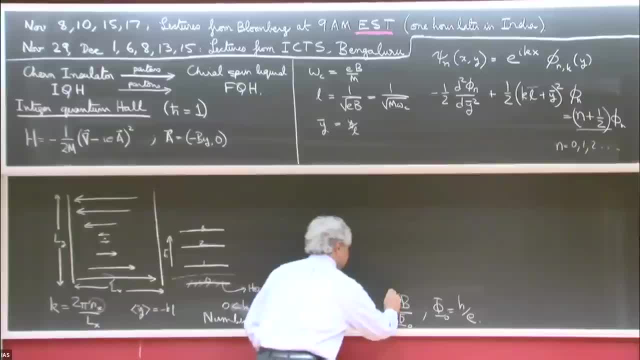 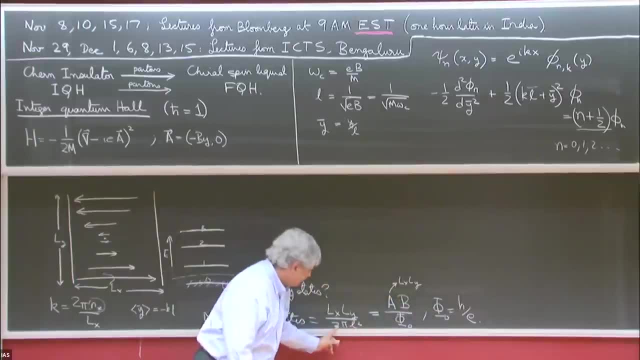 so here a is l x times l y. you'll notice that's h, not h. bar. that gets rid of the two pi over here. okay, that two pi comes from this. two pi, all right. so that's the degeneracy of the states and another very useful thing we're going to. 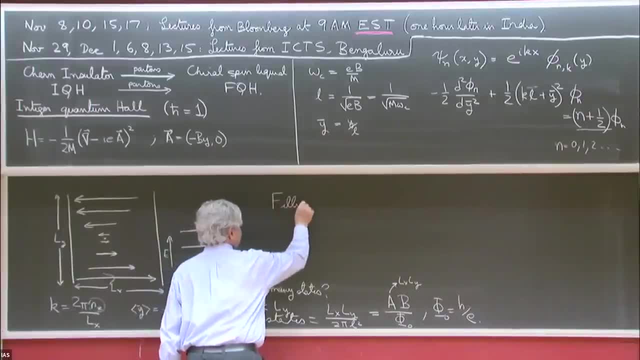 define is the filling factor, uh, which is in this case. we'll get the integer, we will consider a fractional value. you know, let me make sure i get right all the factors of two pi. this is absolutely crucial to get this right for this lecture, so i want to make sure i have it. 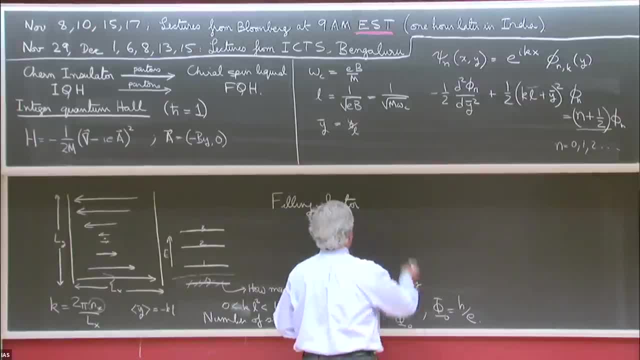 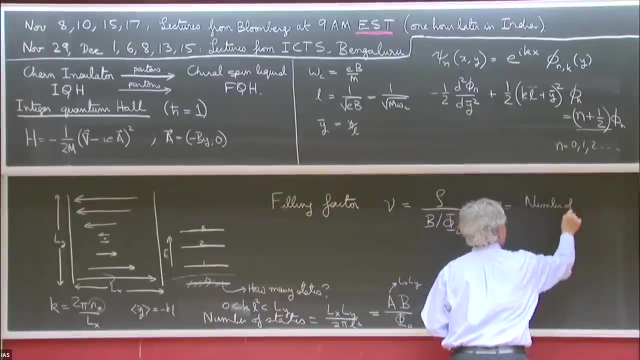 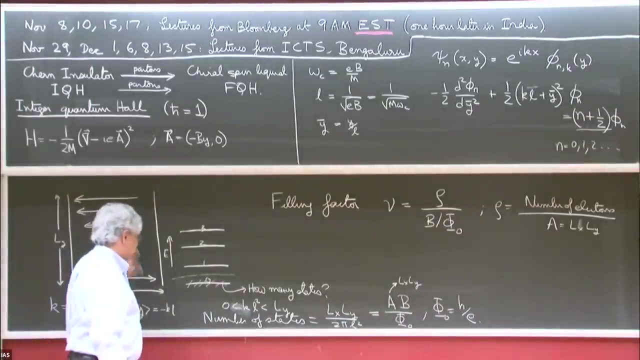 the new, the filling factor is defined as mu, which is rho over b over phi, naught over rho, with the number of electrons divided by the area, which is a, l, x, l, y. okay, so in the image of a very large sample, uh, then you don't have to worry about the edges. 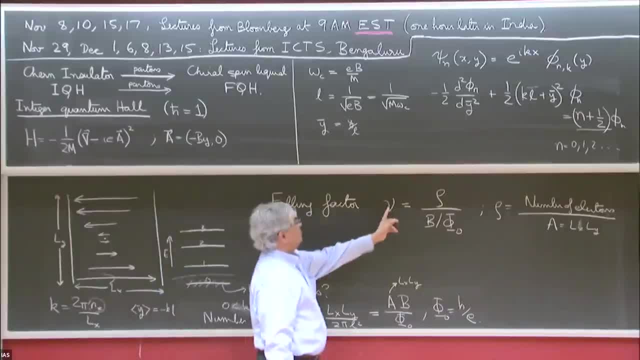 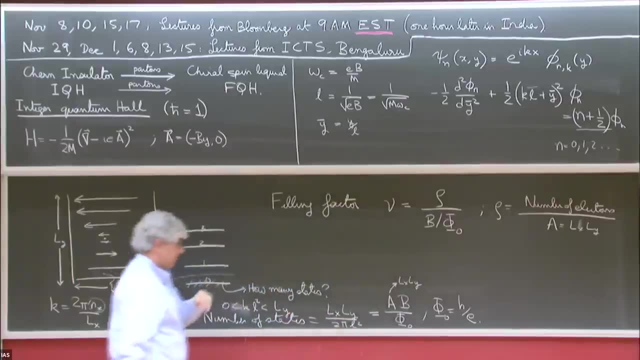 and all these results are exact. and so nu measures the density in units of the number of flux quanta. so that's one very easy way to remember it. and it's inversely proportional to p um. okay, all right, all right, so then. okay, i'm not considering the spin of electrons. 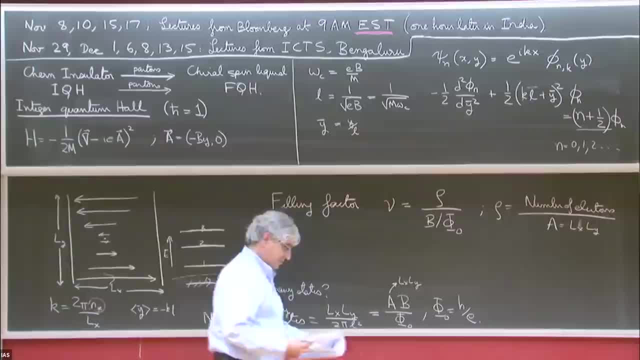 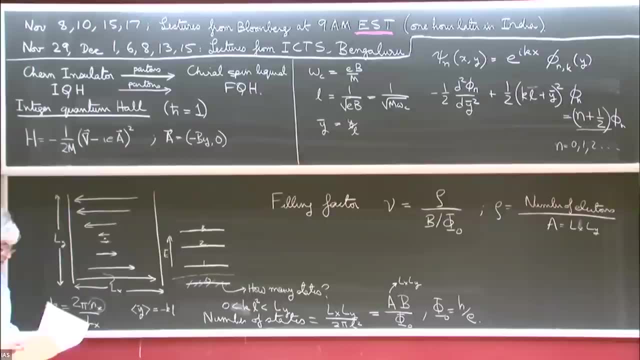 no, yes, thank you. so no spin in this entire lecture. so we assume here it's a very high magnetic field and the spin of the electron is polarized. of course it could be other interesting states where you're going to spend, okay, so we'll be interested now in the case where uh nu equals one. all right, so let me. 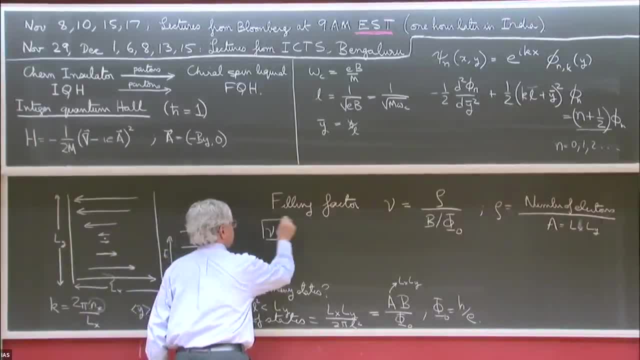 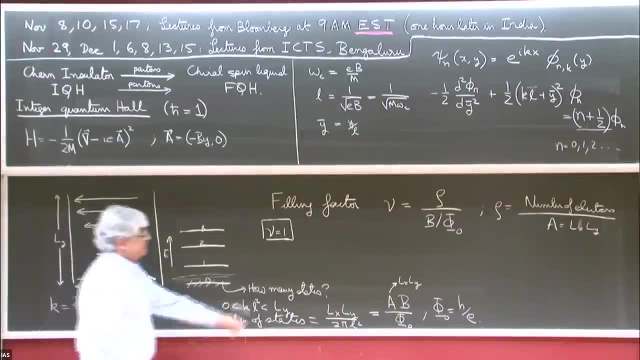 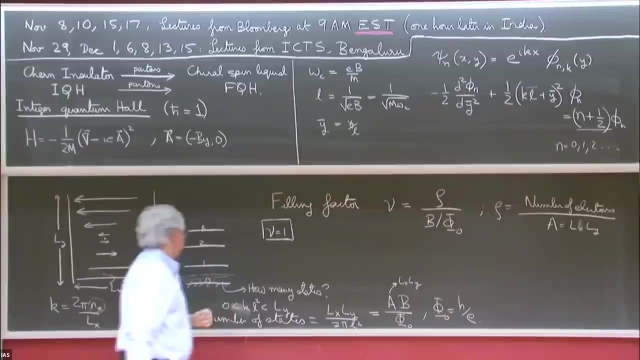 so let's consider: nu equals one, um, and now, in fact, i'll write down the wave function. and now you can write down the wave function if you wish, uh, by looking at occupying all these states at n equals uh, zero for nu equals one, and that will give you plane here times calcium and you'll get a big uh determinant. 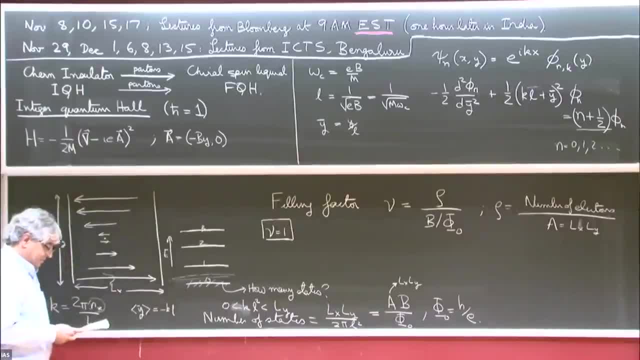 to write down the full wave function, but it's very useful for later purposes, at least briefly, so you can connect with a lot of other things. so that's it for this lecture. thank you so much for a lot of other work. uh, to write the wave function in a different gauge, so we choose a different. 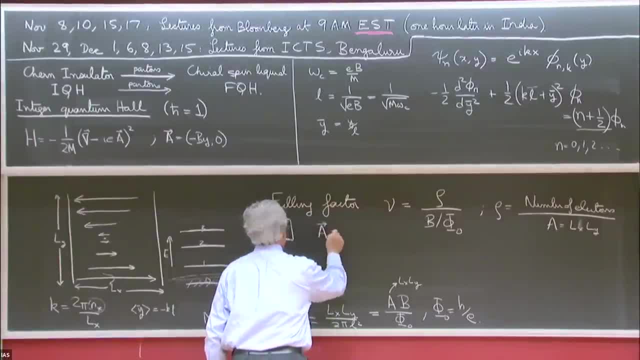 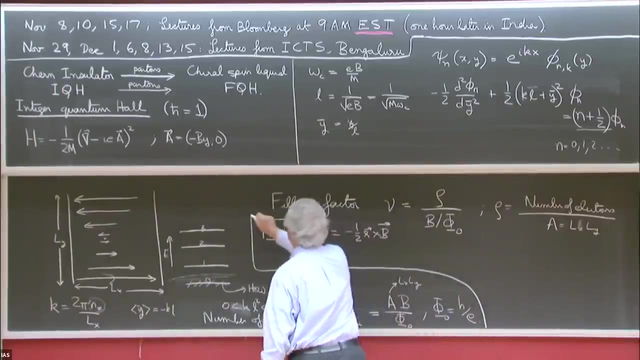 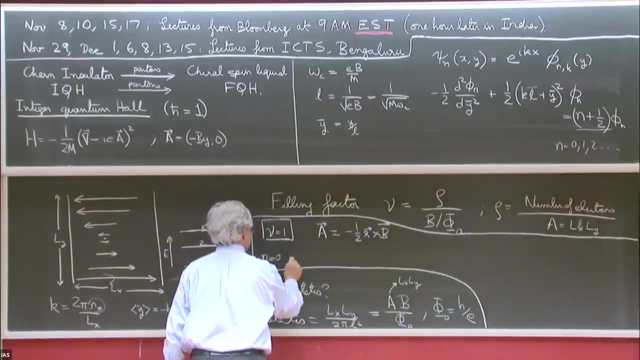 gauge where a- instead of having this value here- uh, we're going to now choose a- is minus one half r plus b. so this is going to be a different rate here. then all the lowest lambda wave functions can equal zero wave function. conditions become very simple. they become analytic functions of z. 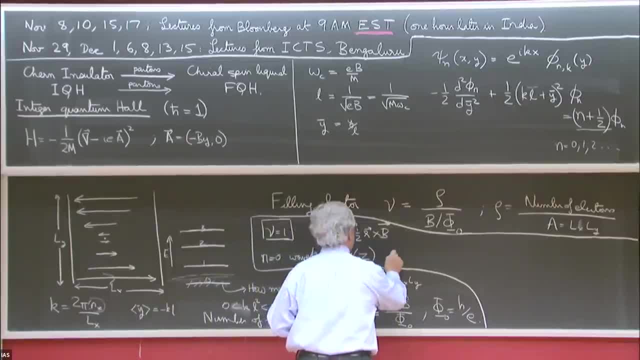 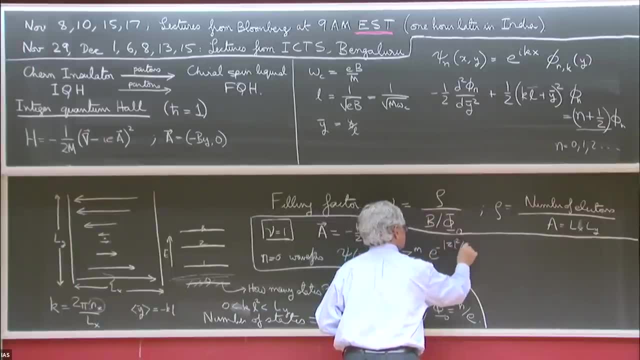 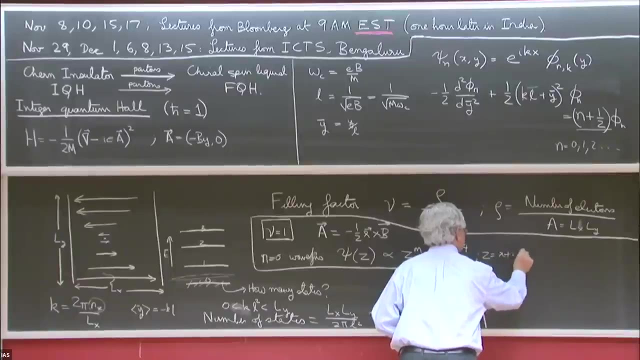 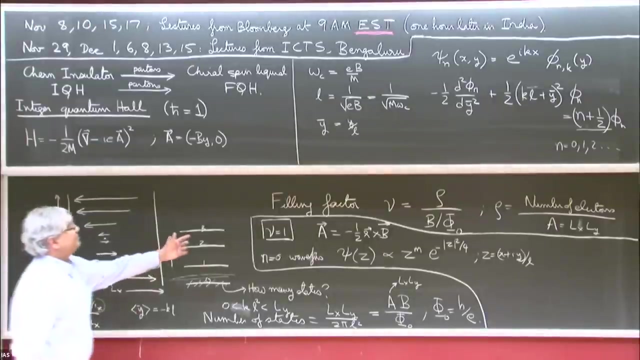 psi of z, which is, uh, proportional to z, to the m, sins, e, to the minus mod, c, squared for y, z plus i, y. so, in this particular gauge, the way to have a, whose turns out to be a, u, i, j, r, which is, you know, explicitly preserves rotational symmetry, in a sense, on angular momentum. 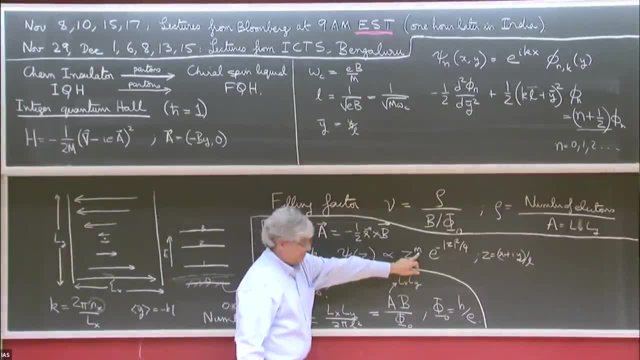 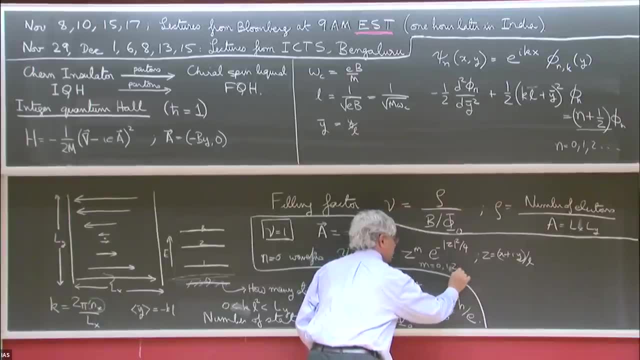 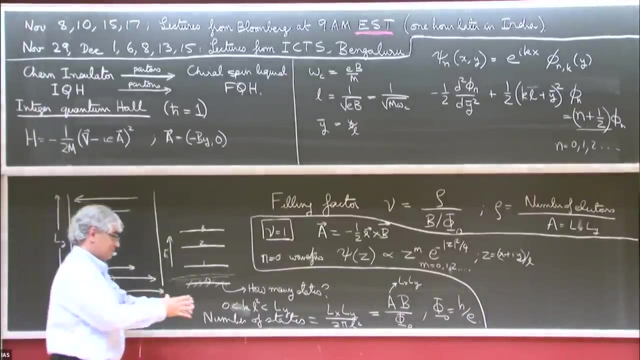 the wave function has this very simple form: And m is an integer and in fact has to be positive. so on, And so these are the so-called circular states. you know, the n equals zero is just a Gaussian. and then you take higher and higher values of n, you get states which 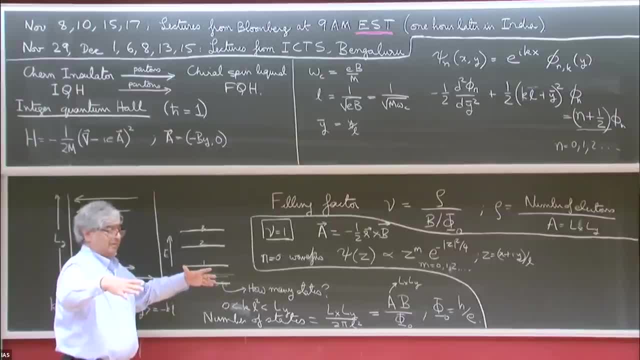 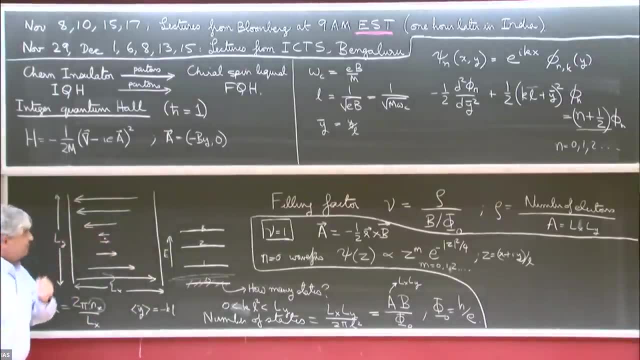 go farther and farther and farther out. So if you fill up a lot of these states, you'll get a sample which is the shape of a disk, rather than here, which is the shape of a strip. So one very interesting result here is: what is the actual wave function? So suppose 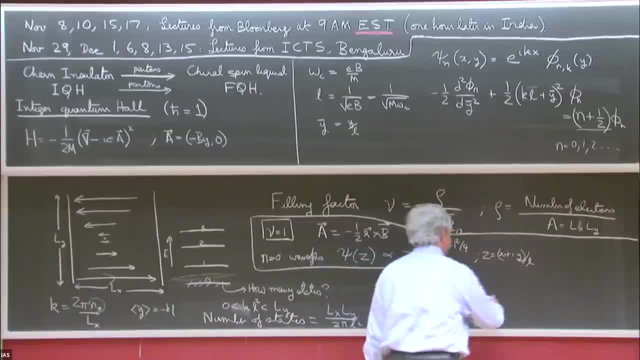 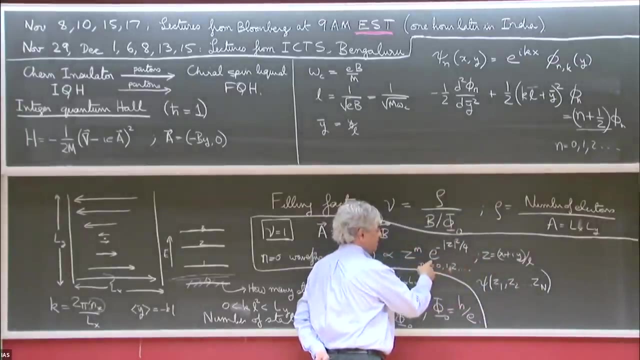 I fill up all of these states in the lowest lambda level. what is the wave function that I get? Well, the wave functions of this particular vector are this one here, this one here, and then I'll repeat what I did there. So the wave functions are this two here and this. 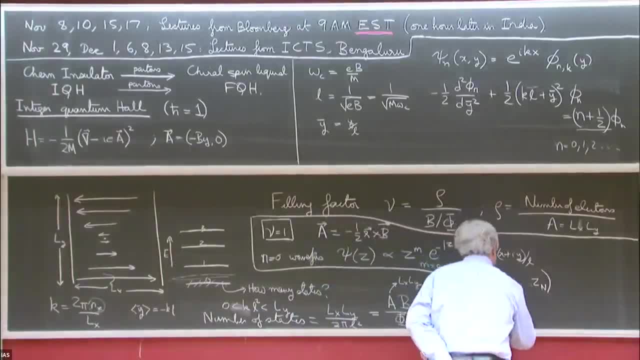 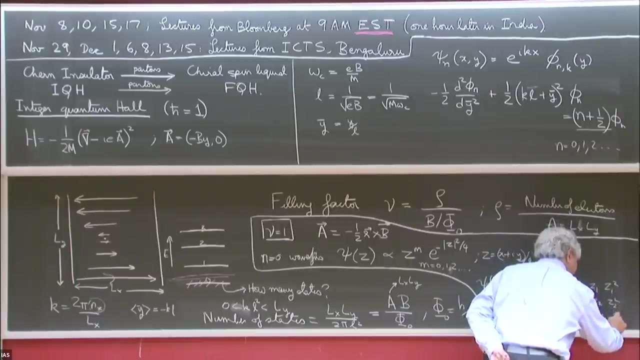 is the same one. So the wave function is is the same vector, but instead the wave function will be the same vector. So what that'll do is we'll calculate the lift factor and one, one, one, one one: z1, z2, z3, z1 squared, z2 squared, and so on, And that's the determinant. 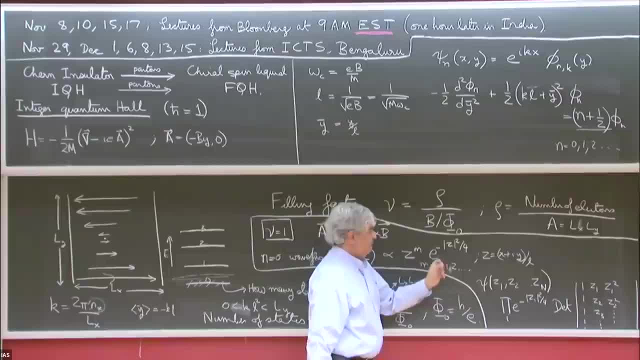 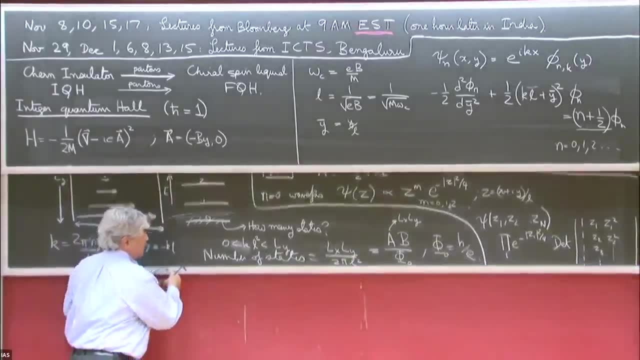 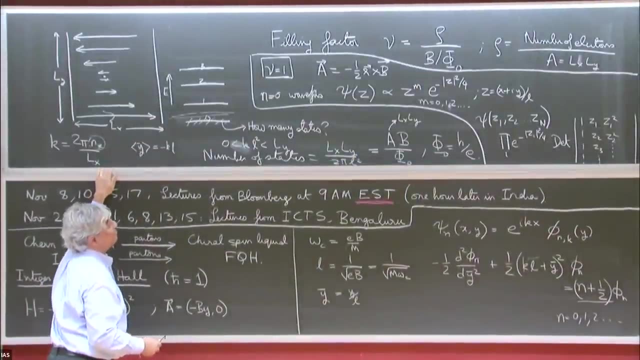 you fill in the lowest n m values of the single particle states. Okay, so that determinant is called a Van der Waal determinant. It has a very simple expression which will be, of course, much more useful in the in the fractional polynomial case. 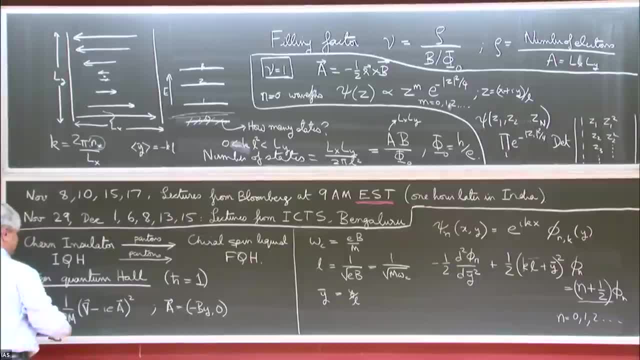 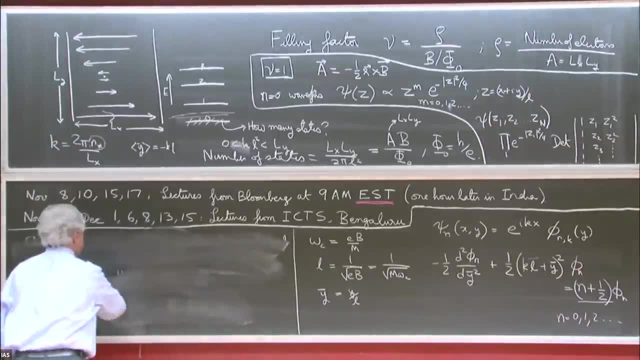 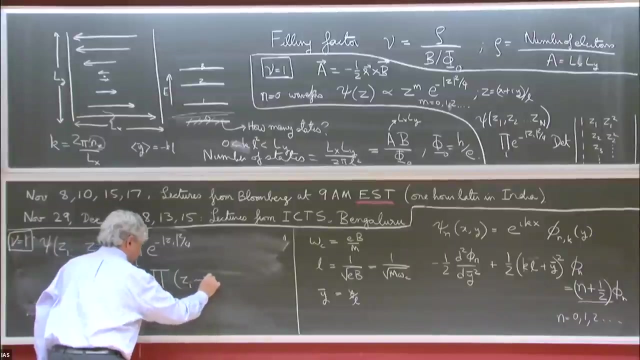 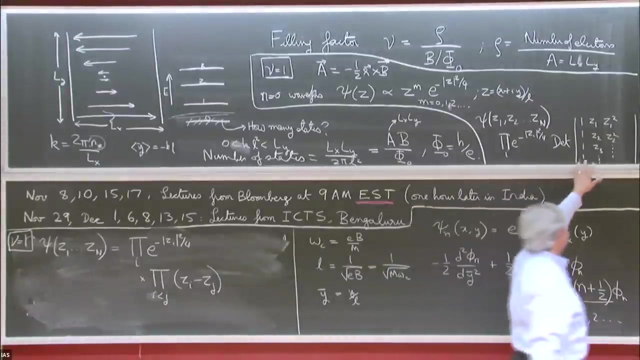 So you can just evaluate that determinant and write a much simpler expression for it. And that determinant is psi, so this is at mu equals one, the wave function, product on I. So this expression here is identical to this expression, the ko determinant. You know this. 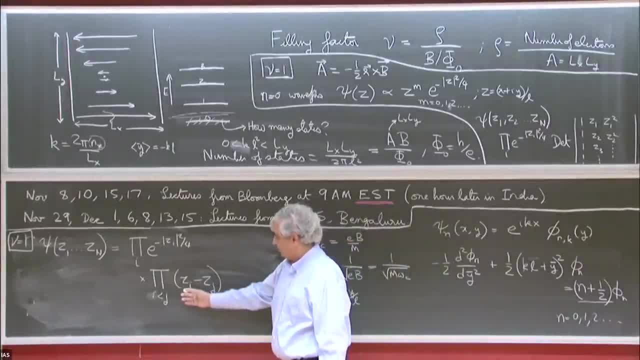 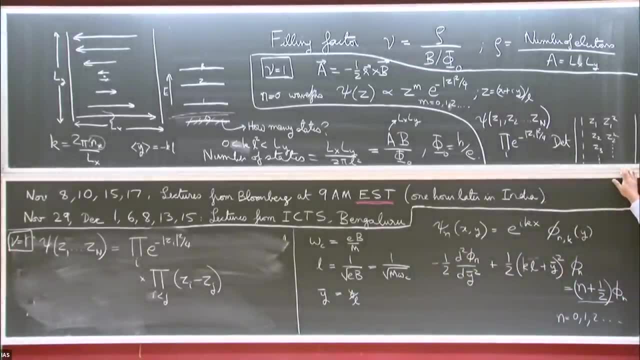 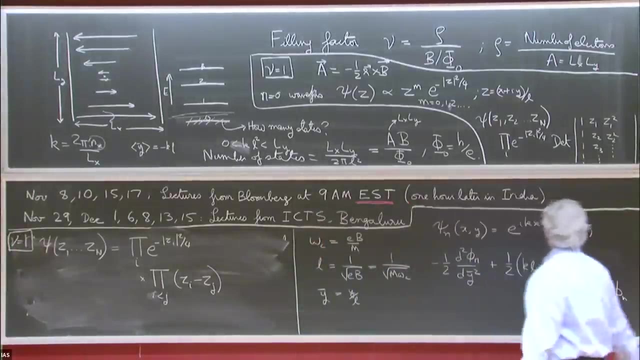 form seems to suggest that some correlations between the particles, but is part of pairs of particles. This one- makes it clear. well, any correlations there, purely due to performance statistics and nothing else. and why is the determinant equal to this? well, it follows from the fact that this is a polynomial. 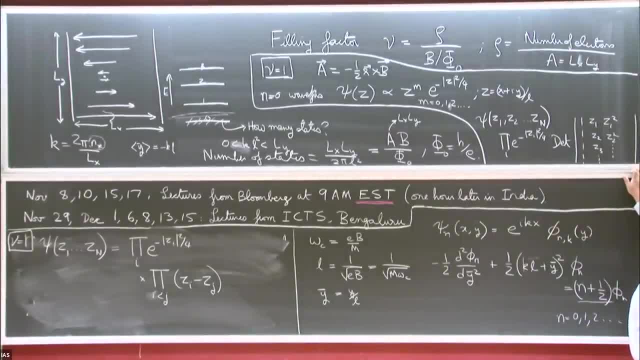 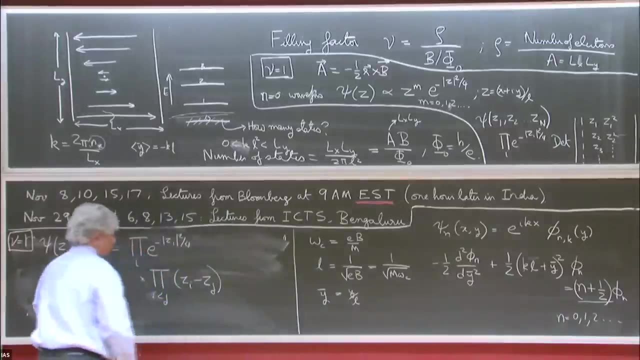 of a certain degree and this polynomial vanishes anytime any two of these z's are equal. so when z2 equals z3, then these rows become identical and the determinant vanishes. and if you just count the degree of the polynomial which vanishes at those points when any pair of points are zero, 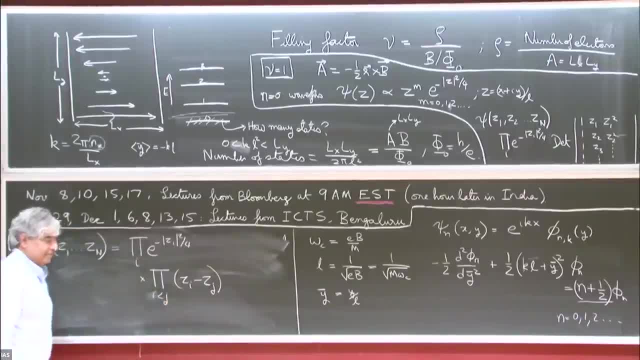 then this is the unique polynomial that has that property. all right, I'm just I'm a bit confused. so this is the weight function. for what? for n electrons, or yes, or n times? m? no, they have n electrons. it may have been too many n's here. 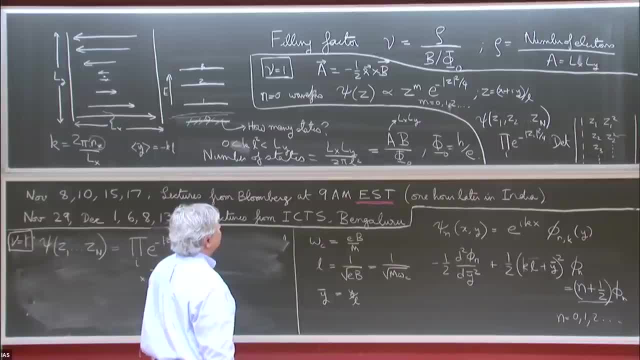 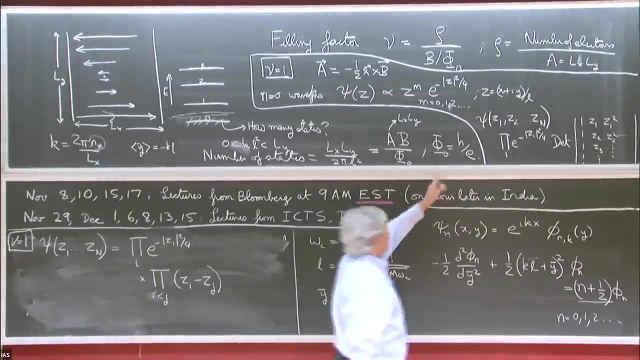 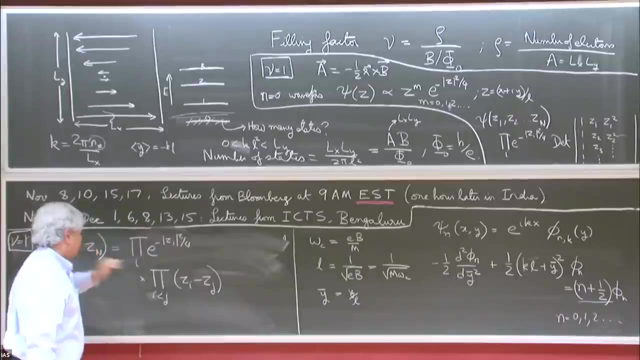 n is the total number of electrons, and electron is n equals zero and that's some value of m, that's right. so the electrons are from m equals zero all the way up to m equals n minus one. so this wave function, you know, if you actually look at the density of particles, so you look at the density average. 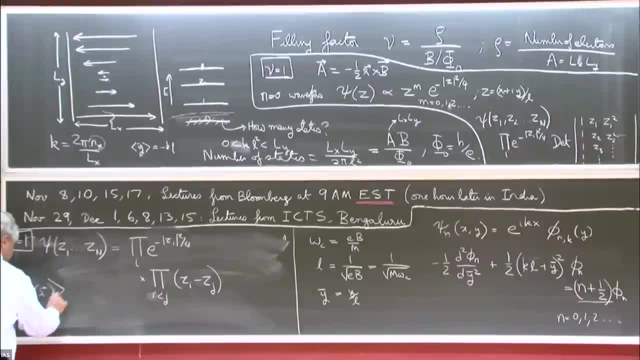 value of the density for this wave function. you can compute it on a computer if you wish. so this is that it's, of course, angularly symmetric. it has a something looks something like this: it's essentially flat here, the density here is rho, but it has an edge and at the edge it goes. 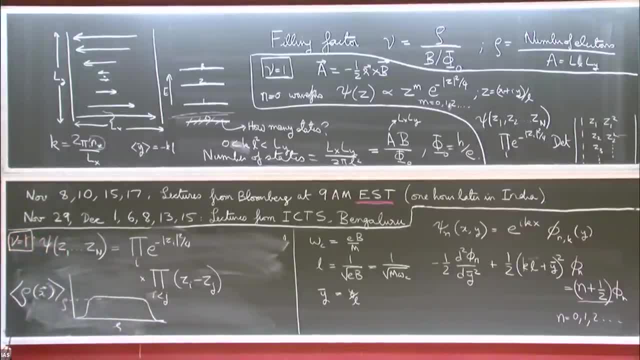 very exponentially down to zero. so that takes a little, you know, work to prove it, but it can be proven. take the modulus square, the wave function. this becomes the statistical mechanics of a Coulomb gas in in two different ways. so this is the wave function of a Coulomb gas in two different ways. 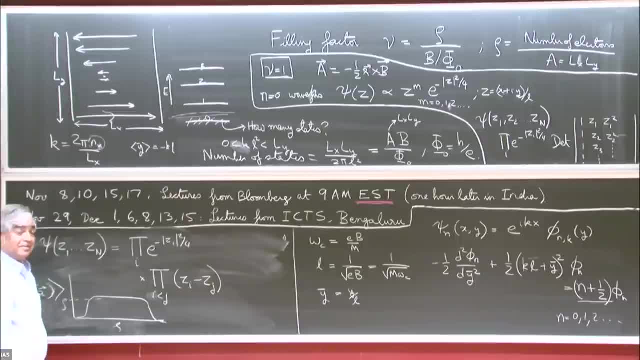 two dimensions, with log interactions, which is the Coulomb interaction two dimension, and from properties of the electrostatics of charges in two dimensions. you can prove this. this wave function, even though it doesn't look, it is actually a state of uniform density, except right near the edges. okay, so this, this distance here, well, it's whatever the distance. 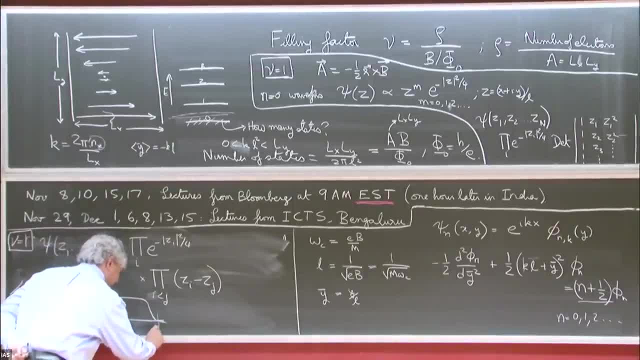 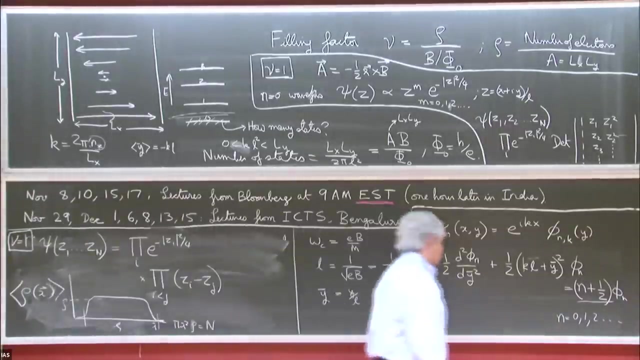 you need to. you know, call this r, then pi r squared times, n, not pi r squared times. the density times we put n over the particles, all right, and rho is inside- is the density of a filled thing. that's right, rho, is this density here, this value? 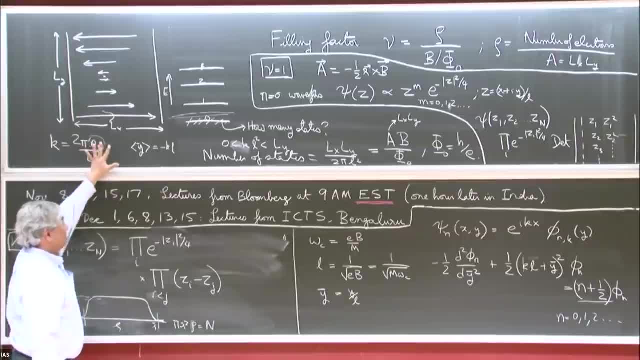 of course, here the density will look rather different. it'll be the same in the center, but on the edges it will fall off and we'll have the rectangular shape. if you took those dates here you, you get a circular shape. okay, all right. so what I want to consider next, then, is I'm going to go back to this rectangular. 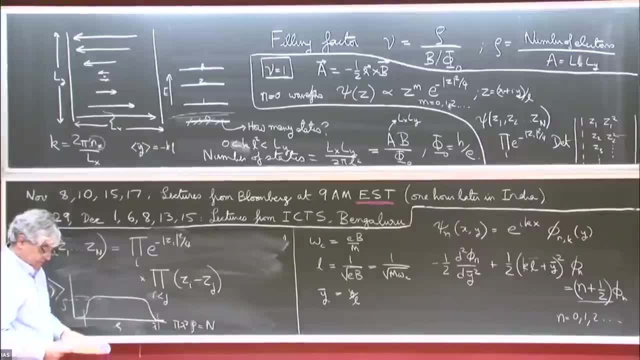 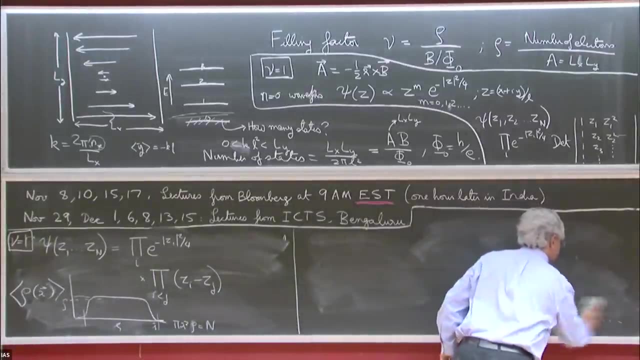 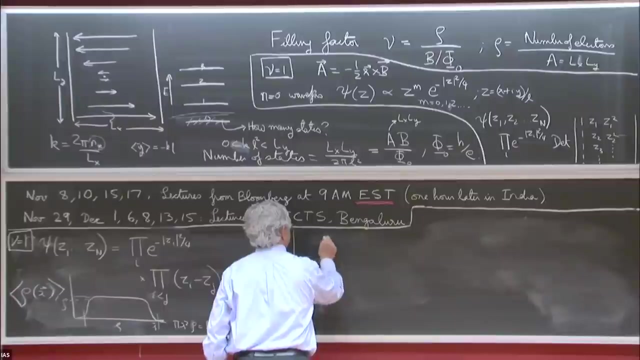 shape and look at the edge states, we go through the computation of by, however. okay. so now, if you want to bring the change, you know x is the velocity of the��. So now we are back to the other gauge. So we're back to the gauge. A equals minus EY and zero. 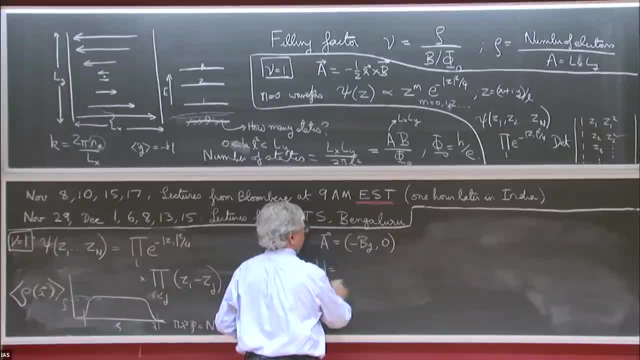 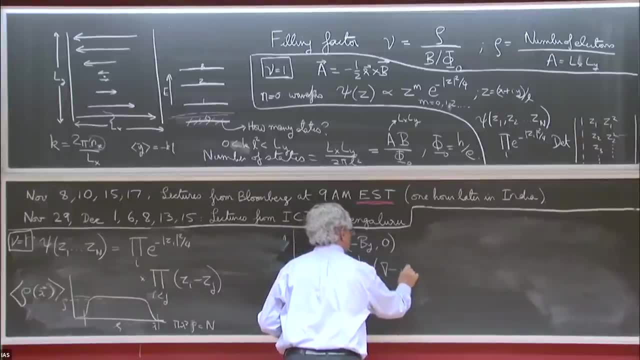 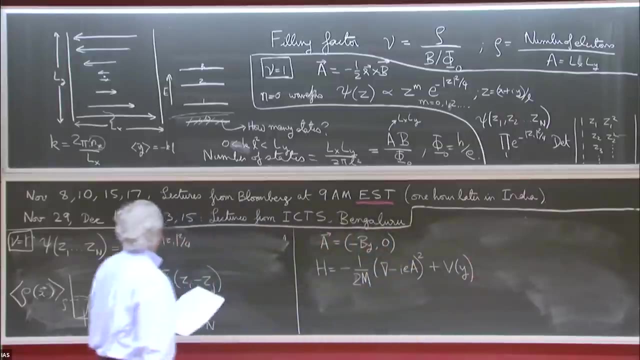 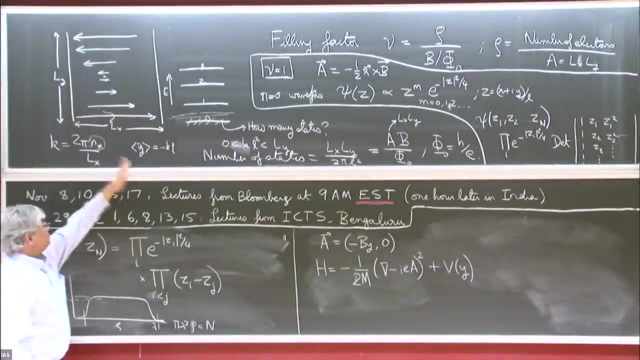 And I'm going to consider the Hamiltonian H is equal to minus one over two M. Okay, so now you'll see why I choose that particular gauge: because I had a potential in this direction. So there are walls or something towards the ends. 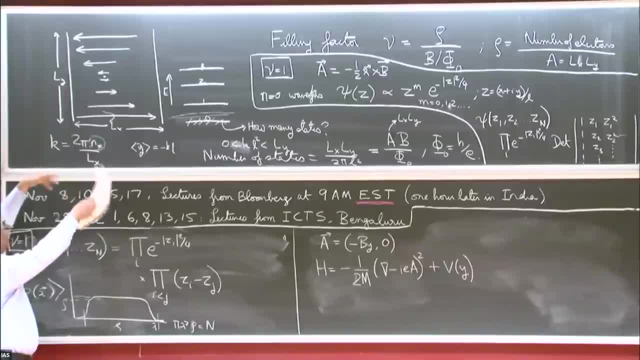 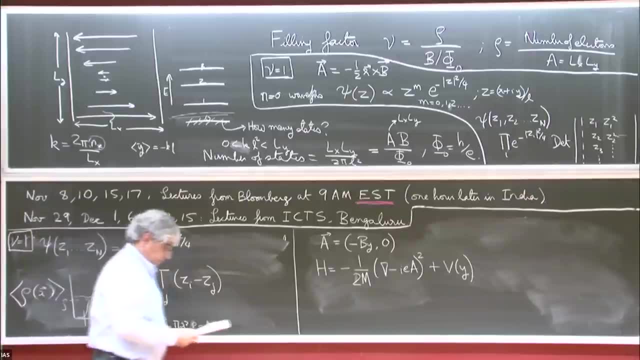 So it's a very slowly varying potential at the bottom of the sample but towards the edge you have a boundary, but I still have a conservation of momentum in the X direction. So if I write down the Schrodinger equation now minus one over two M. 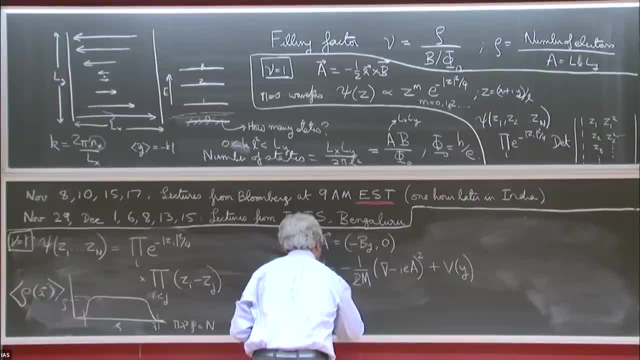 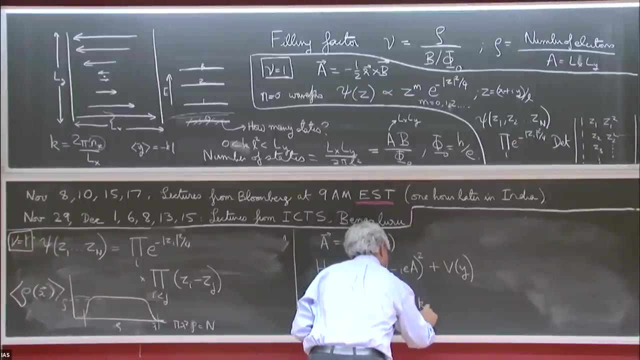 and now I'm dropping the bars here- L is equal to one state M plus one over two M of K, plus K in the X direction, plus BY squared, as we had before. But we don't want to just add on the potential V of Y. 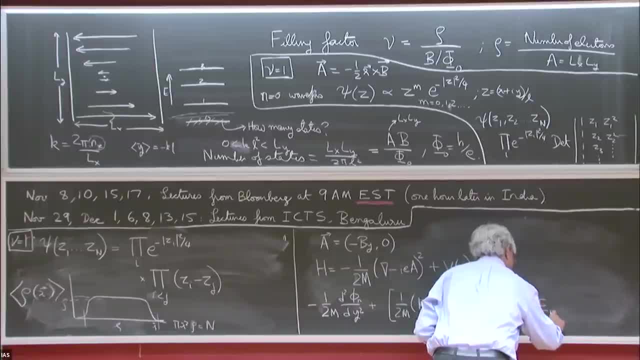 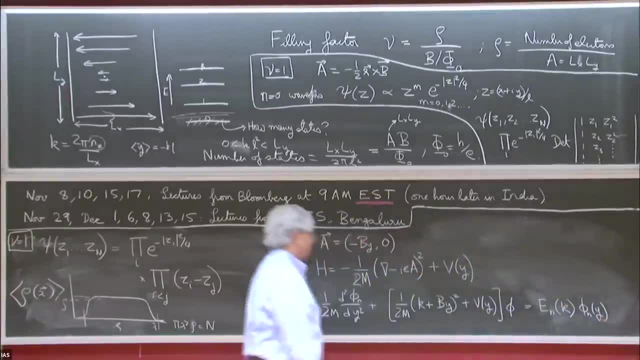 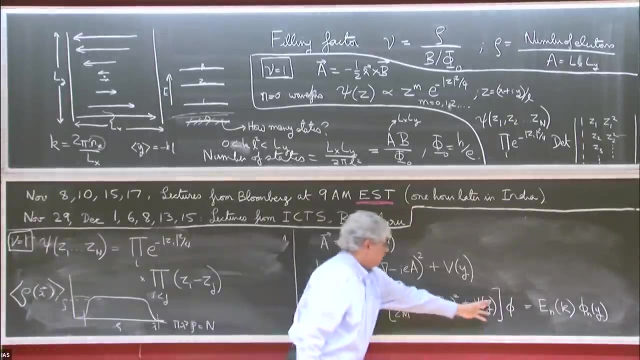 Y would be some eigen energy, which will now depend on K times five N of Y. Okay, so this is still a one dimensional Schrodinger equation and you could have taken: V of Y equals just a quadratic function of Y, and it's still solvable. 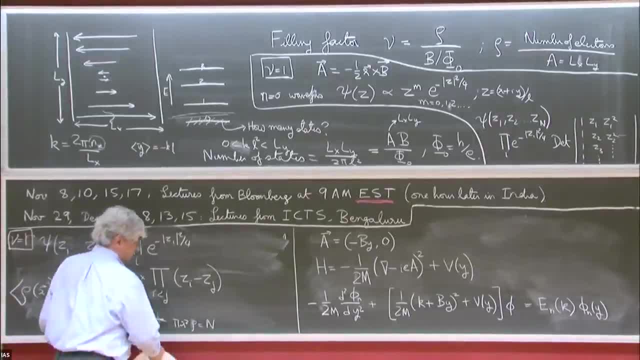 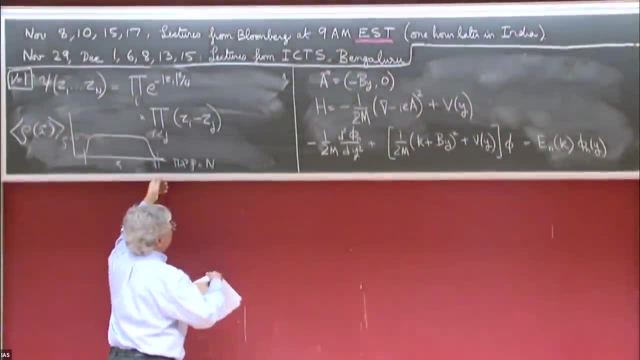 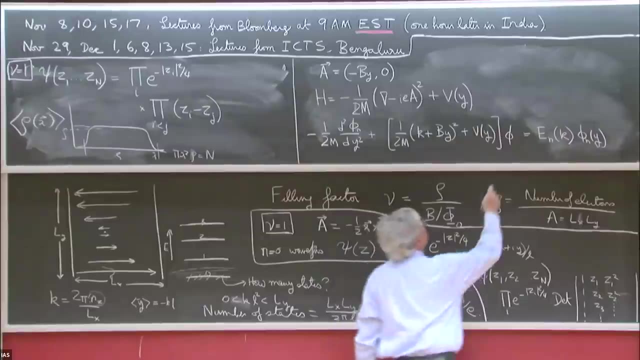 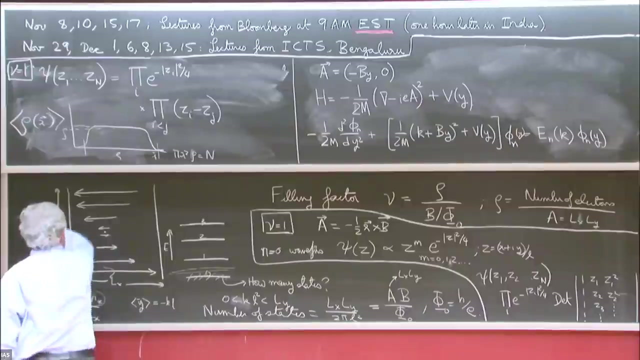 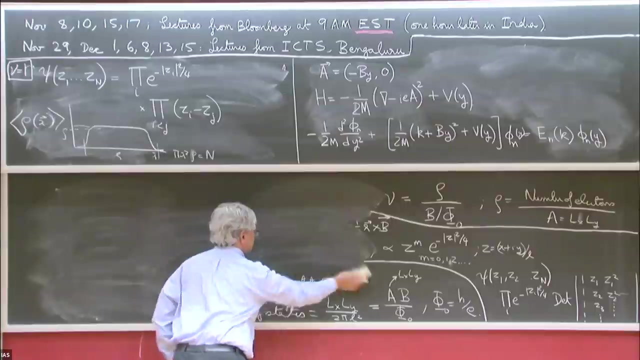 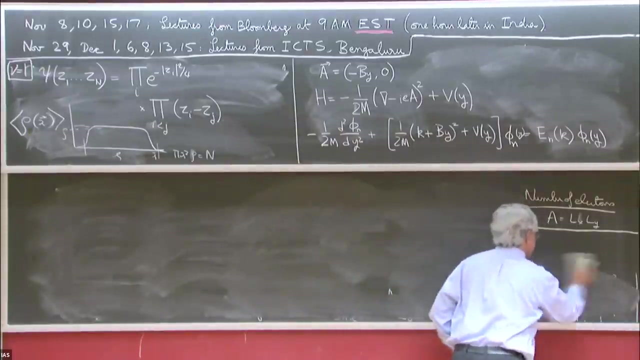 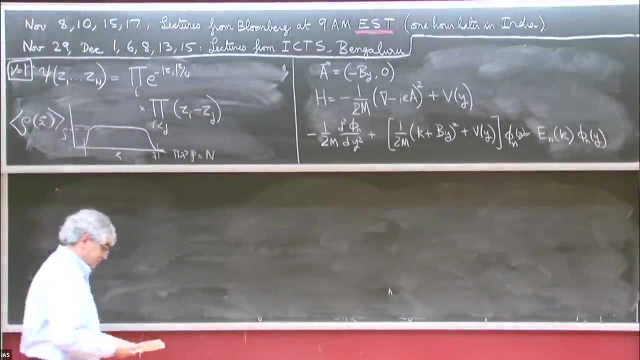 You can do that, but let's just look at some general features. So what this E N of K looks like, It's basically a pony, this superannually- and remember, this is a logarithm. So what this is, this is a. 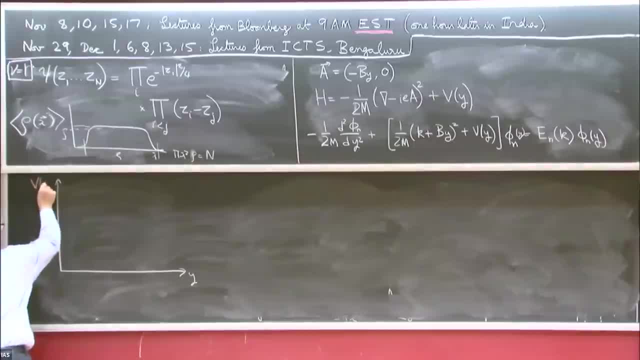 so I'm just gonna look at the right edge of the large Y, the top edge of the sample, That's the big Y. in a lot of cases That's the FOF example. No, my y was this direction. I forget, Yeah. so this is the right edge. Anyway it'll. 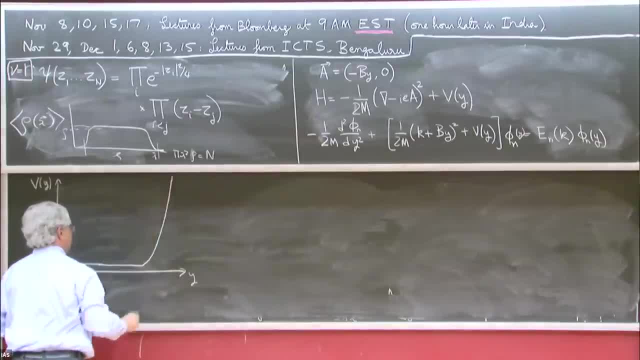 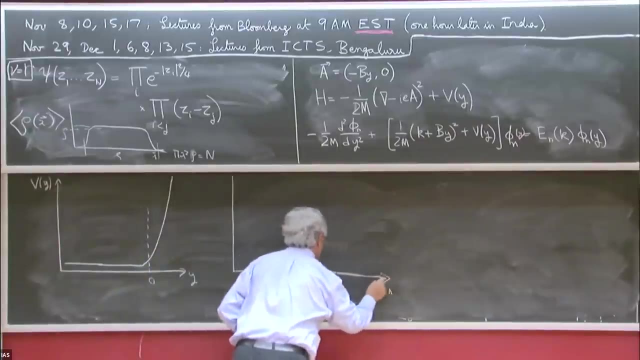 be flat. And then let's imagine it goes off to infinity And somewhere here I'll choose my coordinate, y, to be over here. That's what v of y looks like, Okay, Well, here I'm going to plot the eigenenergy of k, and this is momentum k. So what's going to happen? Well, 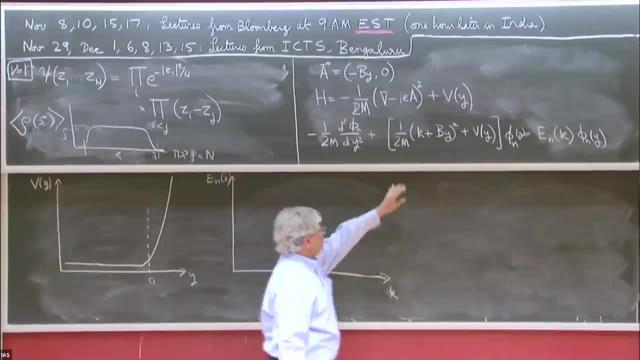 when k is very large in this direction, we see from here that y on the average is large and negative. So when you're out here at very large k, the wave functions are sitting over here. So v of y is just a constant. You can make it zero, So v of y plays no role in this region. 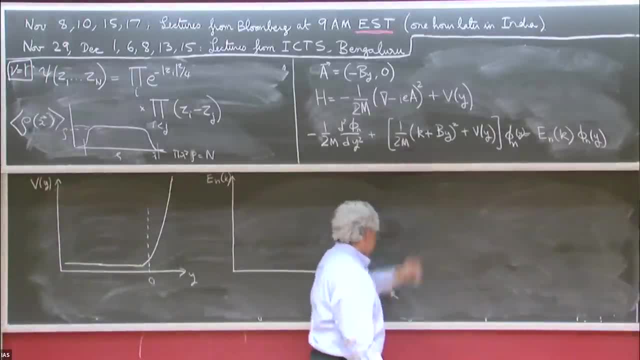 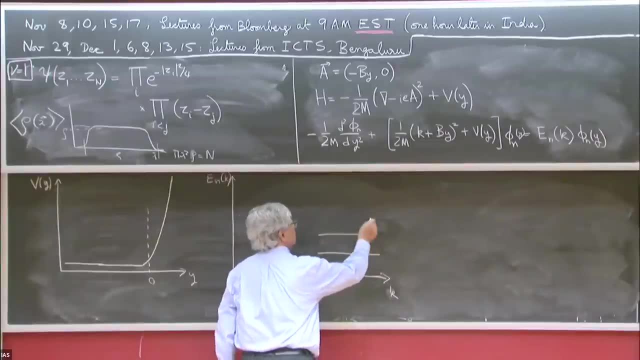 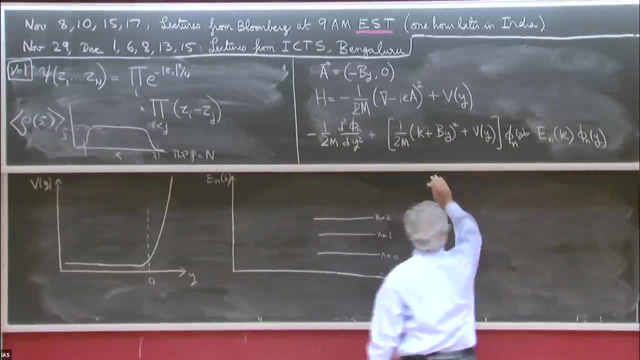 Why can we look at y's that are large k, So we have to scattered theormath, reg udants, half of themaz石. So we're looking here. so I've ever- okay, let's go back here. So I've ever- okay, let's go back here. 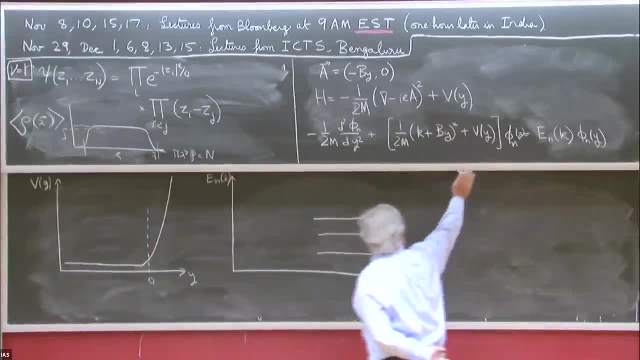 Okay, let's go back here. For y large and negative z of y equal z. So for y large and negative z of y equal z. Okay, so now you're going to have to solve this harmonic oscillator equation and the 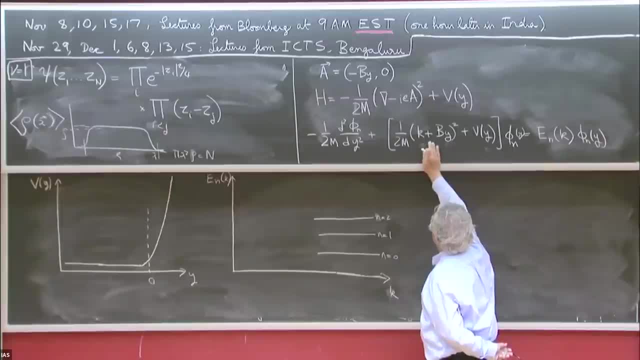 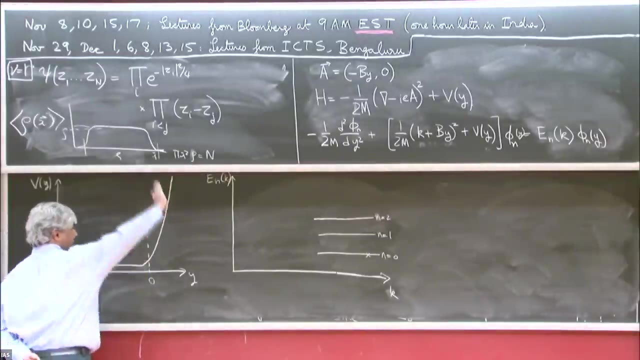 wave function of the harmonic oscillator are centered where this is zero, And that's centered at k equals minus py, which is, since y is large and negative, k is greater than k K, then your wave function is some sort of Gaussian here and it doesn't care about the 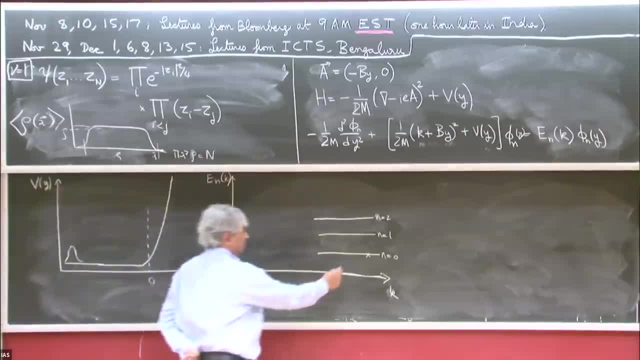 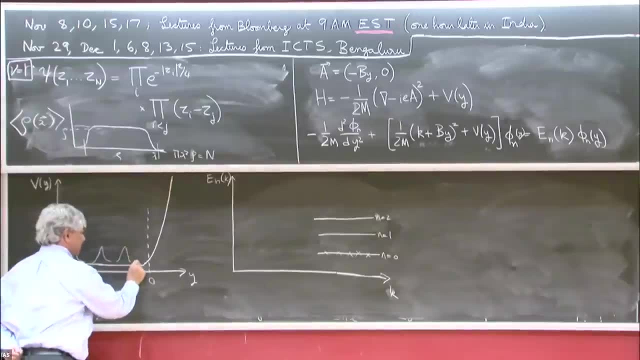 fact that it's going to go up. So as you decrease your values of K and you come down to smaller K, this Gaussian is going to come here, here, here and now you can see it's going to go up and the energy is going to become K-dependent. So as you decrease your K, you approach the. 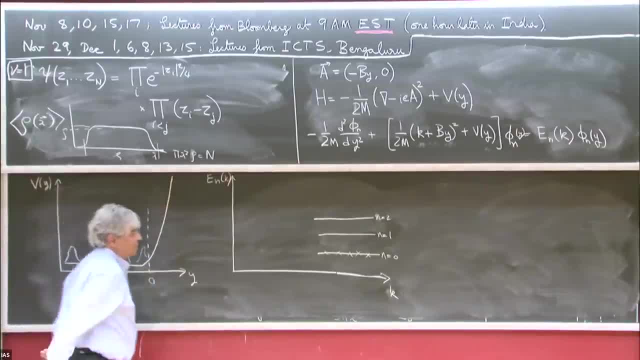 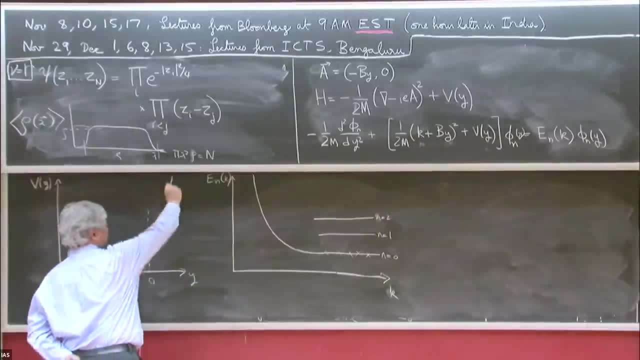 edge of the sample and your energy goes up. So that's really all there is to it. So all of these things will go up in a way that roughly mirrors the increase to be applied. So this is roughly what it looked like. Of course, you can do a better job of solving it and 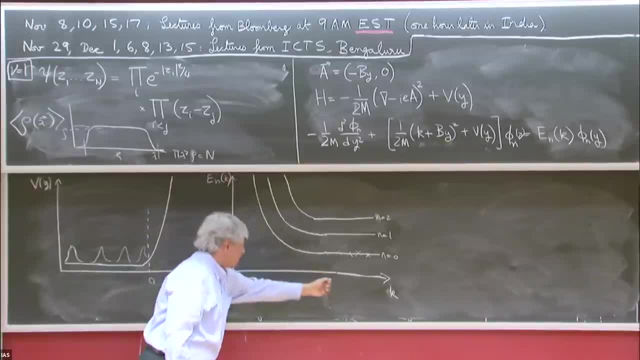 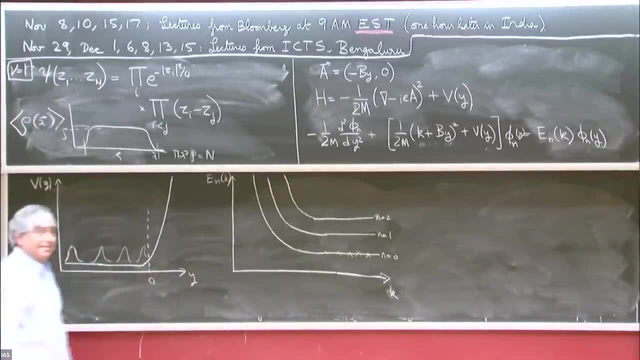 you'll get these states here that move on up as K becomes smaller and smaller, because you're hitting the edge of the sample in the y direction. Okay, so clear, All right. so now still dealing with free electrons. we started in a state. 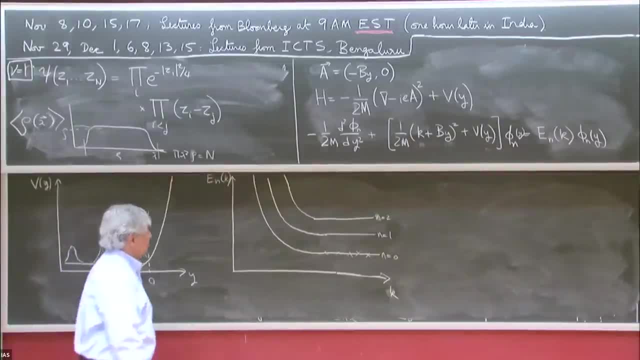 where we fill the lowest time now level in the infinite sample. but we have some chemical potential here. This is our chemical potential, mu, and we're filling all states below that chemical potential. So what we see now? so these states are all occupied. These are the 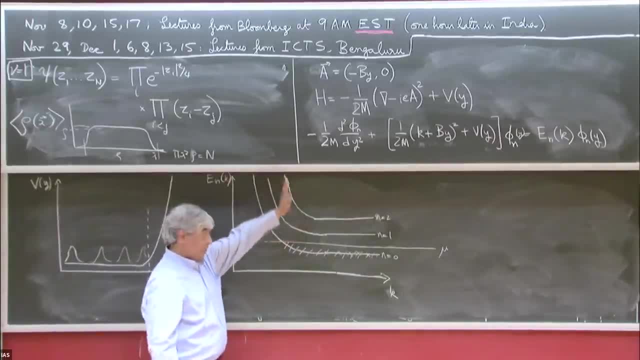 low energy state. All these high energy states are occupied. All these high energy states are occupied. All these higher end states are not occupied. But now we see something very interesting. In the bulk of the sample for large K, which is the same as sitting over here, there's 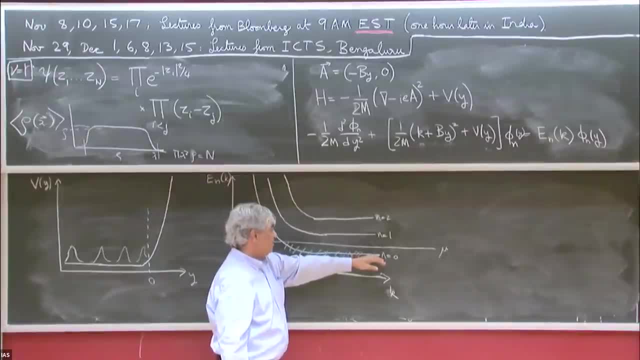 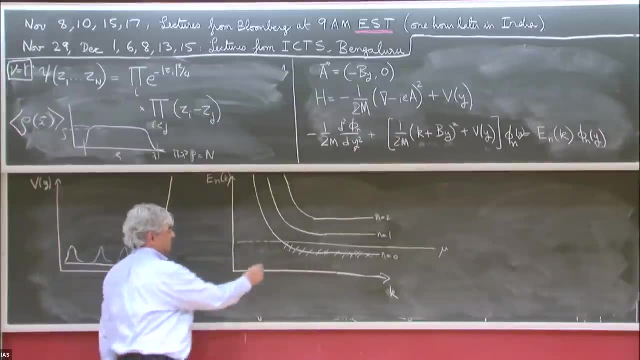 a gap. To add any extra electrons, I have to go all the way up to the next line of them, But as I approach the edge, well, I have a Fermi point and I have a zero energy excitation And in fact, this is exactly the pyro Fermi gas that we saw last time, which is an insulator. 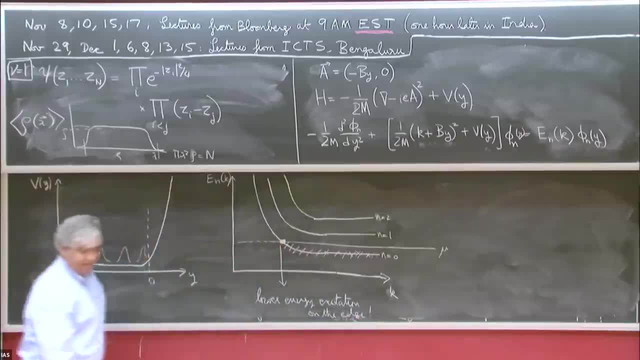 where we had. you know, like I showed you the picture of the bands which is now on the website. actually, where the bands appeared, the one dimensional band appeared within the band gap And then we have a K, which is the same as sitting over here, and we have a zero energy. 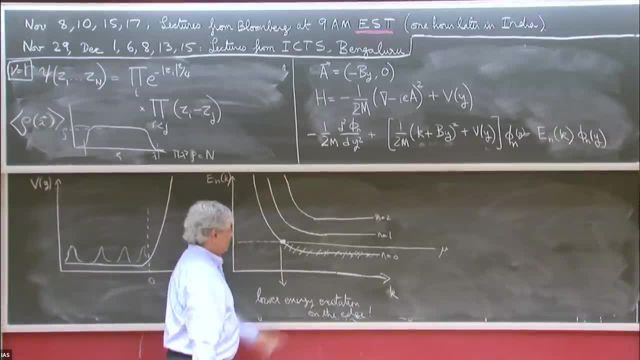 state. So we have a K band gap. Here you can explicitly see the one dimensional bands. Here's one of them, And the other one is at the other end of the sample where you have the other edge. but I'm only showing one edge. 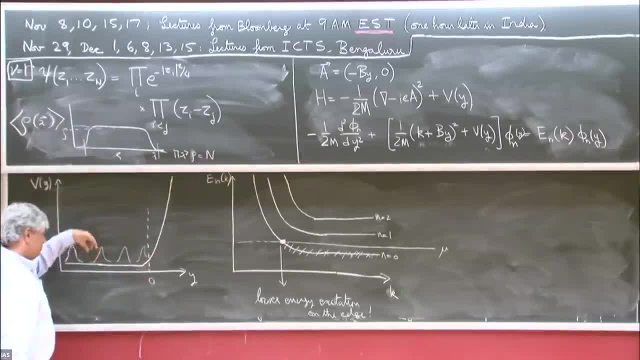 I don't have to worry about the other edge, because the wave functions are bouncing, localized on the magnetic field scale. So what is this state over here? Well, it disperses as a function of K, So that means it's moving. it's you know, it's got a velocity and it's moving in the X direction. 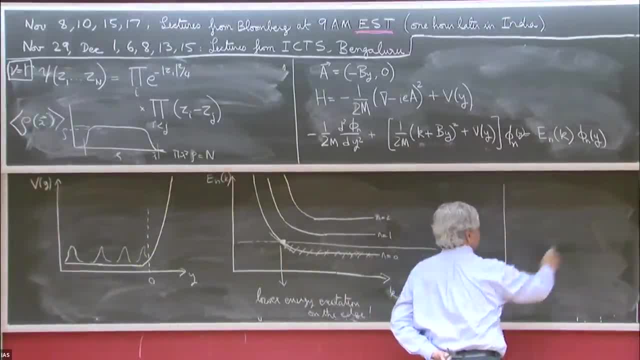 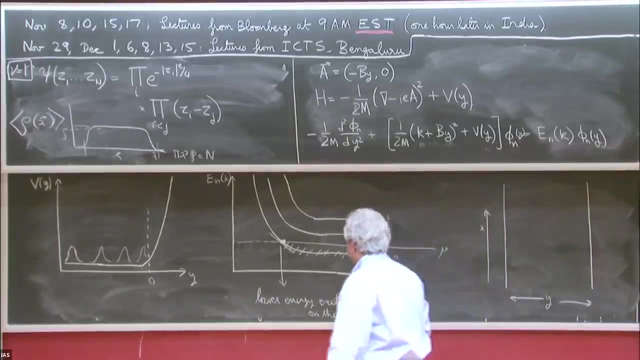 OK, so if I draw my sample again, So I think this was Y. Yeah, this was the Y direction, this was the X direction. So I have a state on what I hear. Let's see if I get the sign right now. 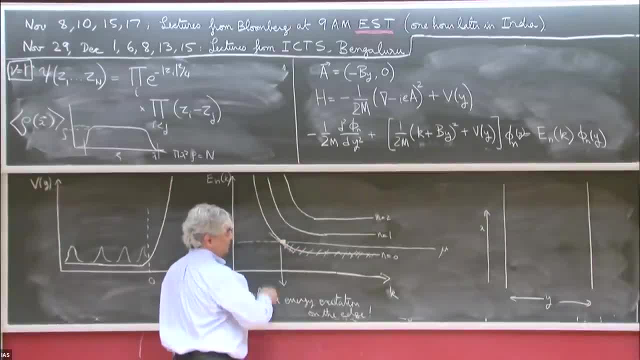 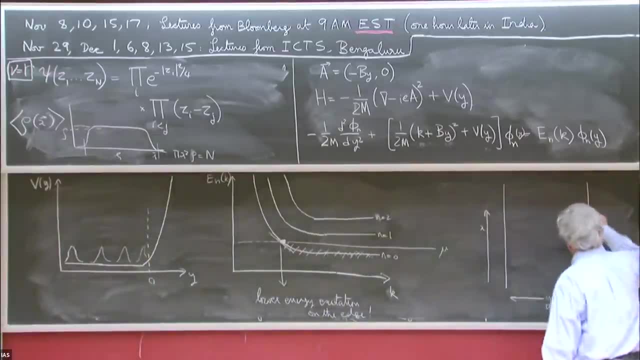 So this thing has a velocity that's negative as K increases. So- and this is on the right edge, So that means the thing is flowing this way. I have a state over here going this way, and on the other edge I'll have a state going the other way. 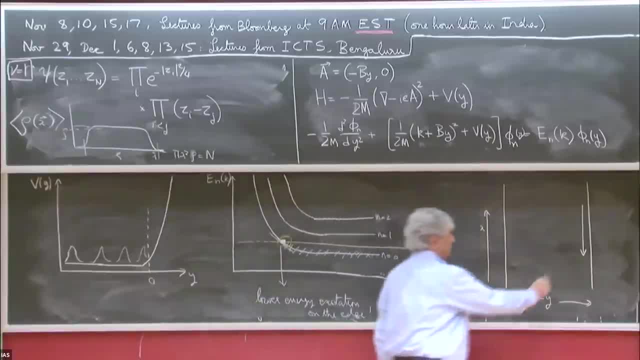 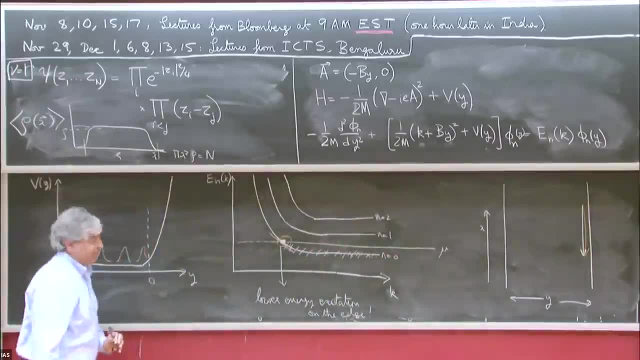 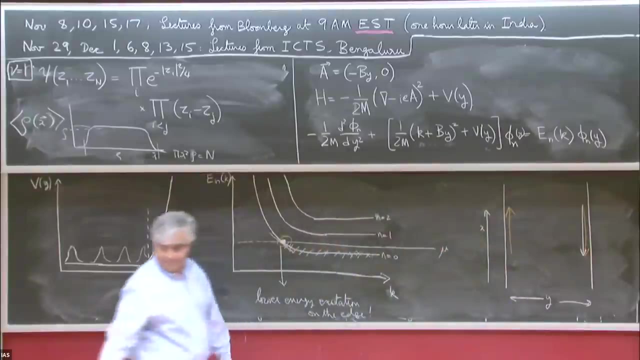 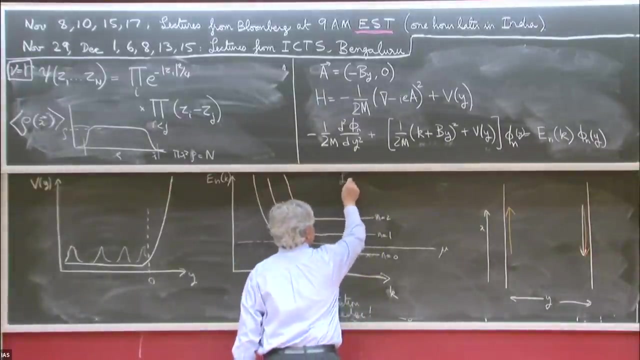 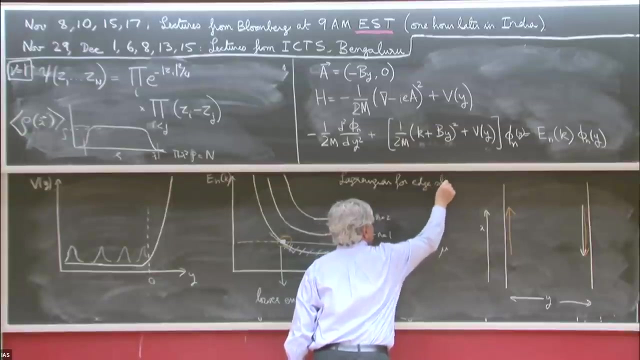 So this state over here is a bunch of wave functions that are moving in the negative X direction. on the positive Y end of the sample And similarly on the other edge, there'll be a bunch of states moving in this direction. So I can now very easily write down a theory for these edge states. so Lagrangian for edge states. 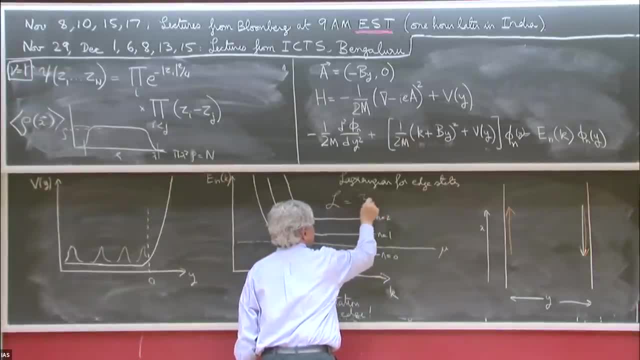 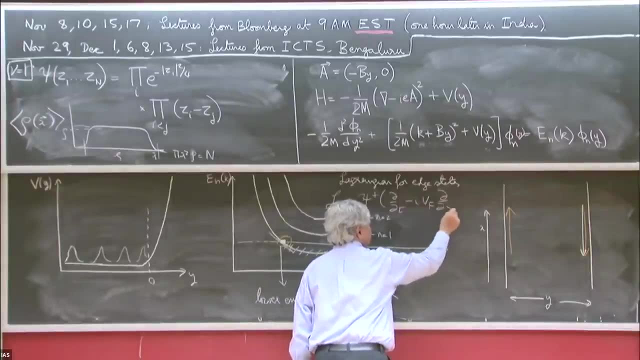 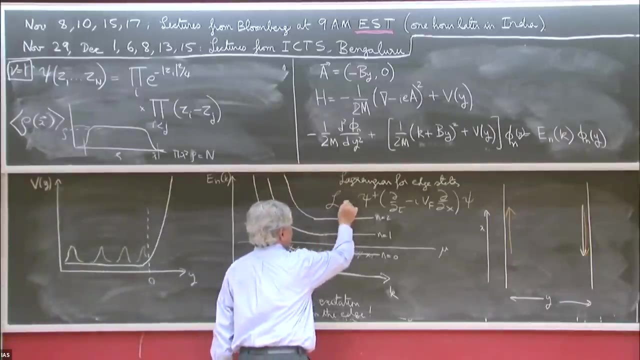 Well, it's exactly what we had last time inside the Eiger: back to tau minus IVF. So it's a 1D gas that only disperses in the KX direction. There's no dispersion in the Y direction. 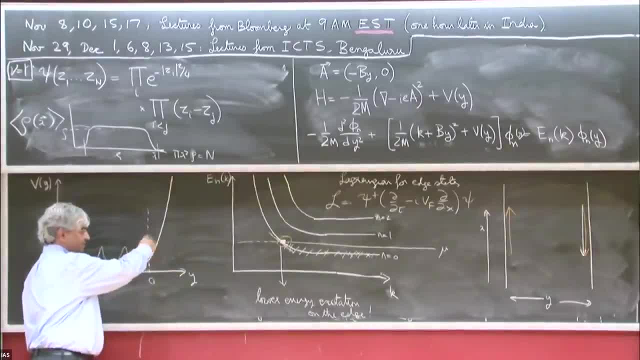 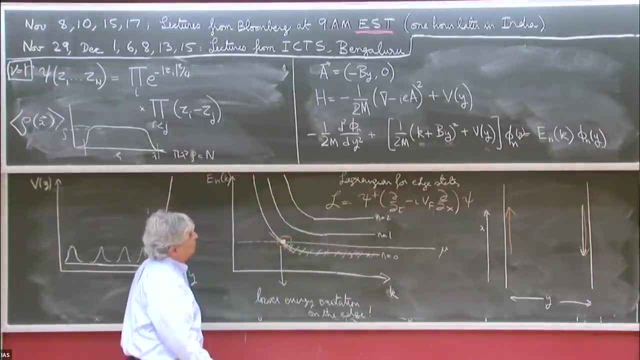 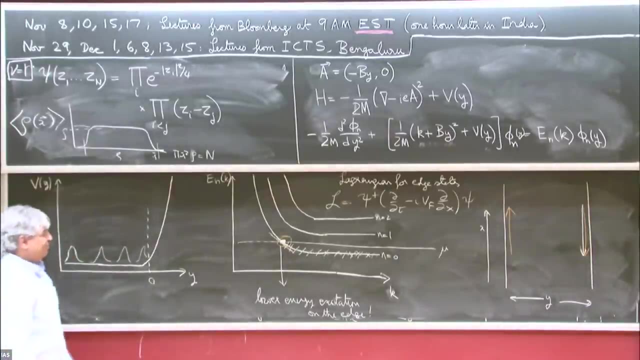 And it's you know, states that are sitting at the edge of the cell And they're exponentially localized in the transverse direction. OK, All right. So this is all very explicit, And you know. you can see them up here without even knowing anything about terms, numbers. 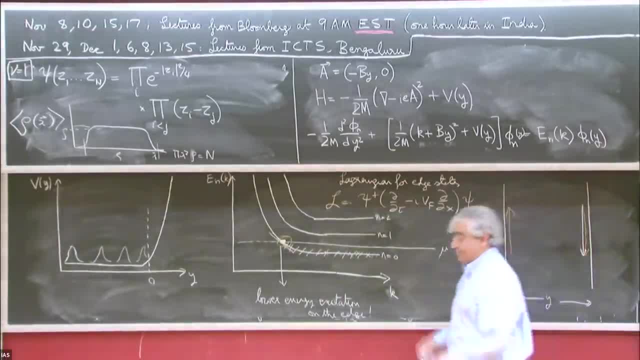 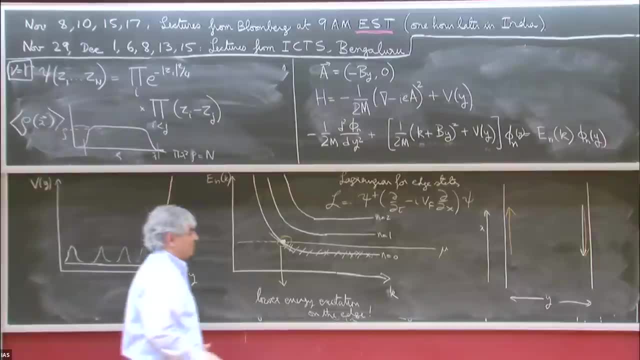 Now these edge states are really important in this case for physical properties. If you now put a voltage and you drag the current to the sample, then, as I said earlier, the states in the bulk of the sample carry no current. but these edge states certainly do carry current. 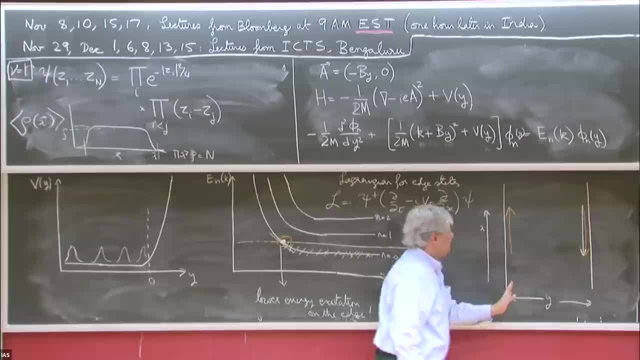 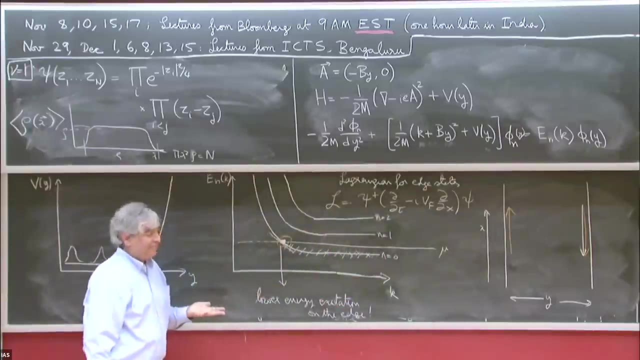 So you can drive a current and the current will move downward from this edge and upwards on the side. So any transport properties at low enough temperatures, especially the Hall conductivity, is completely dominated by the X-states And you can compute the Hall conductivity of the X-states. 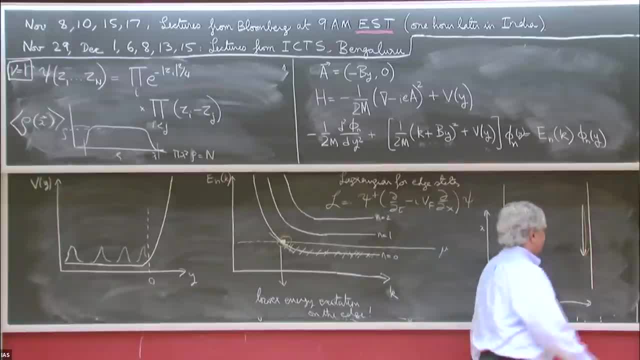 That's done in the notes, I won't do this here. And you find that the Hall conductivity of sigma X-y is E squared over H, And the fact that this one time E squared over H corresponds precisely to the fact that there's exactly one X-state here. 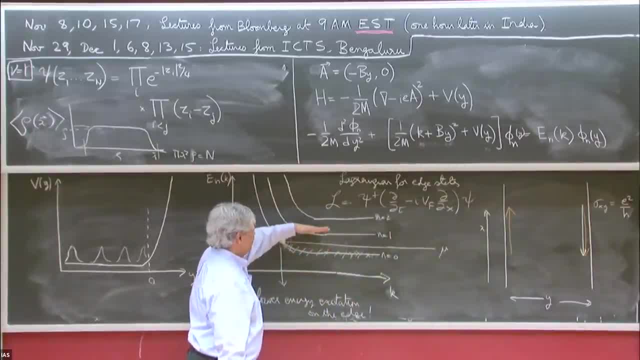 So if you raise your chemical potential and you started getting H-states, the second H-states, then you'd have a transition to a state which has sigma X-y is two E squared over H. Subir, how did you derive this, Lagrangian? 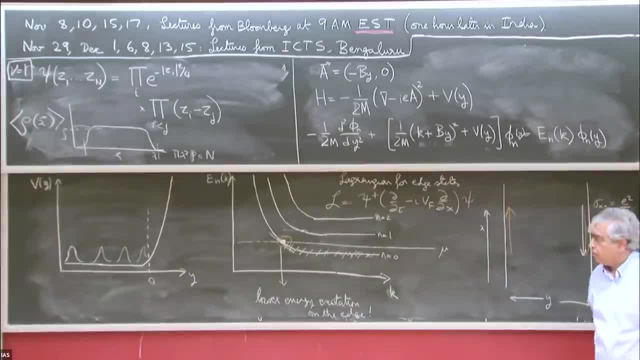 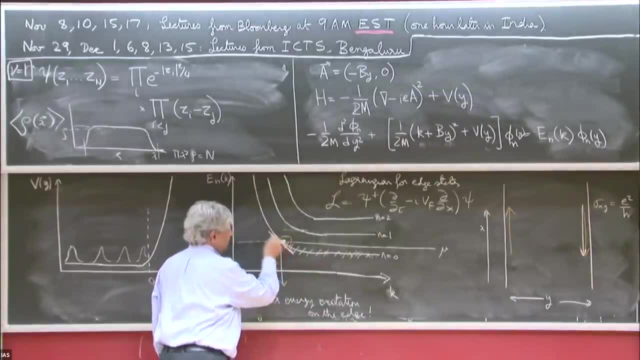 for the H-states from the Landau levels. Well, so the only thing I need to know is the velocity, and the velocity is just a slope here. So the slope of this curve, the EDK, is the velocity. So I have to solve this equation. 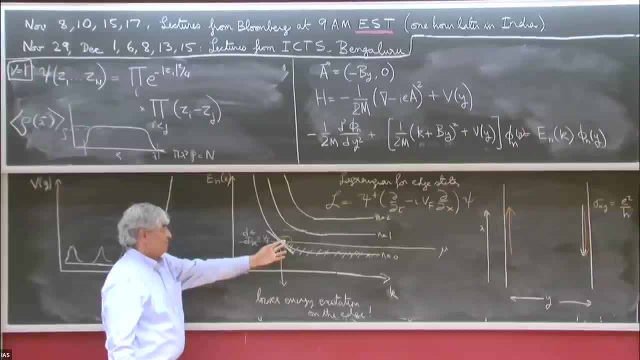 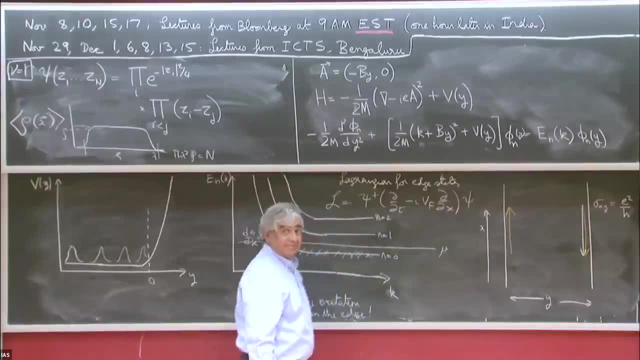 I have to get the energy dispersion. I determine the velocity of the chemical potential, and that's the only parameter I need to know to describe this one dimensional gas, And Seidegger would refer to the-. So this is, you know, some quantum field here. 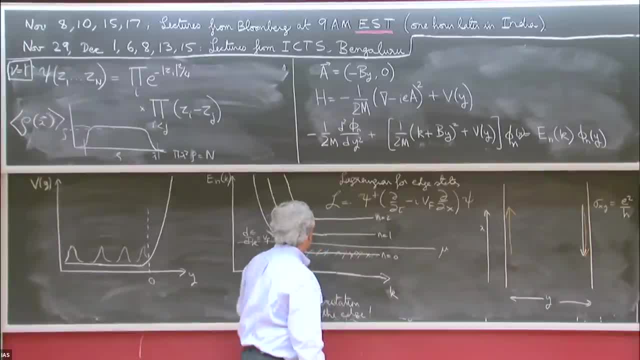 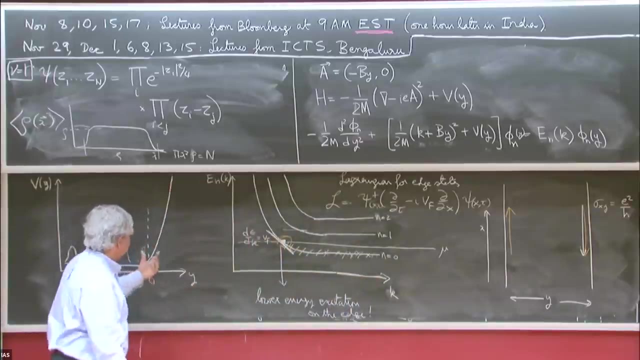 a fermion field which is living on the edge It has. so psi is a function of X, only It creates a particle. psi is Seidegger, creates a particle that lives on the edge, lives over here. It has like a Gaussian shape in this direction. 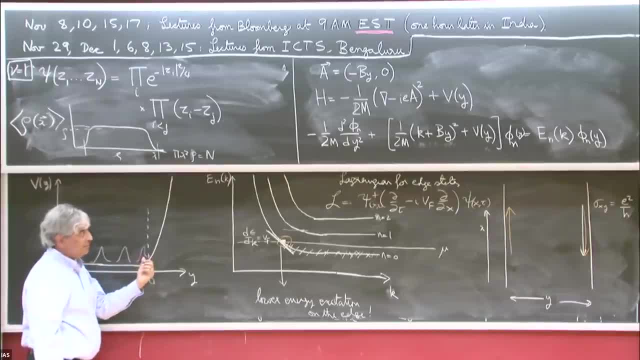 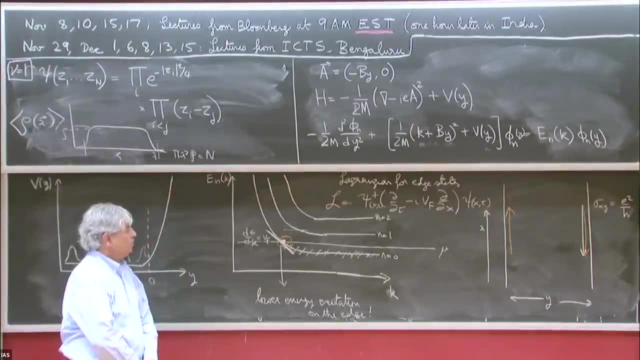 And it's a plane wave in that direction, in the Y, in the X direction, Understood, And the equivalent case for the bulk would not have this V term at all, right? No, The bulk has a V term right. 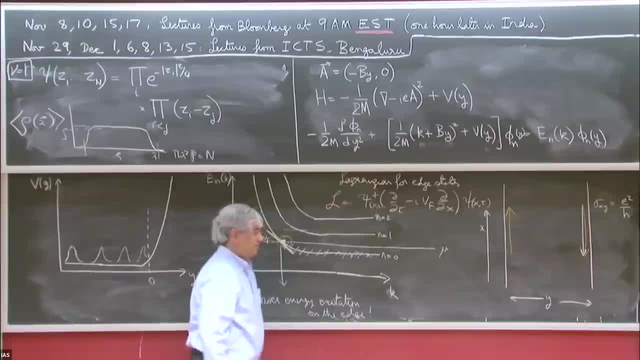 has a gap so you wouldn't be writing it down in some low-energy theory. for the bulk You really have to go back to the full Landau levels and there it costs a finite energy to add or remove any particle Fine. at the edge it costs zero energy to add or remove. 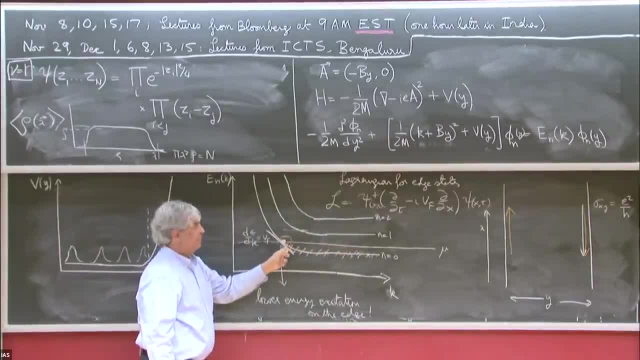 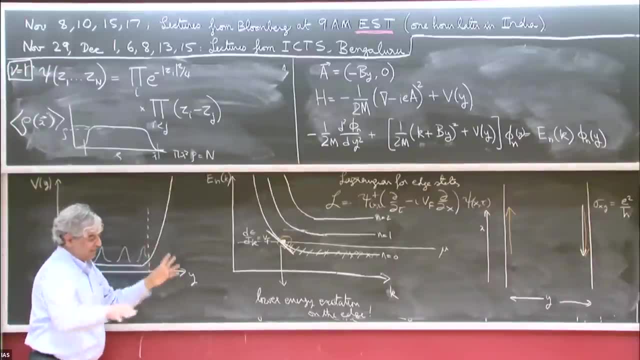 a particle, and that's the only set of particles I'm focusing on. So all of the particles I had on the edge have a Gaussian wave function in the y-direction- I know that I just integrate over that- And they're plane waves in the x-direction. So then this is the Lagrangian. 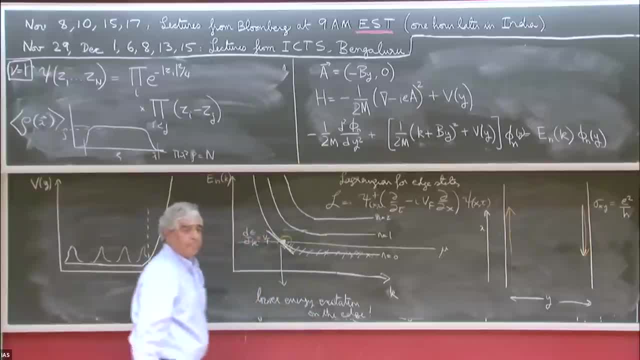 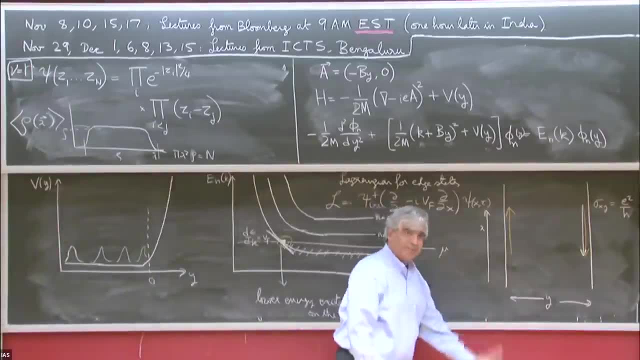 equation to describe plane waves in the x-direction. Thank you. There's three particles moving only in the x-direction or the minus x-direction, depending on which edge you're at. I have a question. So I know the conductivity is going to not be affected by putting in 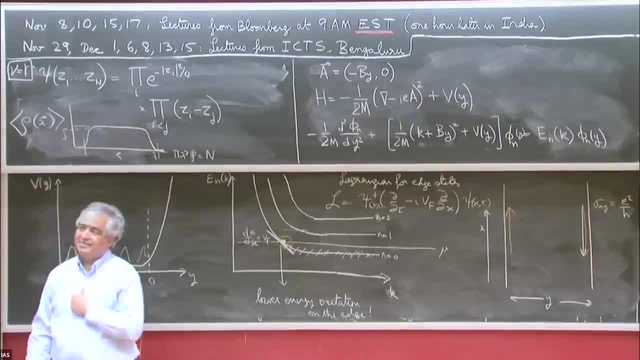 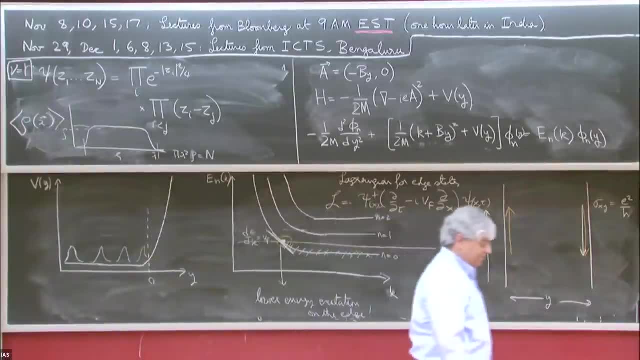 interactions and disorders. Yeah, yeah, What about Vf? Vf you computed from this fermion calculation. Vf is some parameter that gets changed if you put in interactions, right? Yes, So that's a very good point. So I related to what I was going to say. Thank, 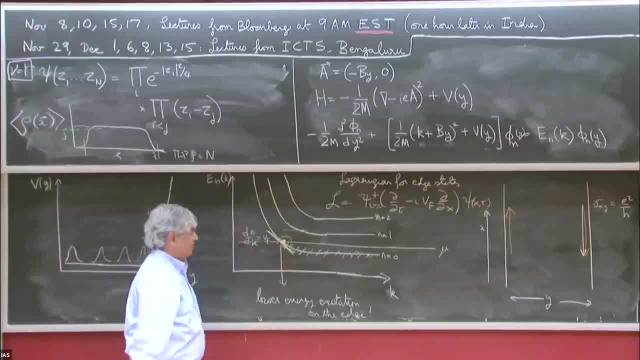 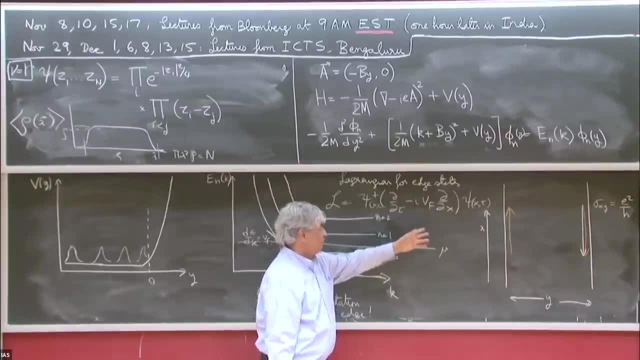 you, Tom, So yeah. So first of all, you put in lots of interactions. if you want, Take a general theory, Then you will certainly renormalize the value of Vf And you could also get interactions between these fermions moving along the edge. You could also put: 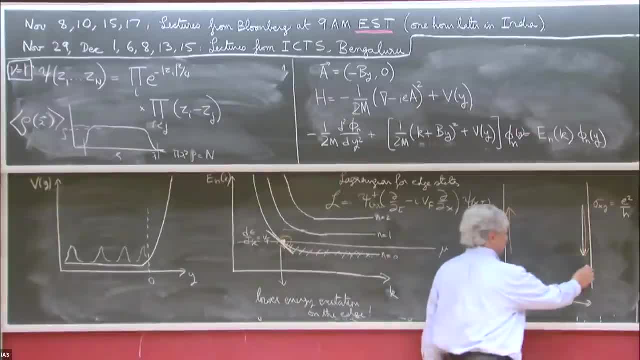 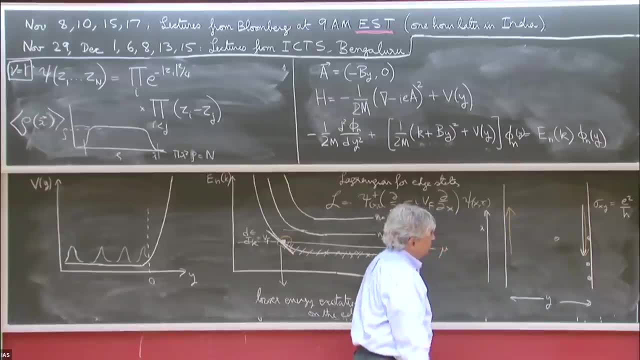 in some disorder, And suppose there's some impurities here. Maybe let me talk about those. So there's a few impurities sitting here in the bulk of the sample. Well, so the point is, first of all, those impurities don't change the conductivity. And why is that? Well, because 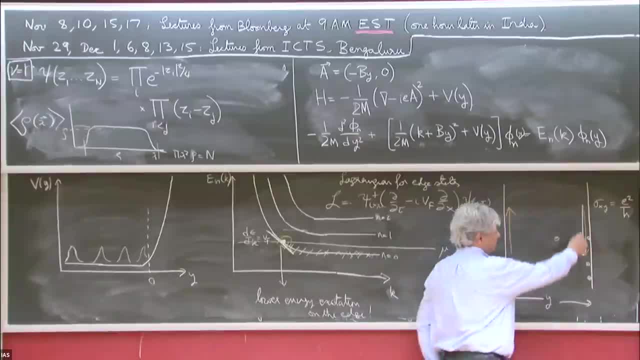 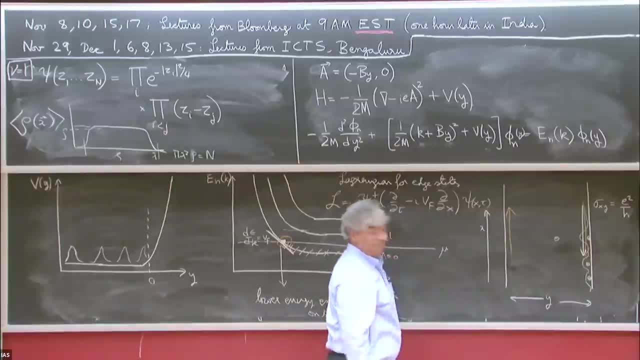 there's no—because the state is chiral. You know the particles are coming in. Well, maybe they'll go around the impurity, No problem It'll be—you know they'll still be moving in the same direction, But they never get backscattered. There's no way for them to. 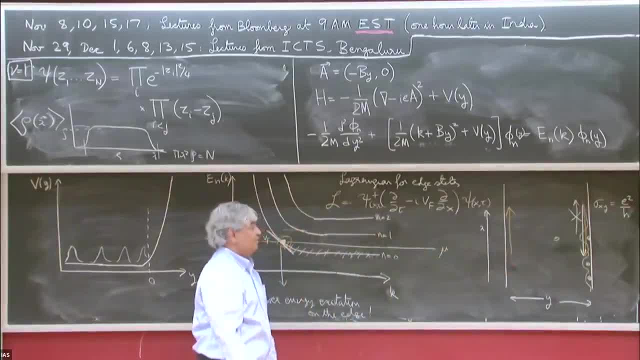 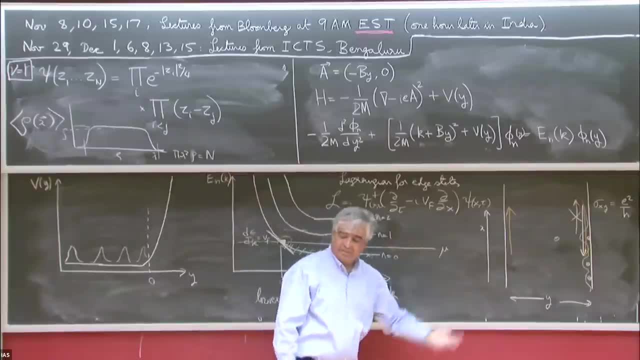 go in the other direction. So there's zero backscattering. The impurities don't matter. There's also interactions here. you can add That's—it's relatively easy to see that they don't matter, because full Fermi terms are unimportant at low energies for one direction. 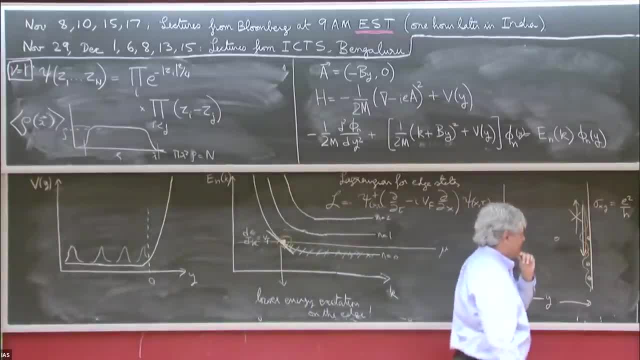 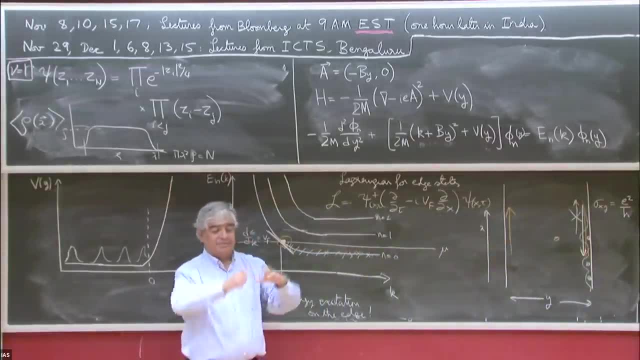 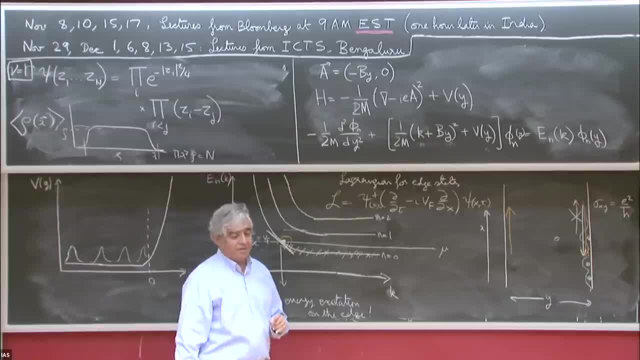 You could get a very good result. You could get a very good result, And then what they did is that they computed the conductor and computed its conductivity. The Landauer formula is that the conductivity is e squared over 8 and the trace of the transmission matrix. 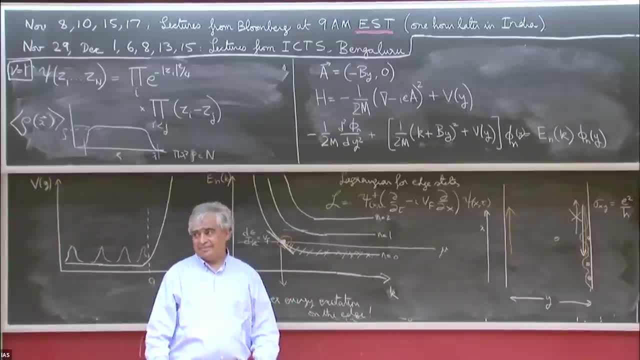 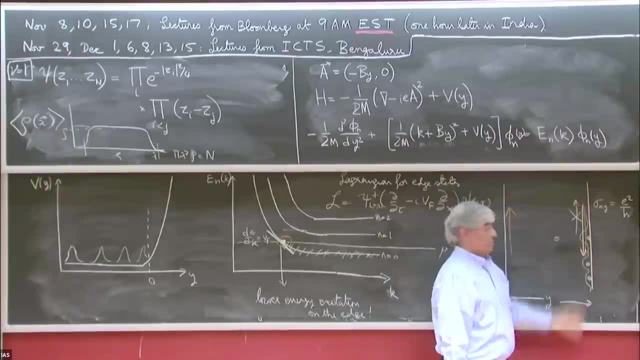 Even for a free electron gas, the velocity cancels out, It doesn't appear in the conductance, And so in the Landauer formula the transmission coefficient is one, because there's no way to get backscattered. So that ultimately—those are the arguments that ultimately justify 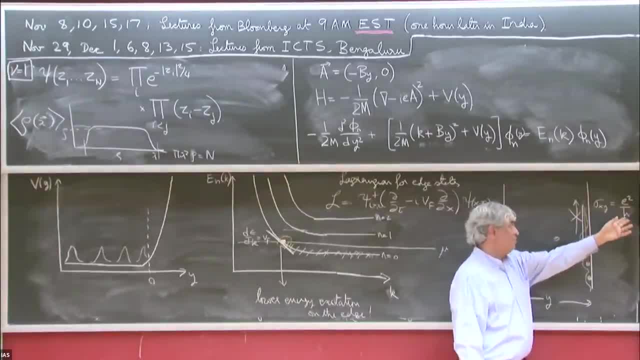 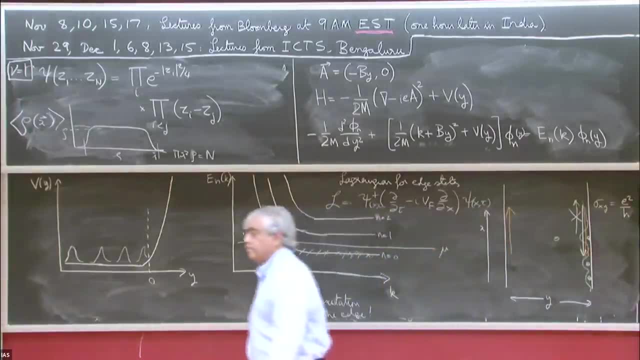 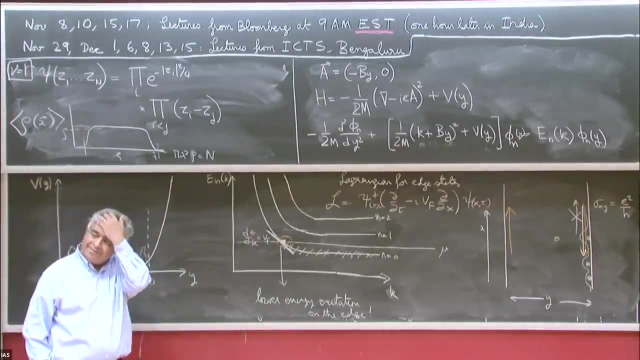 this is quantized and in fact now used as a way of measuring the value of the fine structure constant. The other question I had: last time you did a similar analysis but you actually got the wrong answer by this analysis right, Because there was this factor of 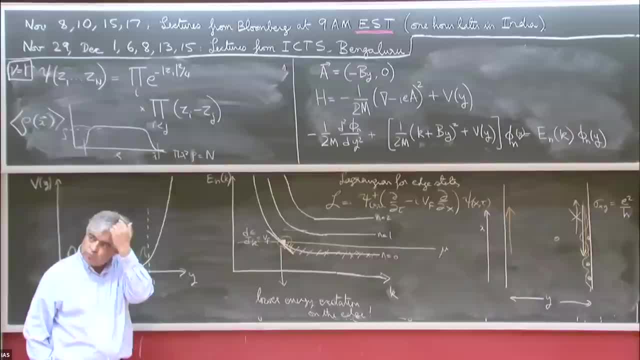 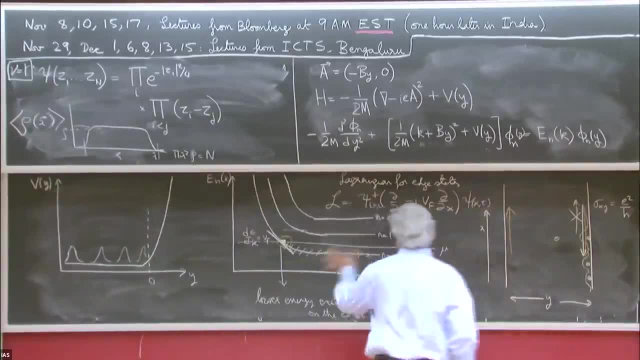 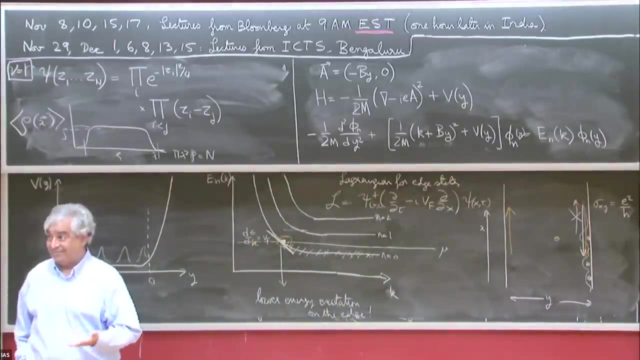 two. that came from the fact that it's level two, Kermit algebra. Oh well, so that here I go. yes, so I don't have any gauge fields here, right? So there I had a gauge field which leads to very singular interactions which we will get in the fresher quantum Hall effect. So you will need 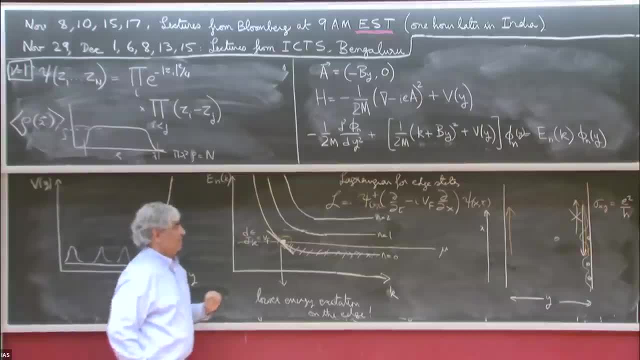 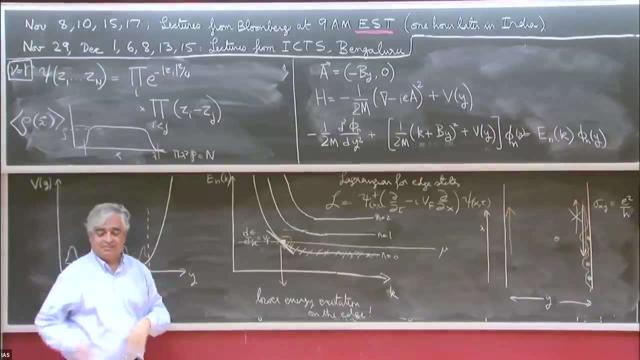 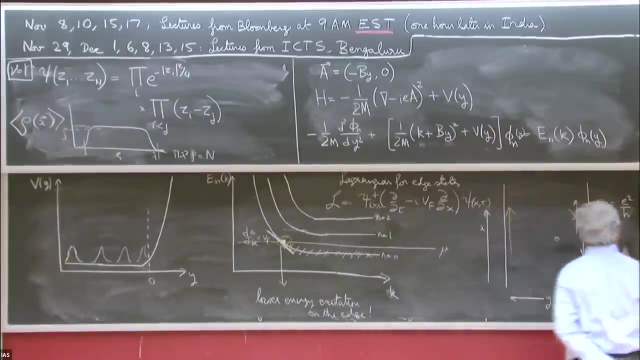 those gauge fields to go away from this integer value. Here I'm just talking about ordinary Coulomb interactions which are typically screened anyway on the edge, so they're not as singular as the gauge field. So we will need the gauge field if you want to move away from integer values. 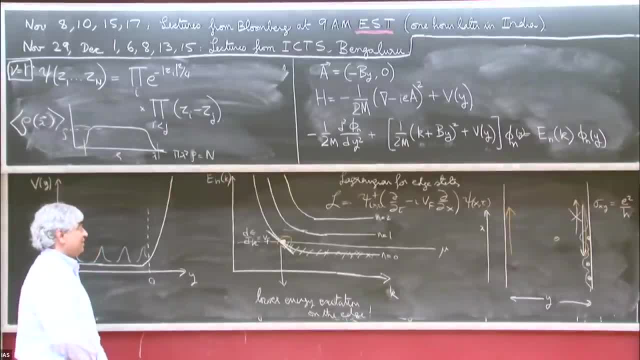 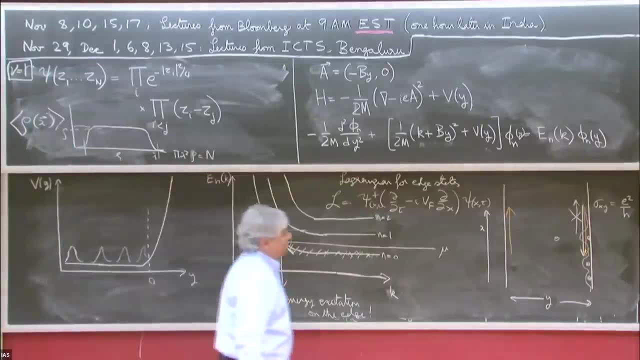 Okay, any other questions? I have many other topics to get through and I could certainly say much more about it, and there is a fair bit more, including explicit calculations of this in two different ways, using either the bulk approach or the edge approach. In both cases, 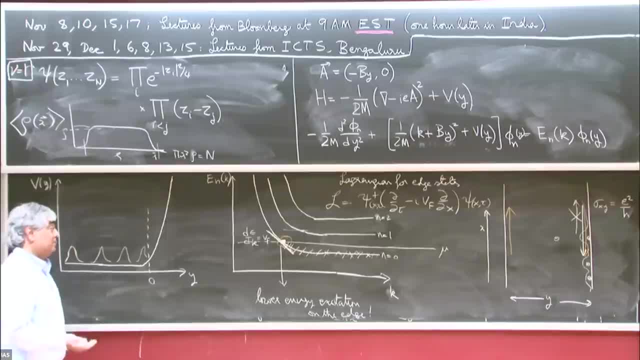 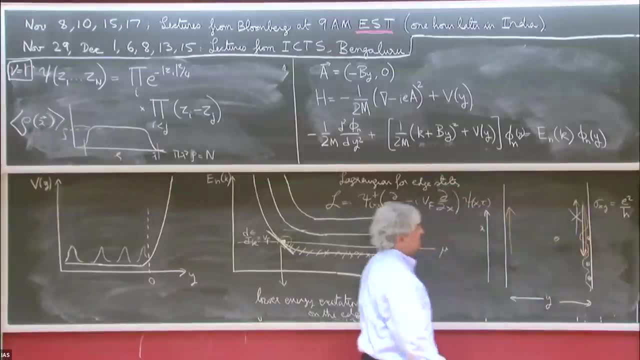 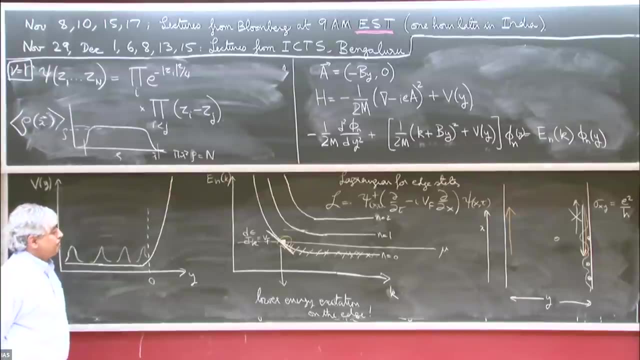 you get the integer answer. The edge approach is much more instructive because it's really what you need to understand: the generality of this result. It has no corrections whatsoever. I have one naive question: Yes, please, At this level, can I see from the 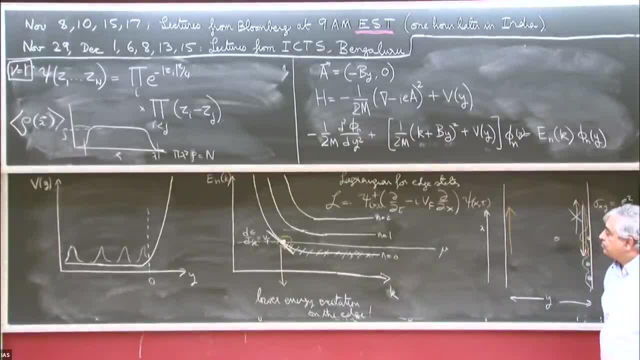 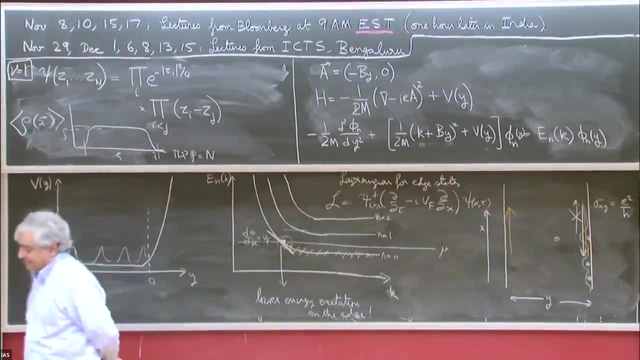 theory of the edge that a bulk is required for it to exist. Yes, yes, Yeah, so that I guess it goes to these so-called anomaly inflow arguments, and I know I keep saying this, but that is also in the notes. So if you take this theory and couple it to an external electromagnetic field, 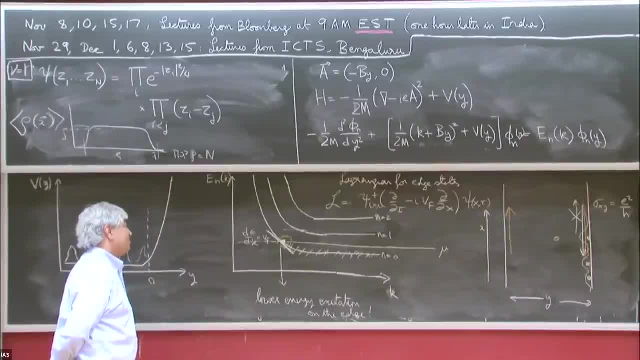 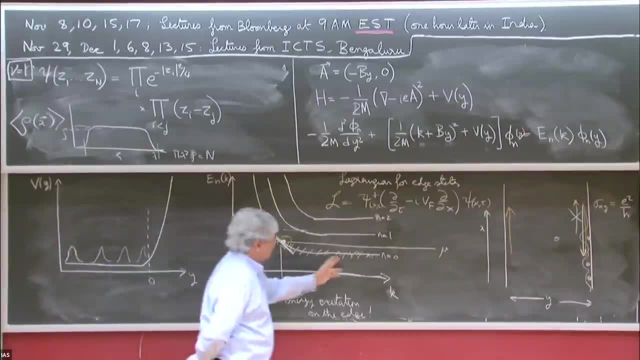 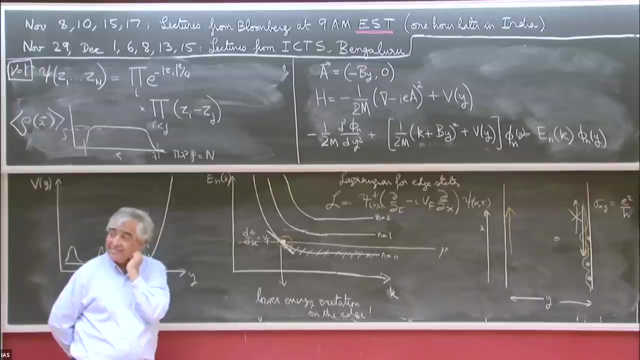 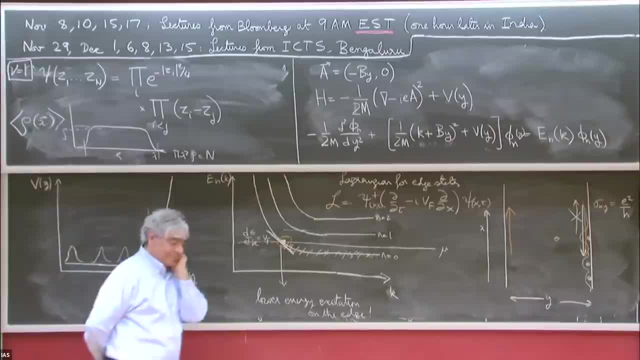 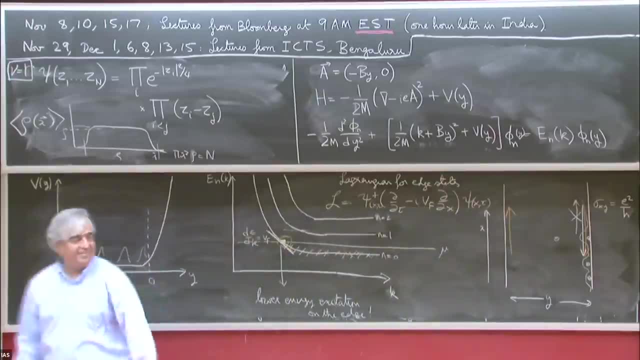 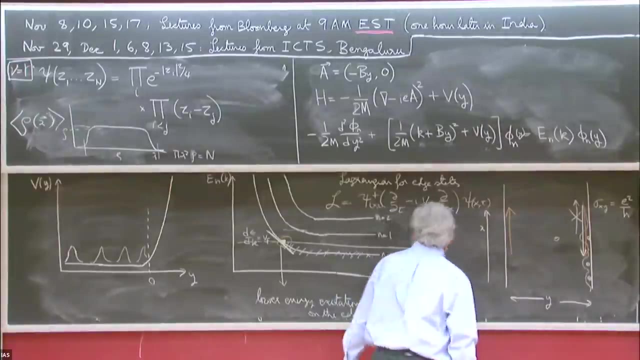 It's anomalous. Okay, thank you. Right, Yeah, which is, I guess, what Nadia was also objecting to last time. Yes, Okay, All right. So now I think that's really all I want to say about the integer quantum hall effect. 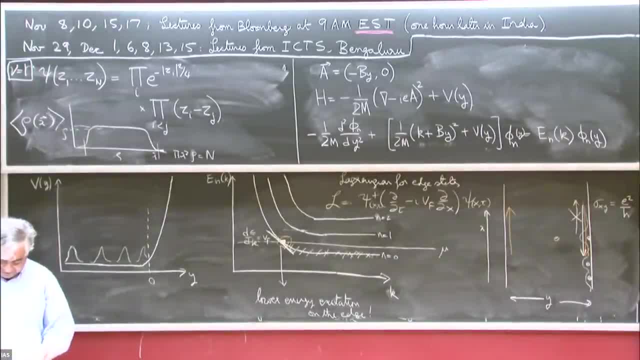 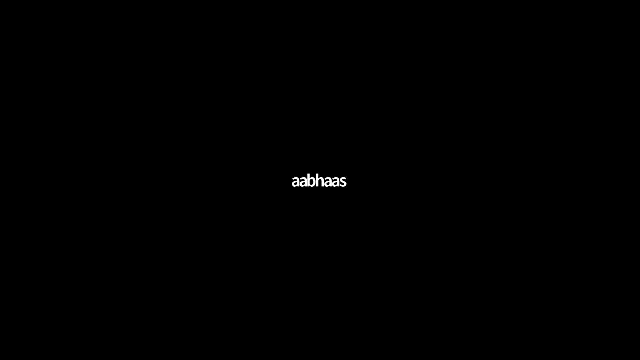 And now you can jump ahead to the rational quantum hall. Thanks, Any further questions? One small clarification? Yes, please, It's a more of an intuitive question. The way you derived it, it looks like the current really flows on the edge. 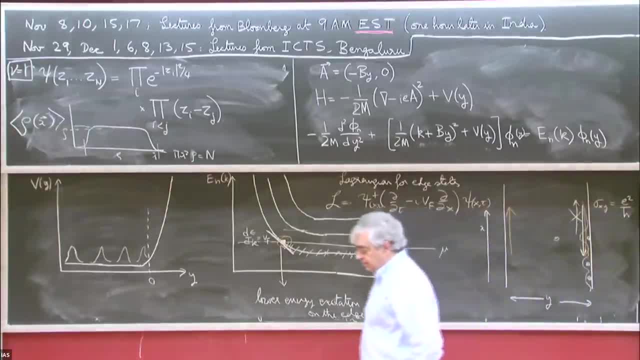 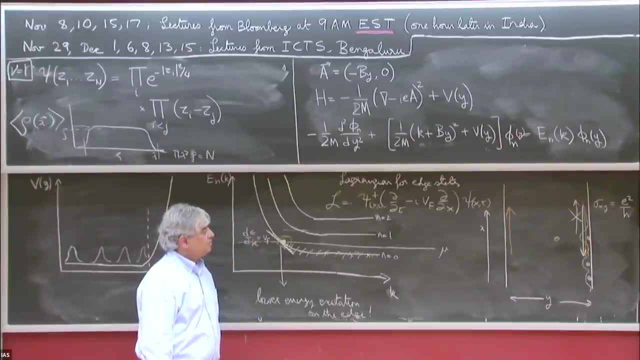 Yes, But it also needs the other edge, the bulk. So is there a sense in which the current flows also in the bulk, or is it only? or is it always the case that it's only on the edge? It's always on the edge. 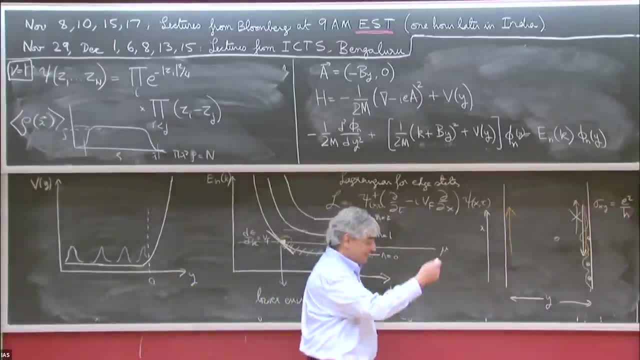 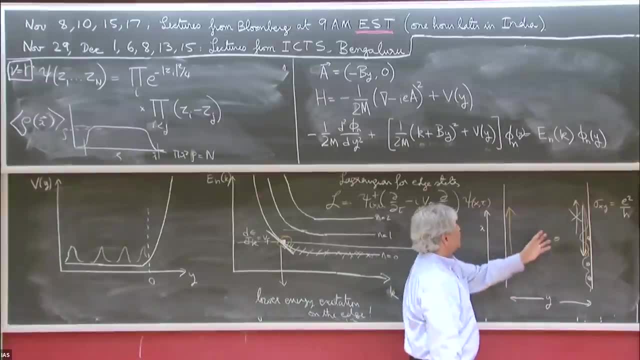 I mean you can measure the current. You know people can come in with various probes and see what the current is and you can see it's only on the edges. Yeah, So there are states in the bulk that if you take any given state you'd see there's some current. 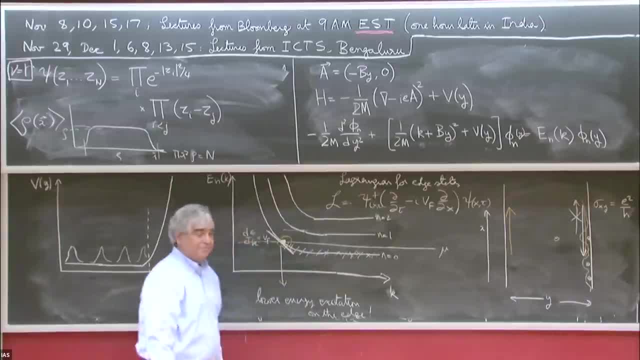 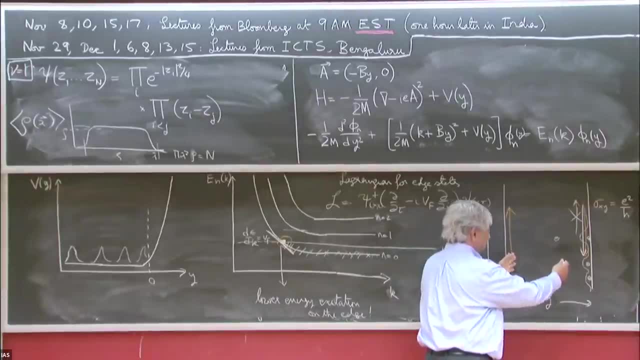 But when you sum over all of this occupied state, the net current is zero. I see, Thank you, And in fact the whole conductivity is: you know, to drive a net current you have to have this: The current here is not exactly equal to the current there. 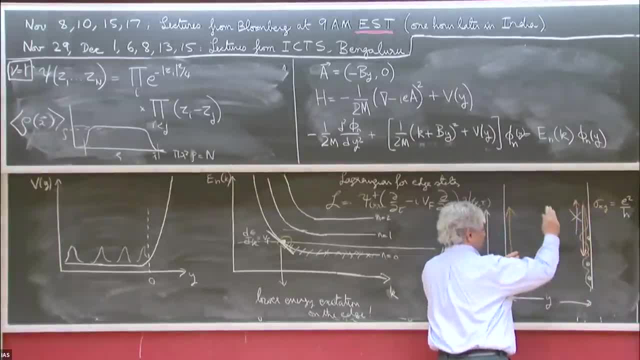 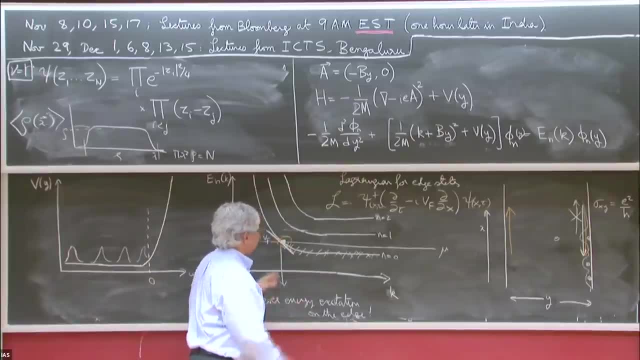 So there's a difference And the net current that you will be driving, the sample is the difference of the left and right currents And from that, and using a few general arguments, you can then see why there's a whole voltage that will develop a character. 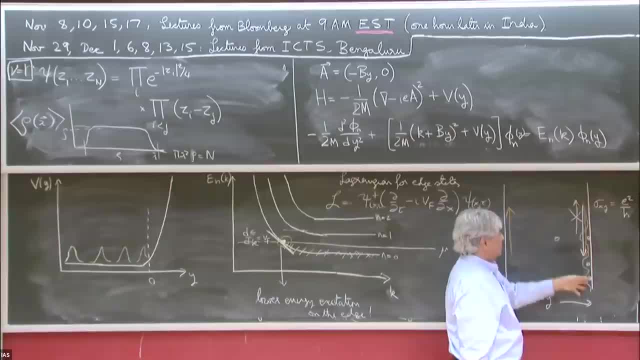 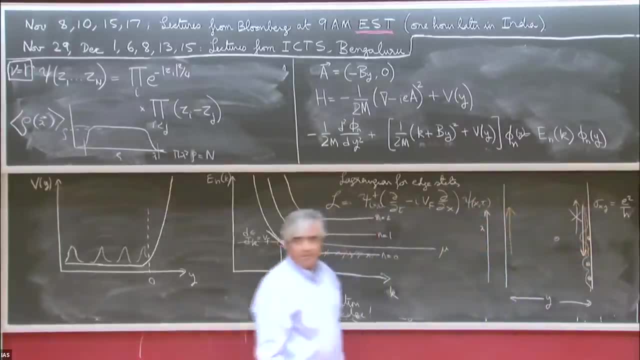 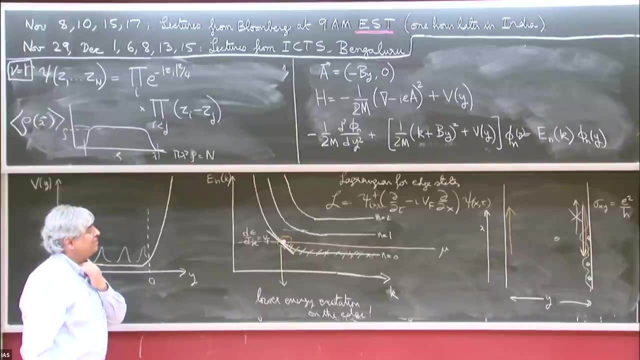 So that's why the linear, in the end the linear conductance of this edge theory is in fact related to the whole conductivity, The whole conductance of the whole bar. So yeah, there's a lot of interest on that with using the Landau-Budecker approach to 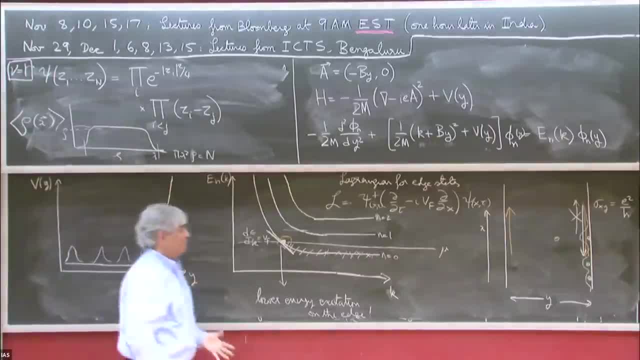 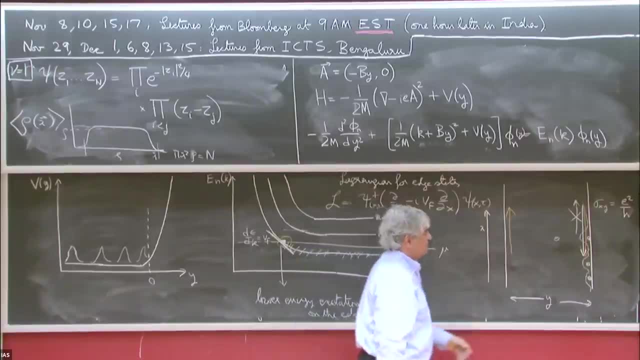 all of this And that's essentially exactly all you need for that is, you know, the various leads on your sample and, at very low temperatures, the collision coefficients of all the edges. Of course you can get in some cases in the fractions, quantum Hall states. 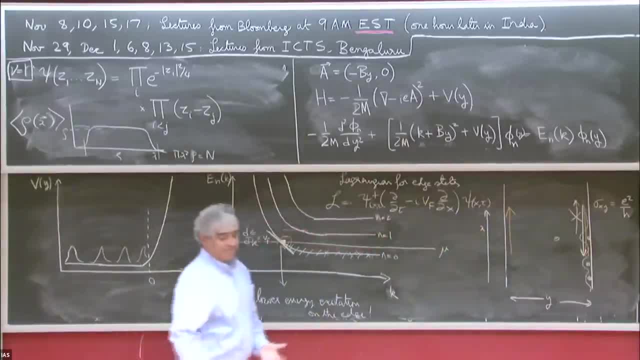 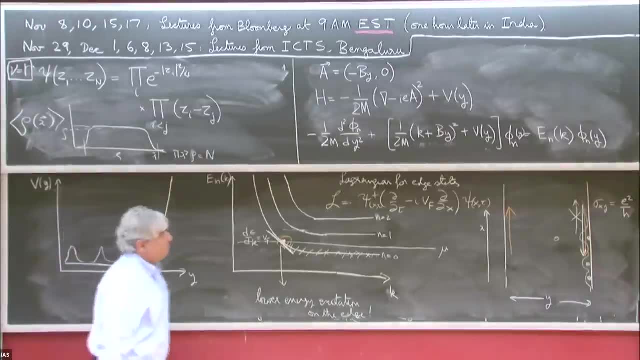 very exotic edges, which are non-trivial conformal view theories, And yeah, so we'll get to those in a minute. Can you please say briefly what does one mean by an anomalous theory, or what does anomaly mean? I'm afraid I can't, because I can't be brief. 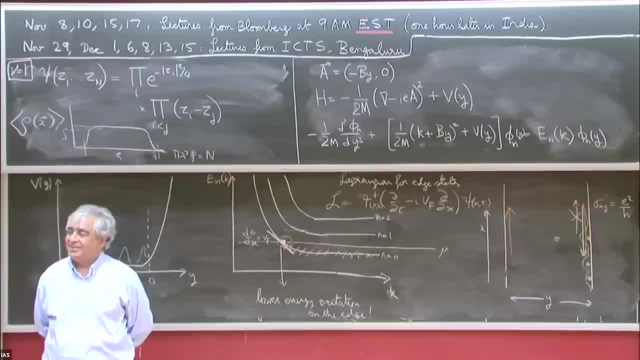 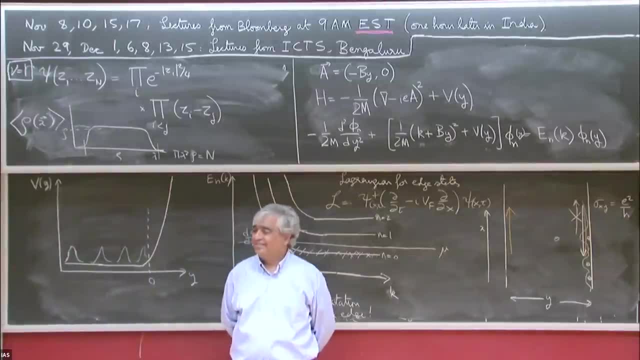 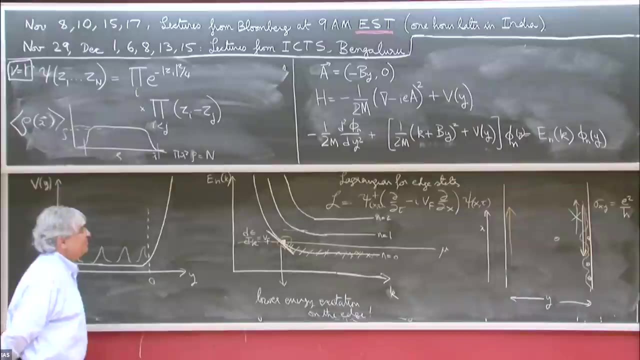 But the more important reason- I'm not sure I understand it well enough to talk about this. Maybe Tom, or Not even to attempt an answer to that- No, Yes In one word, if you just look at this Lagrangian that you wrote and you add the gauge field. 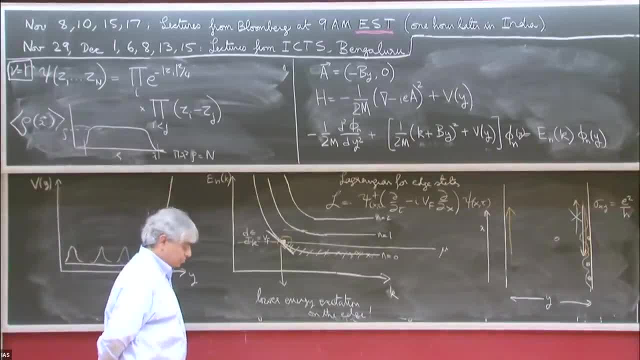 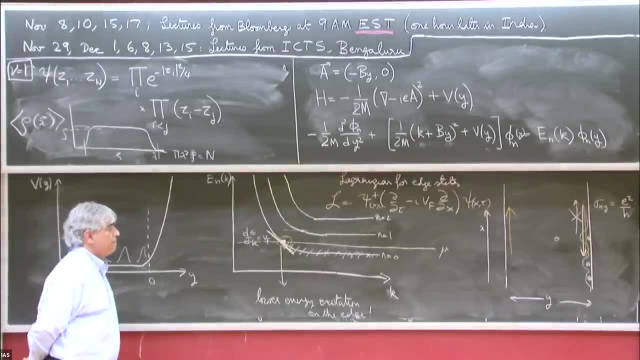 and you try to integrate out the fermions. this is just a determinant. It's straightforward to integrate it out. The result you get is not gauge variant, And that's what's That's called the anomaly. I mean that doesn't mean the theory is inconsistent. 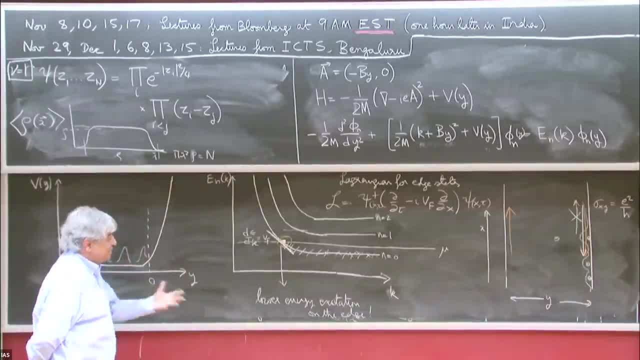 It just means that if you put an external gauge field, then the final theory will not be gauged in better respect to that external gauge field. Yeah, Yeah, It's not an inconsistency in the theory. Theory is perfectly consistent, Okay. 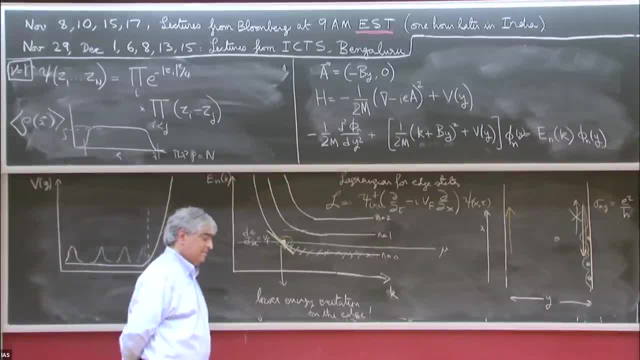 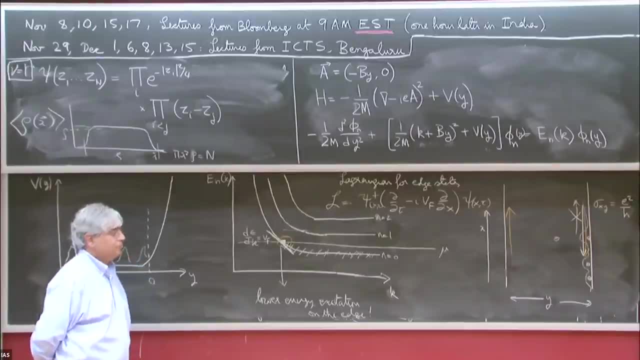 Yes, I know, I was just going to suggest the following. Suppose you only have one edge. You apply an electric field which accelerates the electrons and makes the Fermi level go up, And if you have only this one band, it would change by the electric charge conservation. 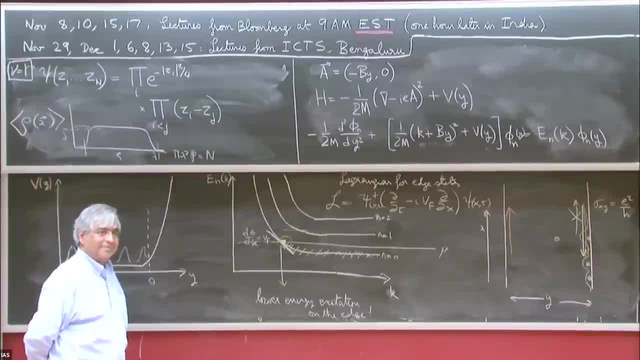 When the Fermi level goes up, the electron density goes up. Okay, All right. Okay, So I hope you could hear that. Okay, that's good. Thank you, Actually, I could not hear it well. So what Edward said was that if you apply an electric field, 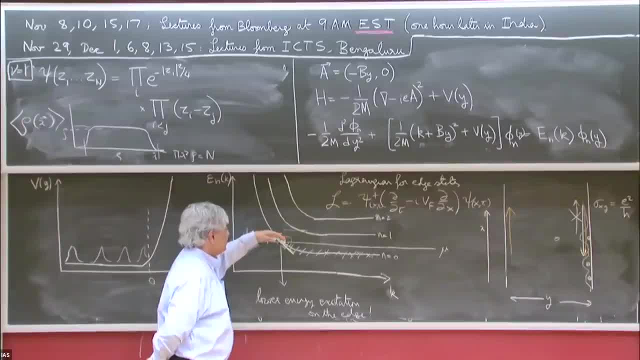 then the Fermi level will move up here over here And therefore you get a net charge on the left edge And the question is where that charge comes from. So you end up violating charge conservation, Because charge, if you accumulate on one side, has to come from the other side. 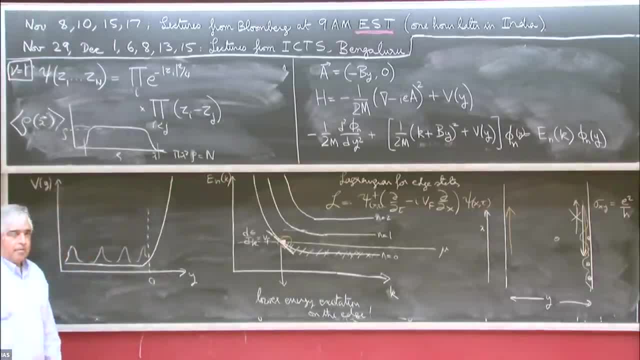 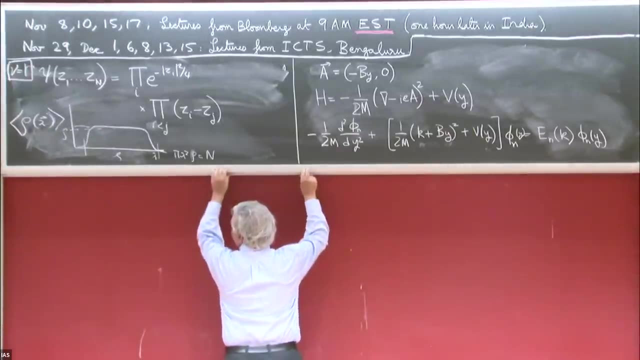 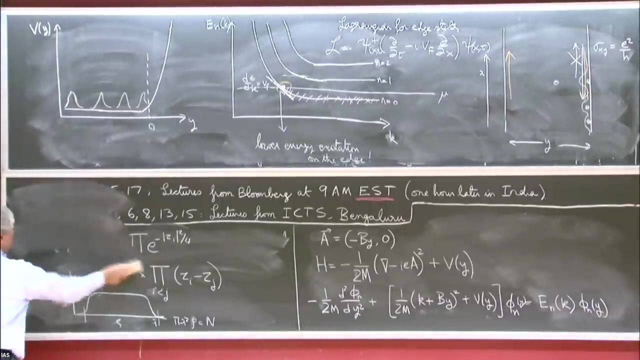 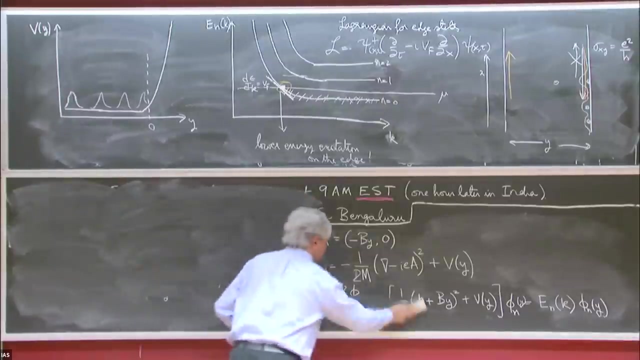 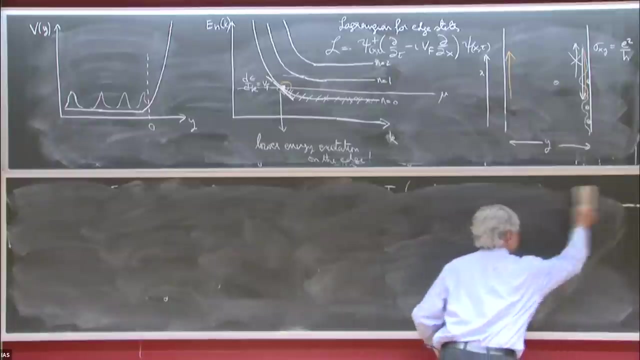 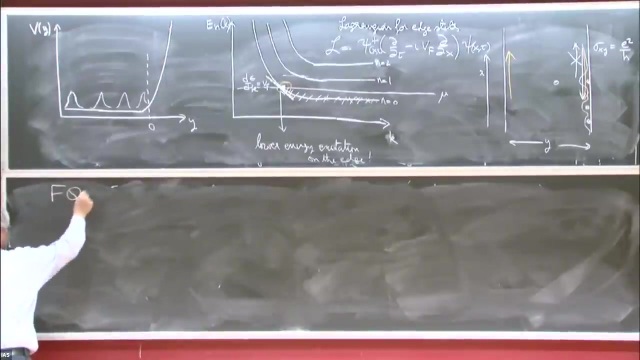 Okay, Thank you. Okay, Right, So now let's just jump ahead to the Fraction Bottom Hall effect. So I'm going to use the part-time approach. And this was- This context you know, rather explicitly discussed by Jane very early on 1989 already. 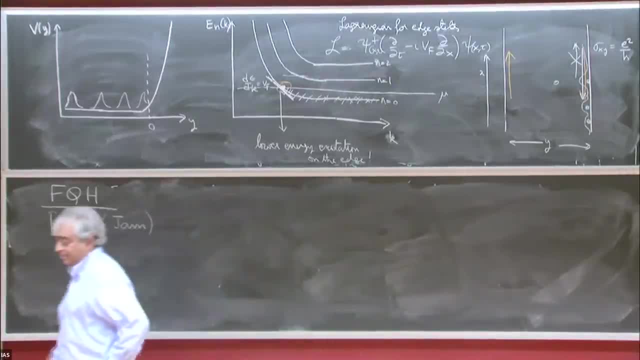 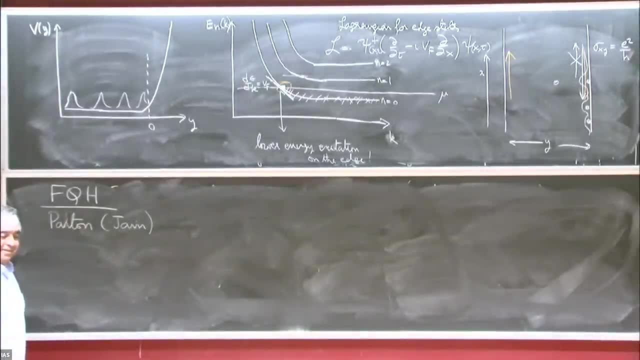 around the time he wrote down the famous Jane states, which we'll also talk about, But strangely enough it hasn't been used much in the literature since then. For the benefit of hindsight, I think this is the cleanest way to do a lot of things. 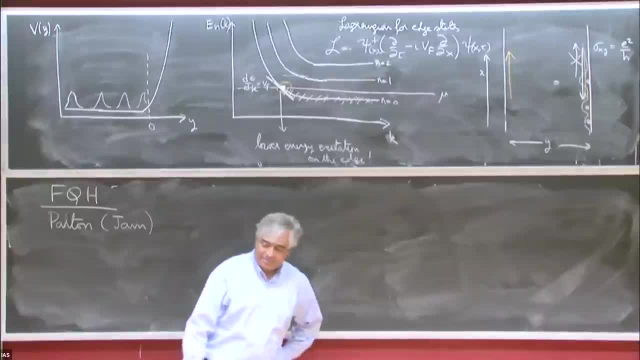 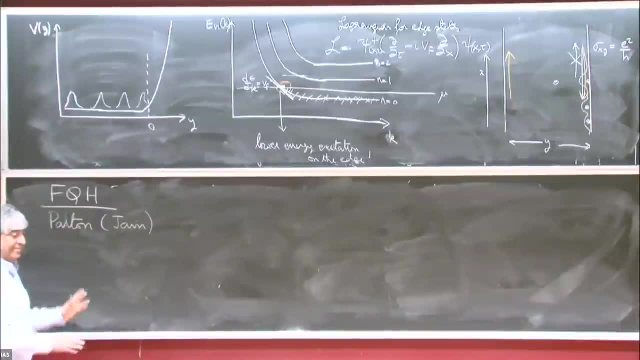 Much of the condensed matter literature uses flux attachment, transformations and dualities and they can be highly confusing and often not interesting. But this one, at least formally at every stage, is well-defined And it does actually give you a very compact description of the important quantum Hall states. 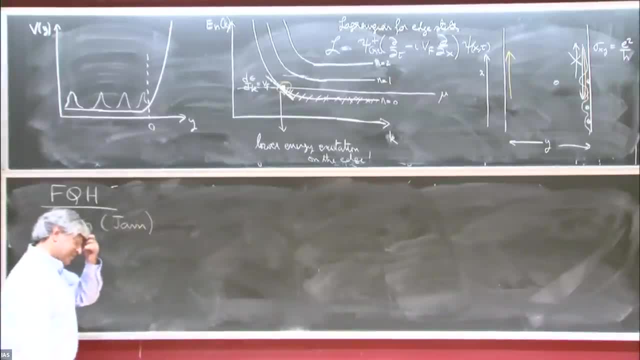 particularly most of the ones that have been observed. So let me just discuss it. So, what we're going to do, we're going to take our electron operator, which I'll call C and no spin here, And I'm going to decompose it into three fermions: the part-d, the part-trons, which are going to be here. 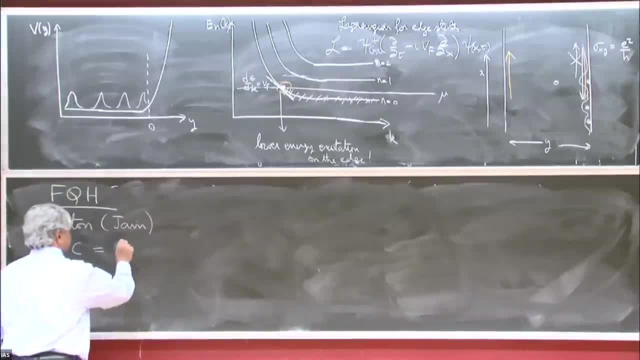 Okay, So we're going to take that. We're going to take the two fermions which are called psi 1, psi 2, and psi 3.. Okay, So you can imagine putting this on a lattice So you can put a site index if you want. 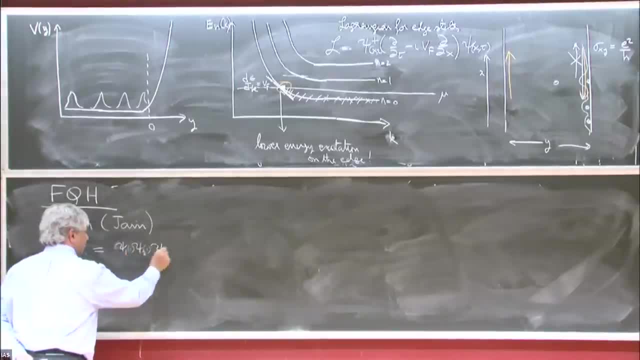 Eventually I'll just work in the continuum And this is just a very simple thing. On each side of the lattice I have two states: I have the empty state and I have the filled state with one electron in it, And that I'm going to just equate here, also with the empty state. 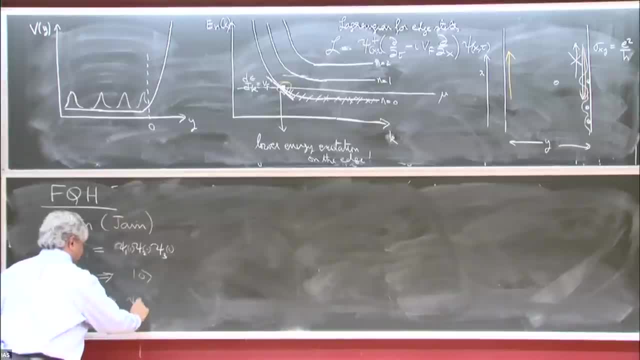 And this state I'm going to equate with psi 1 dagger, psi 2 dagger, psi 3 dagger. So now, if I had, if you really had, three part-trons, then you know they're independent. So the total number of states in my Hilbert space is eight on each side. 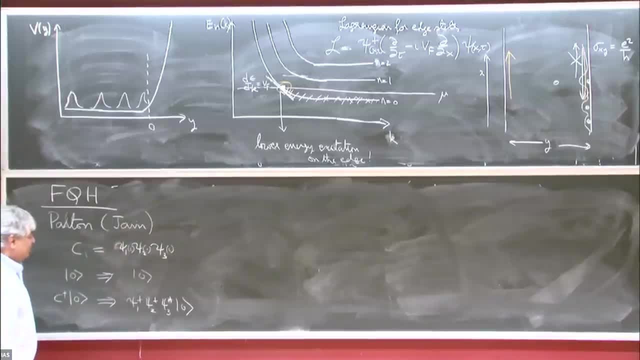 I'm going to declare all the other states to be illegal And demand that these are the only two legal states. Okay, So you could. it's sort of like a repetition code. You're representing 1 by 1, 1, 1.. 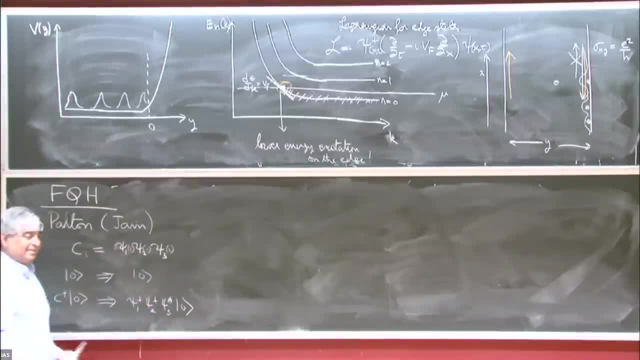 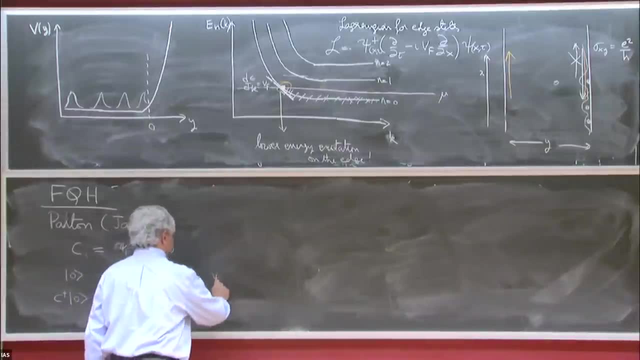 That's all, And all of the states are not allowed, Okay. So if you want to get this, these two states only. then you have a constraint, And the constraint is very simple: Psi dagger 1, psi 1 equals psi dagger 2, psi 2 equals psi dagger 3, psi 3.. 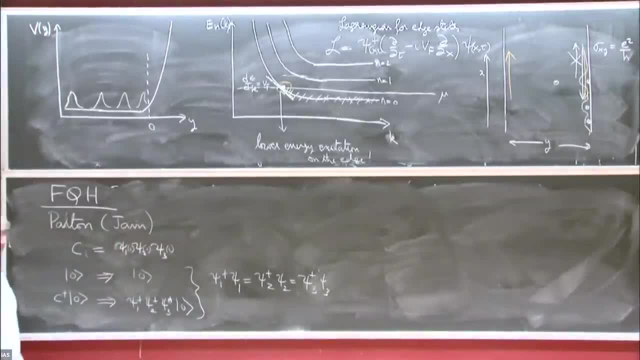 So if I impose these constraints exactly, then I will exactly restrict my eight states in the Hilbert space of the three part-trons to these two states. These are the only two states that satisfy both constraints, So I only need to impose two constraints. 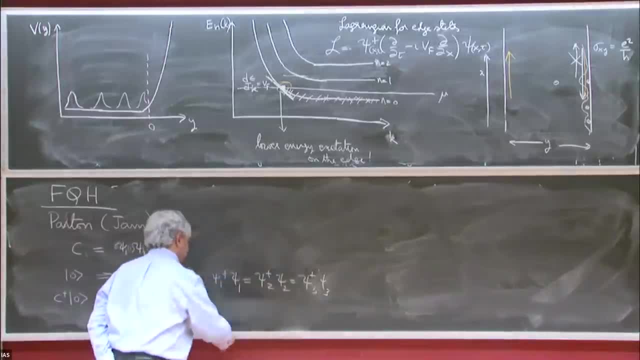 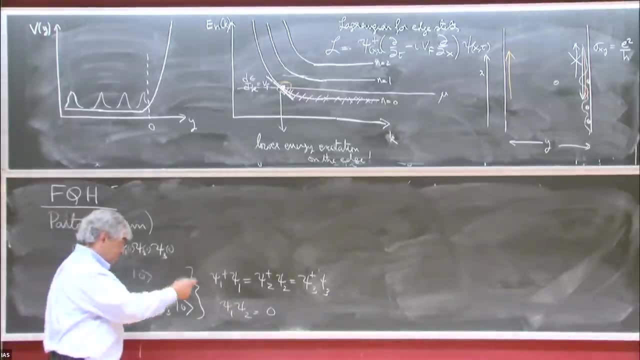 There are also other constraints which are implied by these. For example, like psi 1, psi 2 equals 0. Or psi dagger 1, psi 2.. So these are implied by these, But if you may want to impose them explicitly, 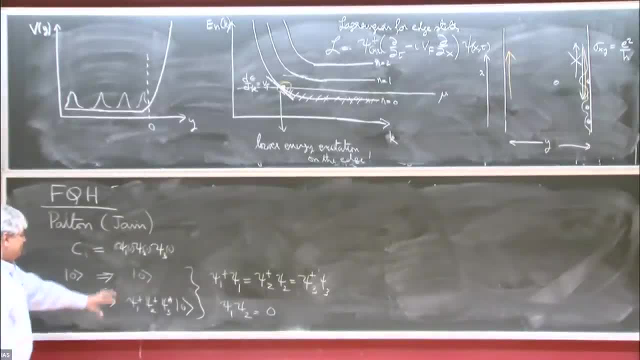 uh, in particular. uh, you can see that there's a certain SU symmetry here, And if you want to make everything SU invariant, uh, then you'll probably want to expose those constraints too as you go along. We're not going to bother with that, because just imposing these two constraints is sufficient. 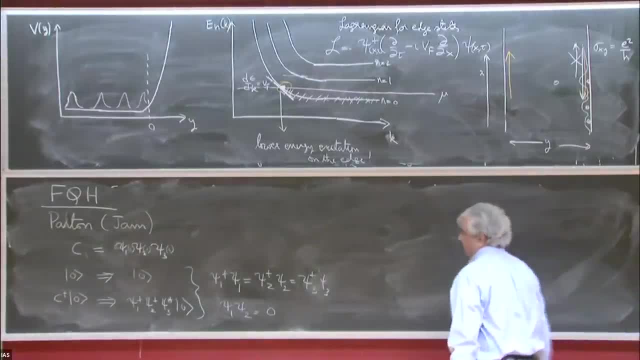 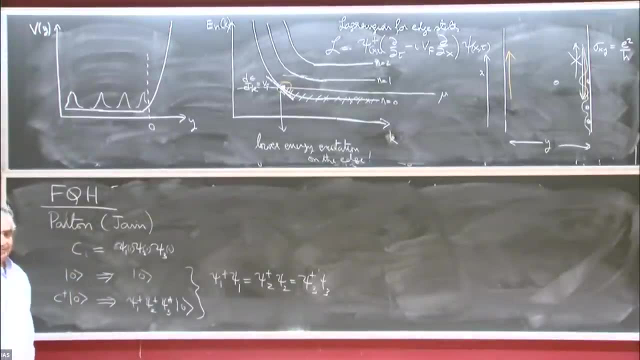 And so let's- uh, let's just stick to that And we're going to so only work with U gauge field, that we might expect rather than SU gauge field. But if you insist, sometimes you could work with SU gauge fields. 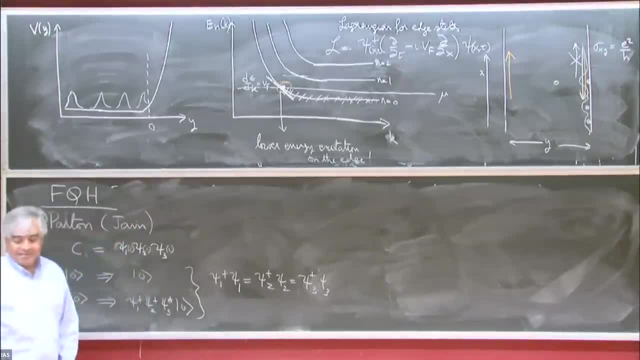 and then you can get even more exotic states. that could be important for certain non-obligion states if you care about them, But at this point let's just stick to the U1 case. So now, the point, of course, here is that if you have this constraint, 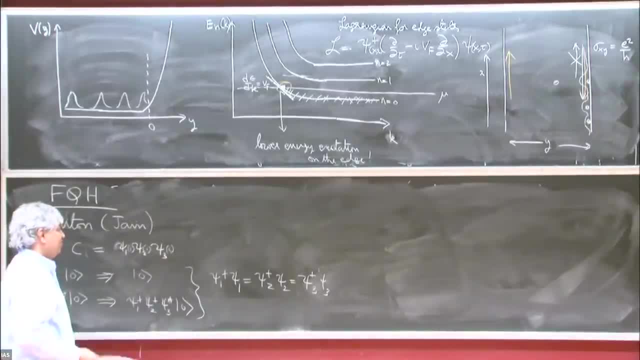 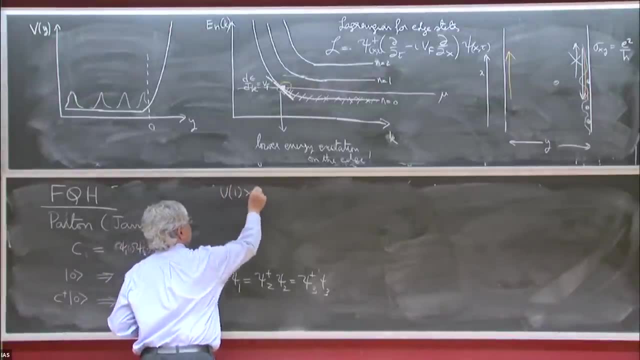 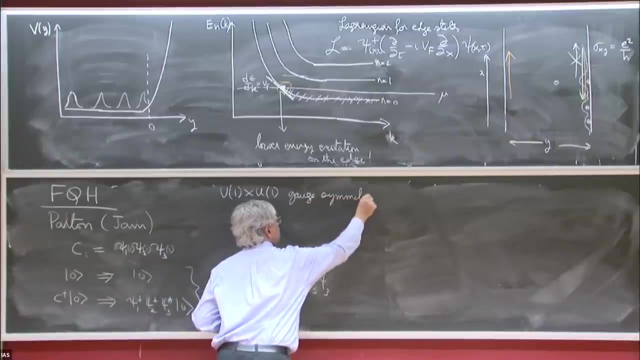 then you have a gauge symmetry, just like we had for the spins. So I now have two U1 gauge symmetries: U1 cross U2.. U1 cross U3.. U1 cross U1.. Gauge symmetry Which I will take to be: 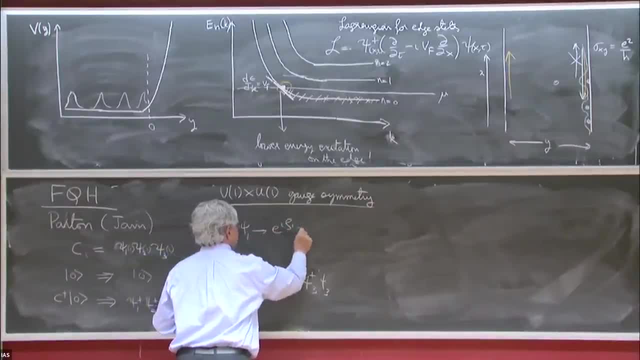 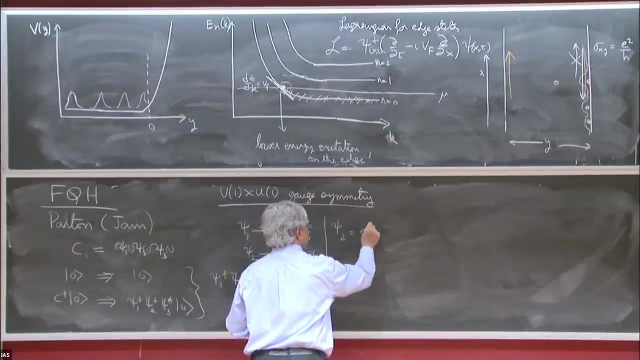 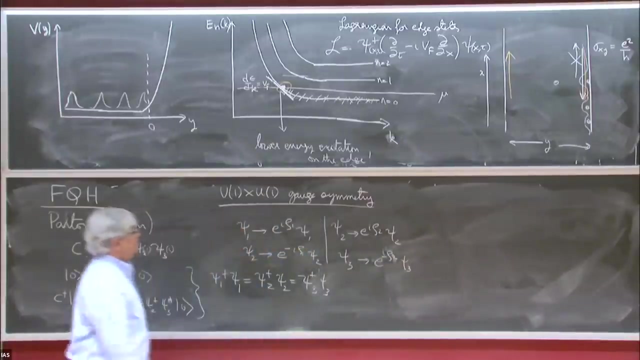 psi 1 goes to equal to I rho 1, psi 1.. And psi 2 goes to equal to that Minus I rho 1, psi 2.. That's gauge symmetry 1.. And the other one is the. 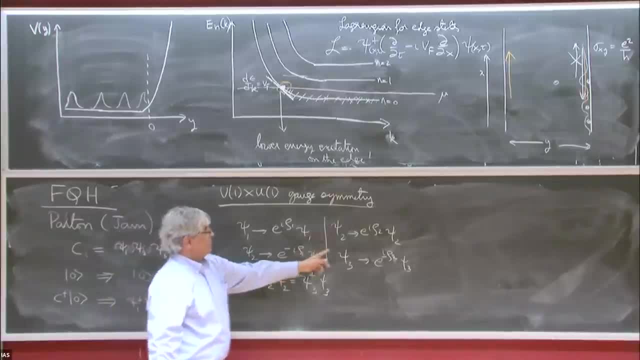 Gauge symmetry And you'll be psi 3.. Oops, Okay. Well, if I could just assign. so: I want to have a positive charge in the first gauge field, then psi 2 will have a negative charge. side two: positive chart of the first gauge field. 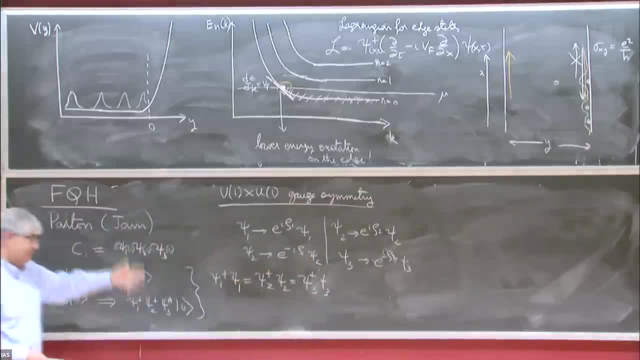 side three would have a negative chart. Of course, there's many ways of choosing it, and, okay, there's one way, All right, So now what you should really do- this is what we did for the spin system- is you want to take these onsets? 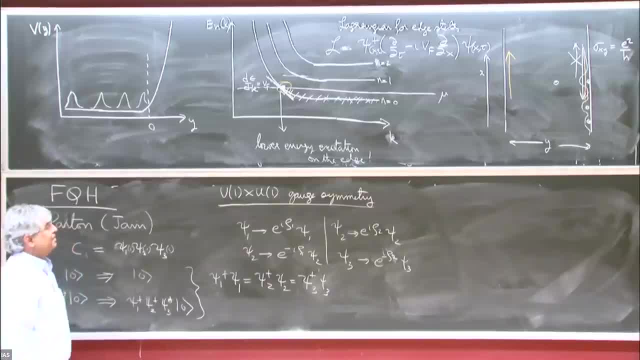 put it into your actual Lagrangian or Hamiltonian for your freshness point of all states or whatever, and then you'll get very complicated terms like C, dagger, C will become a six fermion term. Previously, the spin dot spin became a four fermion term. 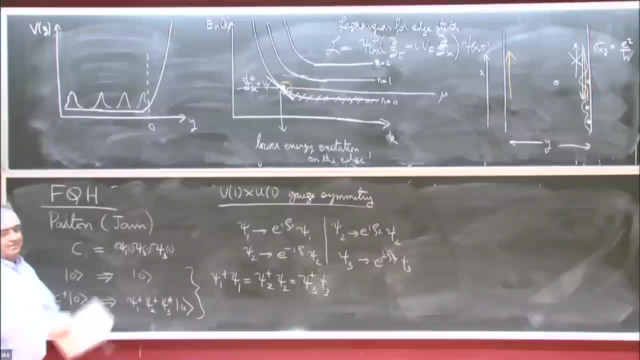 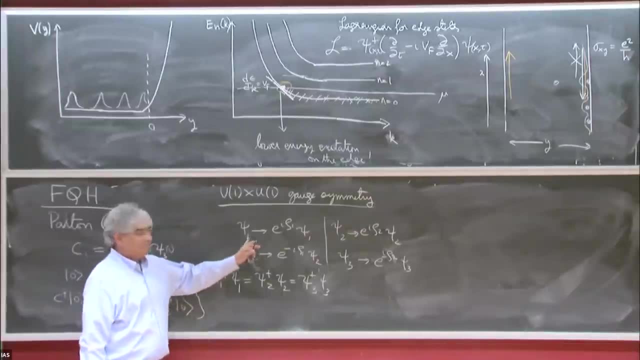 Here this will be even more complicated. six: So you get some very complicated Lagrangian and then you imagine that you have some saddle point at which these gauge fields are not fluctuating too strongly. So you take some mean field saddle point. 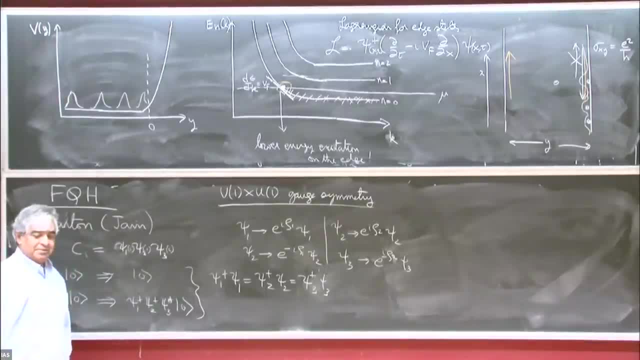 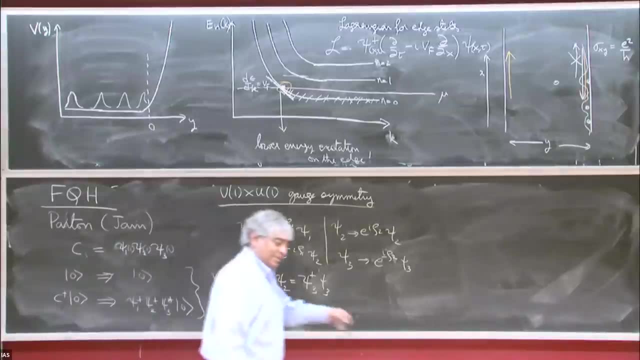 and then you do all kinds of how about? you're trying to decouplings, to write down a simple theory for the partons in the background of the saddle point. Now, all of those steps we laboriously went through for the Z2 spin liquid anyways. 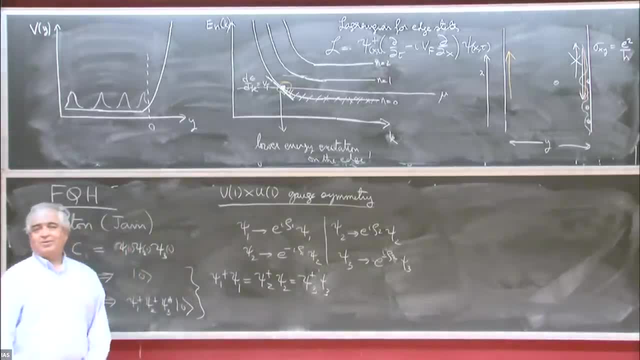 and maybe partially for the chiral spin liquid. but hopefully you're all experts at it by now, And so we'll just skip all the steps and just write down what the general structure of the effect of Lagrangian should be, just from gauging there. 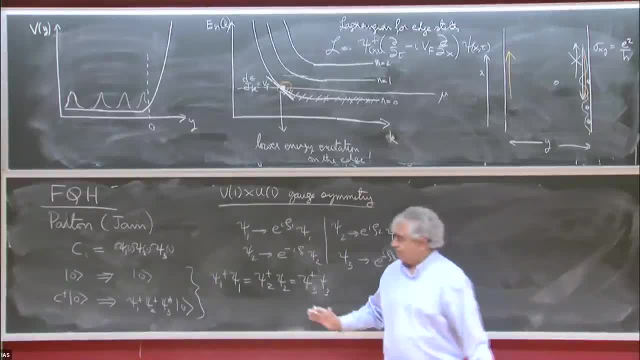 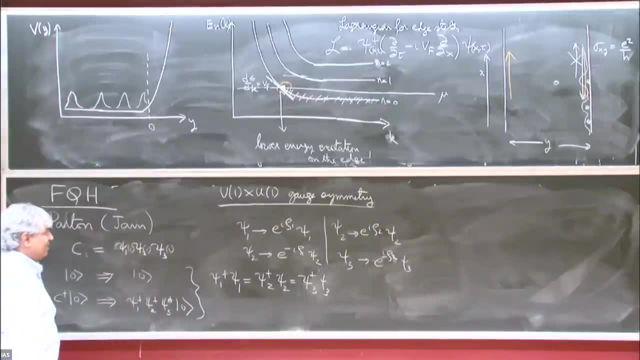 So in this case we are assuming that everything is moving. If you make this rigorous, you probably want a lattice, but let's assume everything is happening on a much longer scale. Everything is long wavelength on the lattice scale you use to define these states. 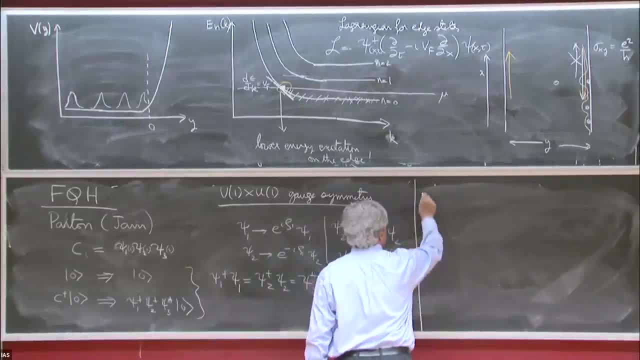 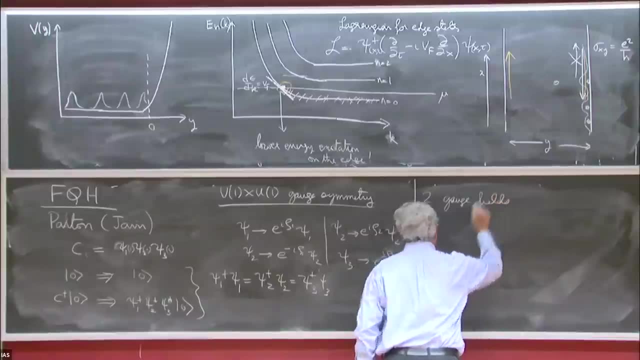 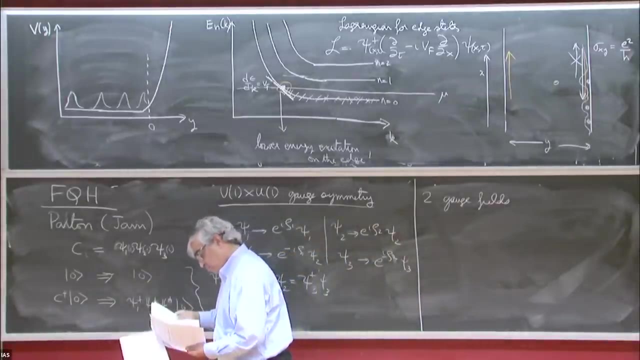 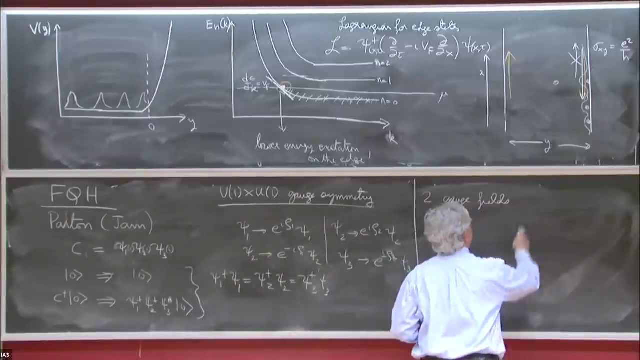 So what would the theory look like? So I will have two gauge fields. Let me see if I can use it in a minute. what would I call that? Oh, that's B. all right, sorry. So I have two gauge fields, B1 and B2.. 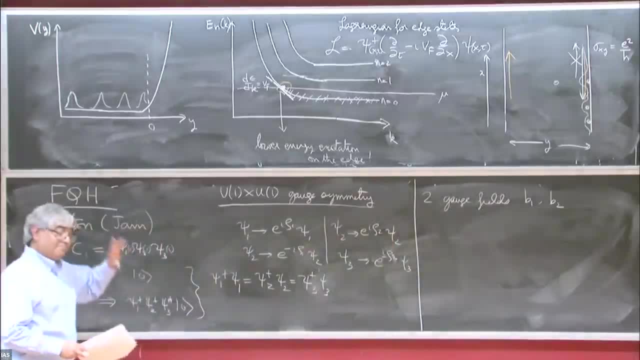 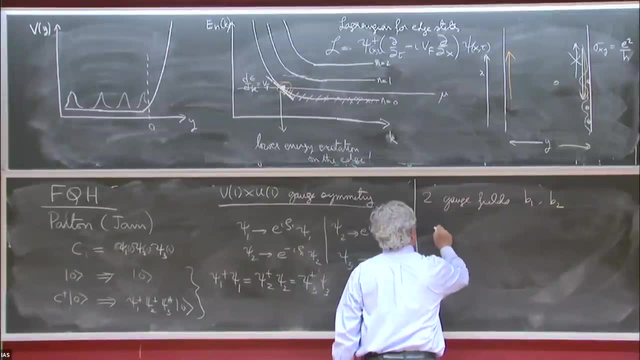 That's unfortunate notation, but small B will refer to gauge field and big B will refer to magnetic fields. Okay, so what would the theory look like? So you would have let me you know. let me write down the spatial terms. 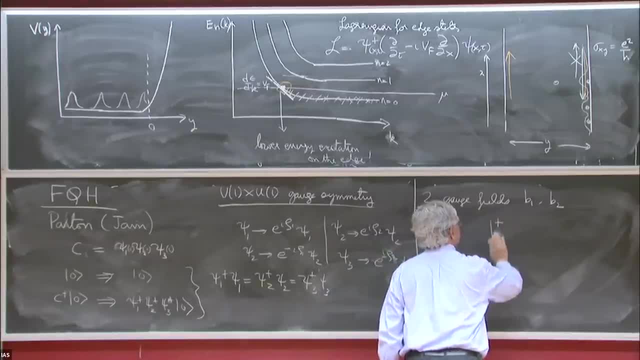 the most important one. So we'll have B dagger one B dagger, two B dagger, three B dagger, four B dagger, five B dagger, six B dagger, seven B. it should be appearing on the play- О sorry, XI dagger one over sweep coefficient than grad minus. 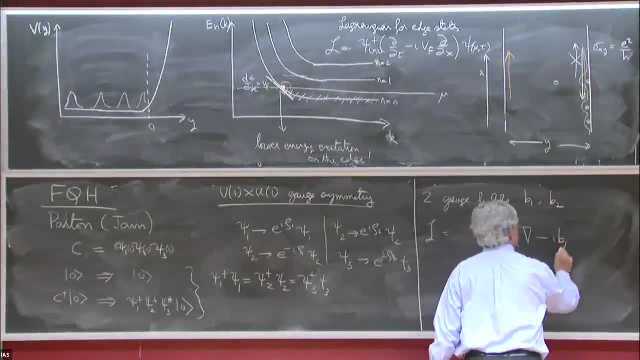 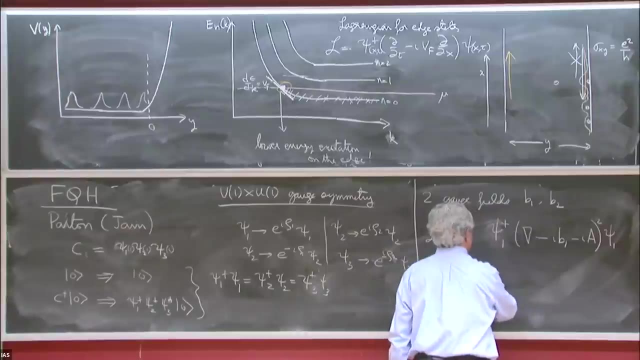 so si one has a charge Minus IV one, And let's put the external field to act fully on si one. It's up to you where it acts, but let's put it on si one, and then I'll have Heaven XI under two. 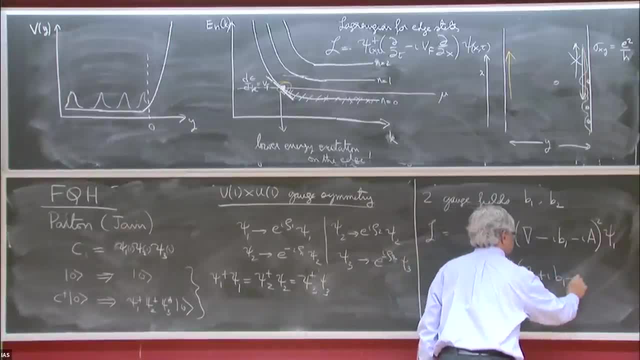 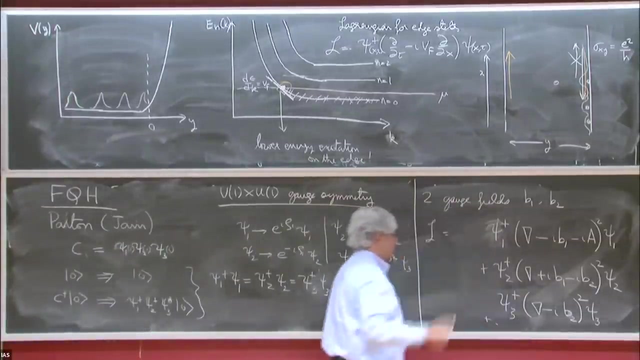 of rad plus i b1, minus i b2 minus i2 and I have psi dagger 3 of rad minus i b2 of psi 3. And various other terms, and really, since we're not trying to do a microscopic theory, we're not going to try to write that down, just the statement is: whatever you write down. 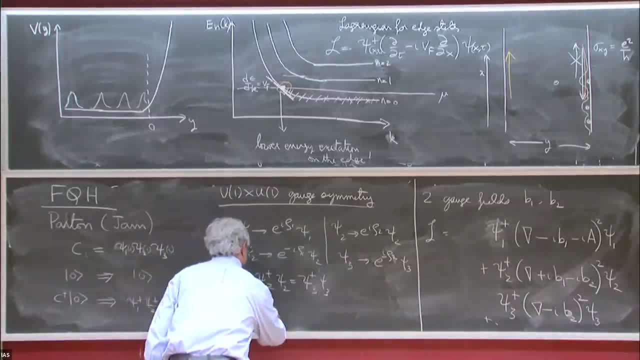 it's invariant under these gauge transformations and of course the gauge transformation b1 goes to b1, and I want to get the sign right- minus, I guess, minus grad of rho 1, and b2 goes to b2 minus grad of rho 2.. So you have these. 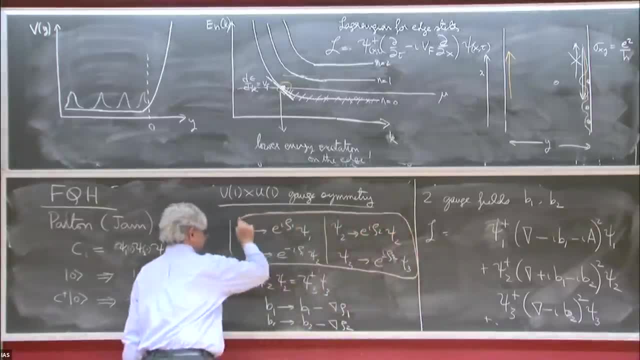 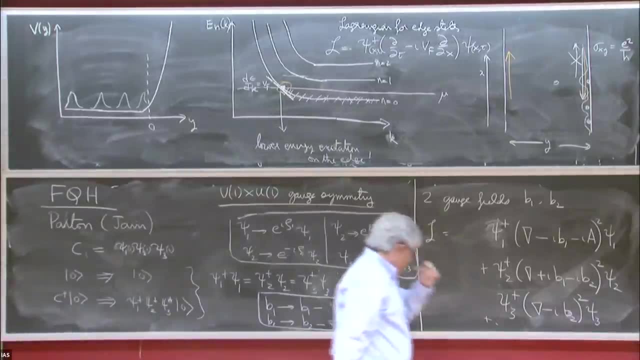 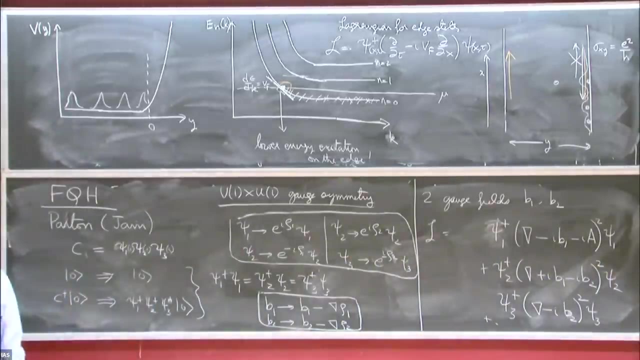 gauge invariances here and this gauge invariance here and you just write down all possible terms consistent with these gauge transformations. So what you're saying is: no matter how much how I distribute the real charge among those three sides, you can reabsorb it. 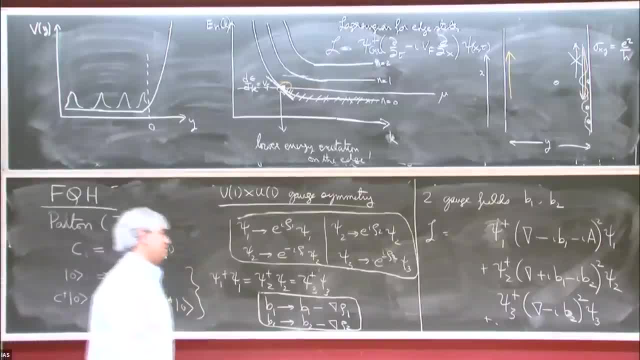 into the b fields. Correct That you can redefine your b1 and b2 so that you can put the charge in where you want. Yeah, so I just chose to put it there. Okay, Yeah, You can put. I don't want to take fractions. well, because these are compact gauge fields in some 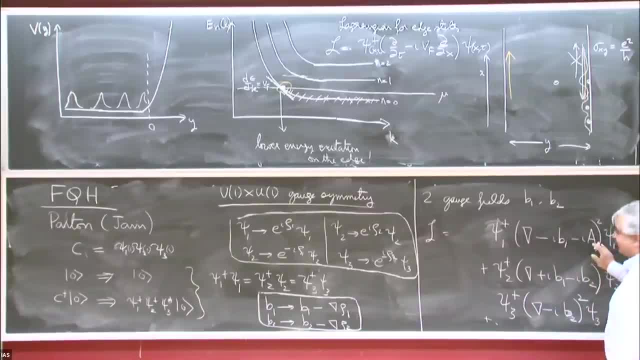 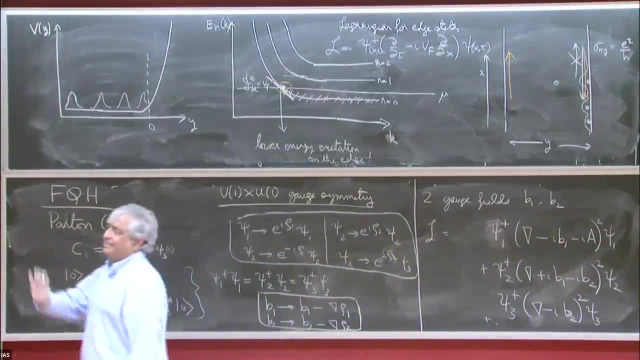 cases. that's important. so you don't want to put factors of two. but with the external gauge field you could take fractions, but even that's a little uncomfortable. So if you don't want to put a over three, a over three, a over three, then you have to keep track of, you know, the flux quantum. let's. 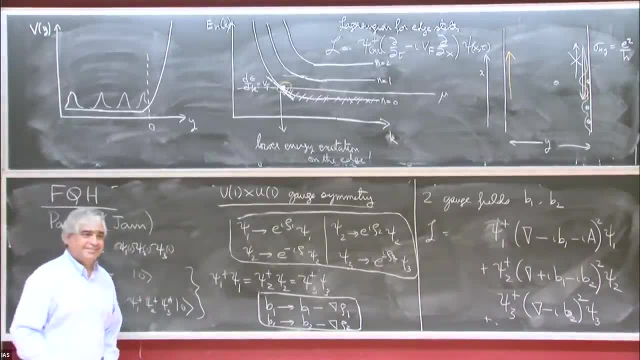 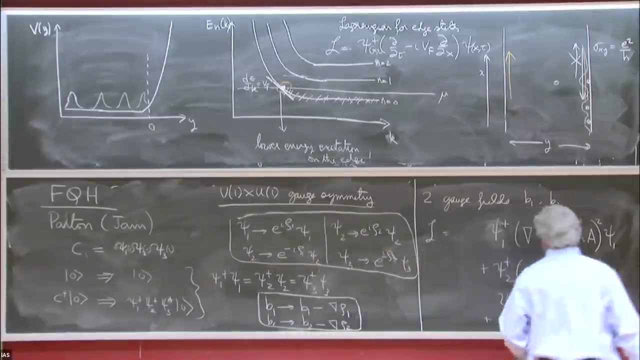 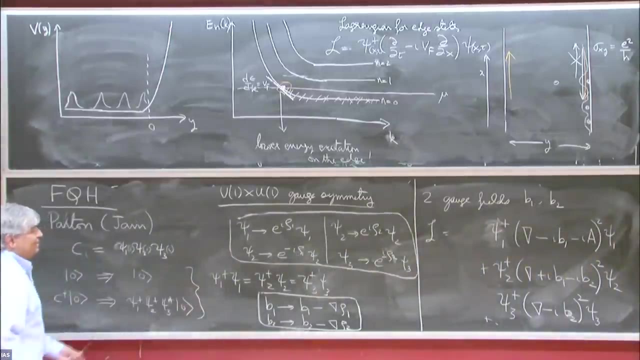 become a little more careful, So it's better to put it in one place. Okay, um, all right, so this is our theory, or this is just a general theory of electrons in any dimension. so far I haven't made any uh, any uh, any particular uh specialization. 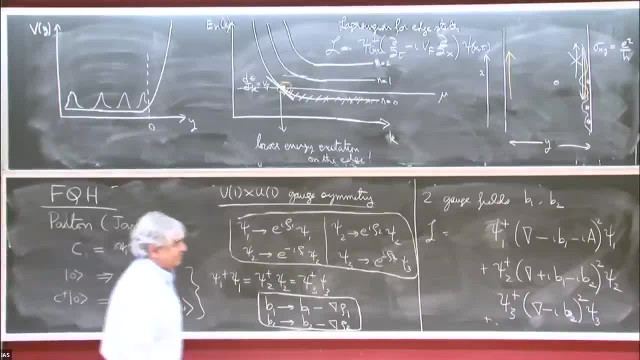 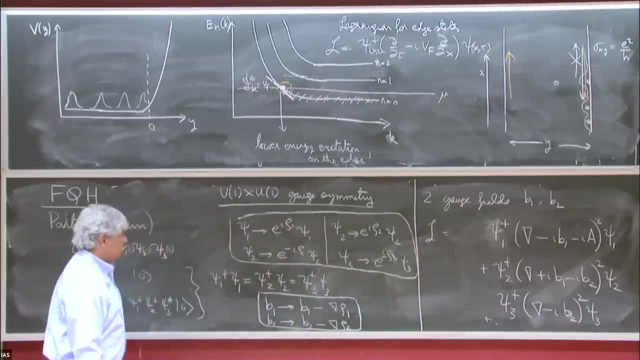 you could do this, if you know, whenever. you could always do this for any system, uh, but of course, the question is: when is this a useful thing to do? um, when is this particular fractionization something that's likely to happen? and I suppose that's probably why the parton method has been. 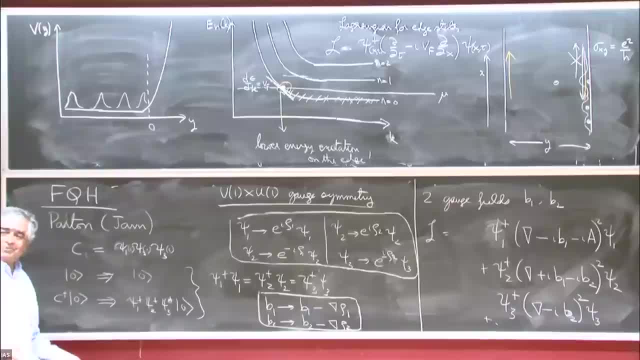 used as much. it's very powerful but it doesn't tell you when it's good to use it. Other methods are numerical methods, you know, somehow motivated from particular Hamiltonian. but once others have motivated or experiments have seen a certain state, you can just go ahead and figure out what's the 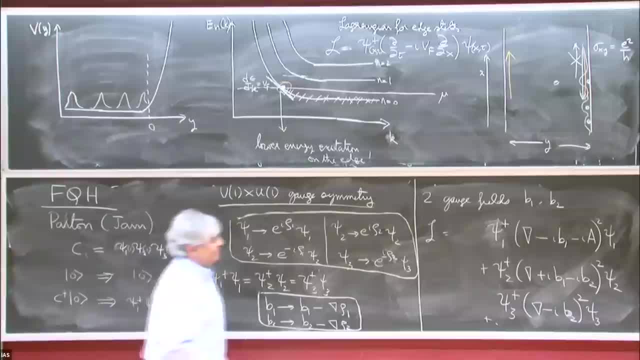 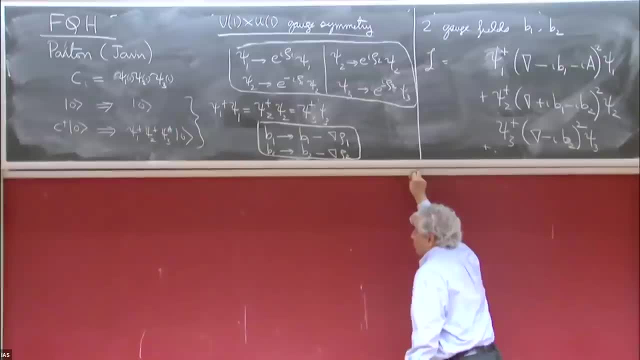 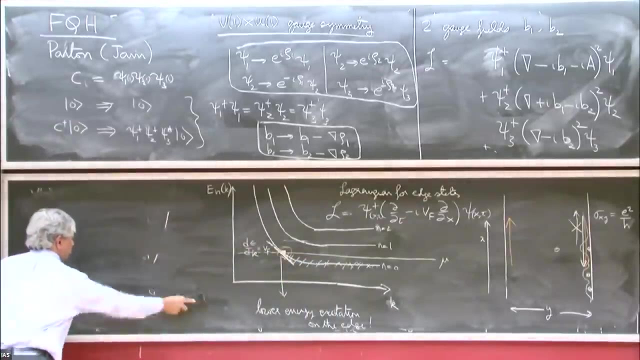 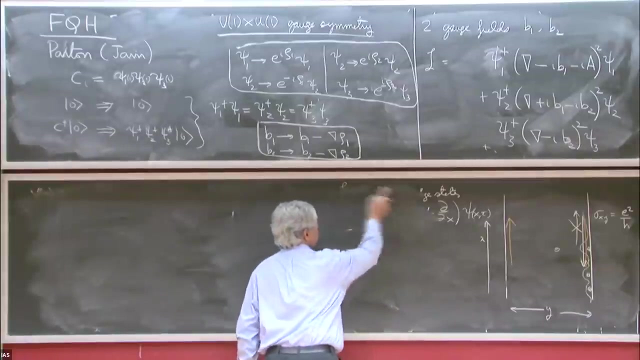 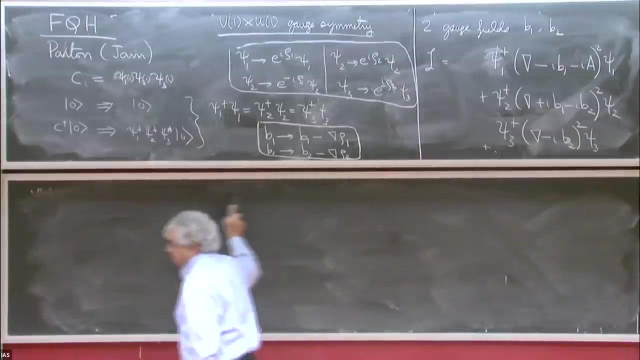 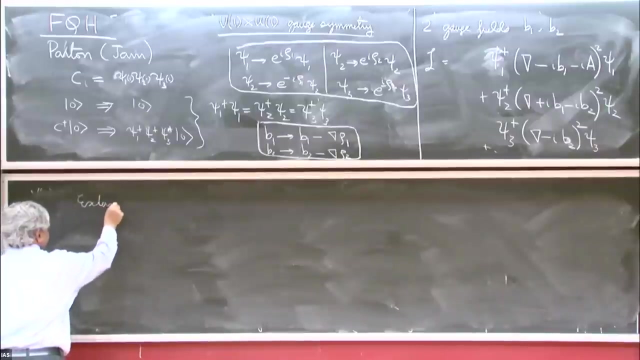 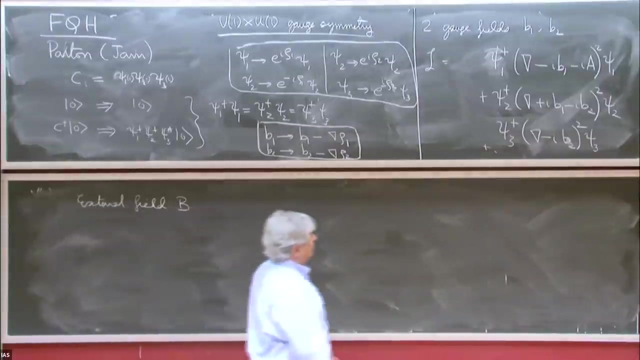 right part on description that will give me that state. So so why do we use it? so we want to use this in the following situation: so we have an external, so we're going to be in two dimensions. we have an external field b and. uh, I'm sorry, the electric charge has gone, it goes off. 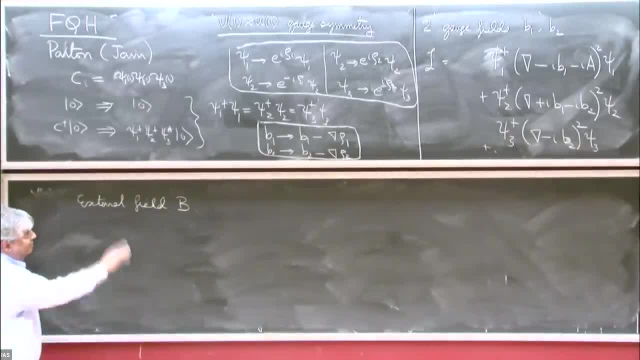 okay, that's for simplicity. uh, and now these protons are going to experience their own magnetic field. so the magnetic field on on psi one will be, I'll call it b1, and b1 will be, you know, del cross a plus del cross b1. and parton two will experience the field b2. um, which will be del cross a. uh, sorry, 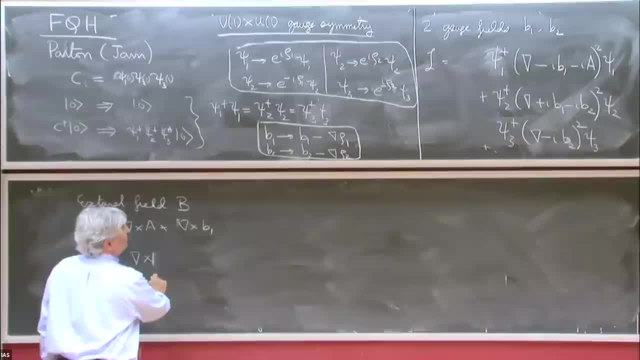 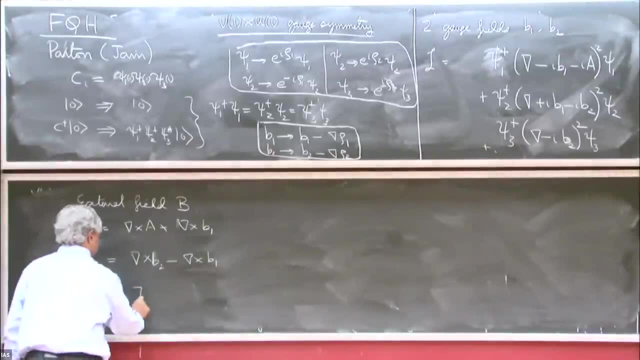 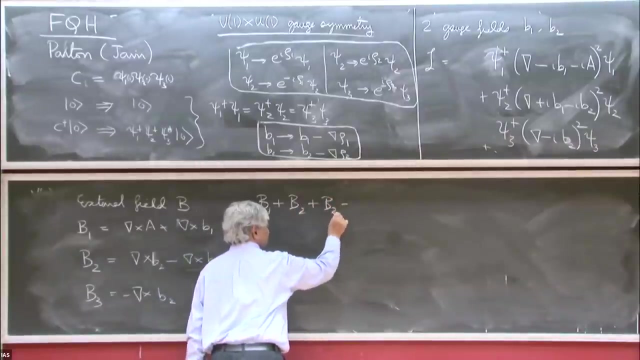 del cross b1, b2 minus del cross, b1 and b3 will be uh del cross minus del cross, b2. and of course now you should check that uh, b1, b1 plus b2 is b3. the next field, uh, is equal to the external field. 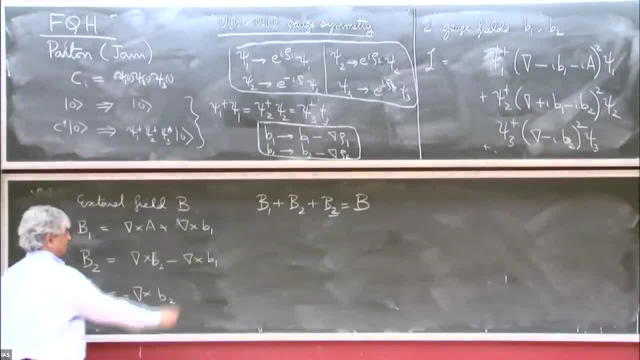 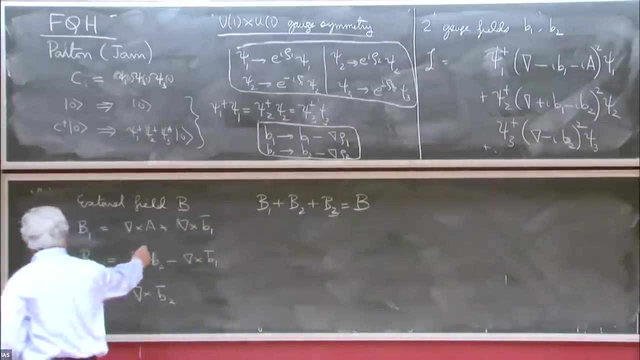 so each of the protons experience the next field. and just I'll put a bar here, because we're going to imagine that these gauge fields have a non-zero expectation value on the saddle point. these are fluctuating fields here. this is their average value. okay, okay. 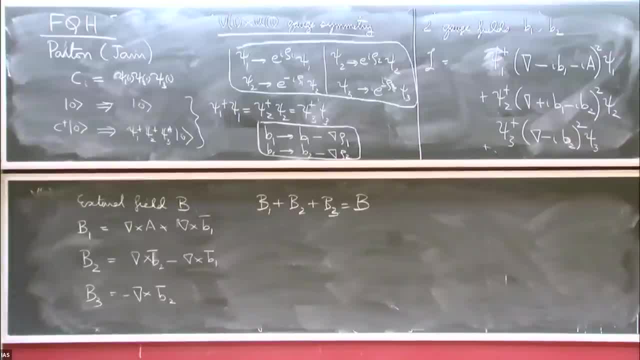 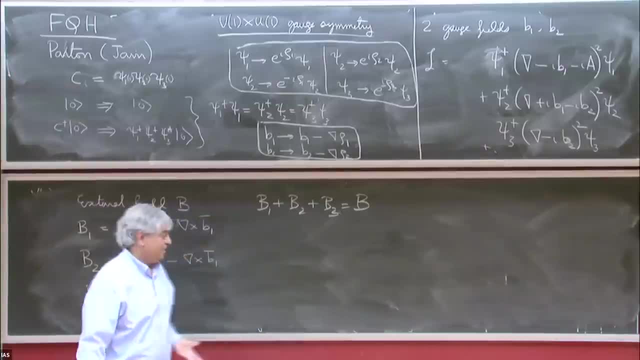 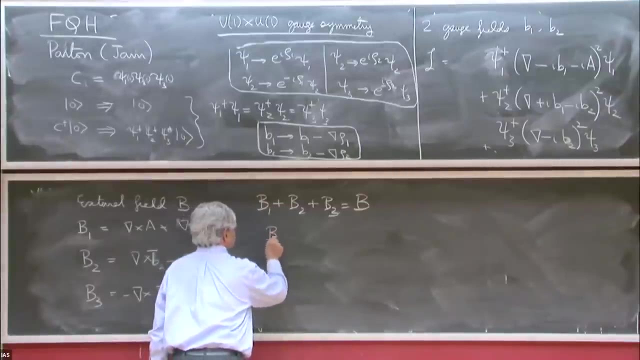 so when should this be useful? well, when it's useful is if the parton fluctuations are are weak, and so well with the parton fluctuations will be well if, if there's a gap to the proton excitation, so in a magnetic field, uh. so what we require is b1, b2, b3, uh, such that 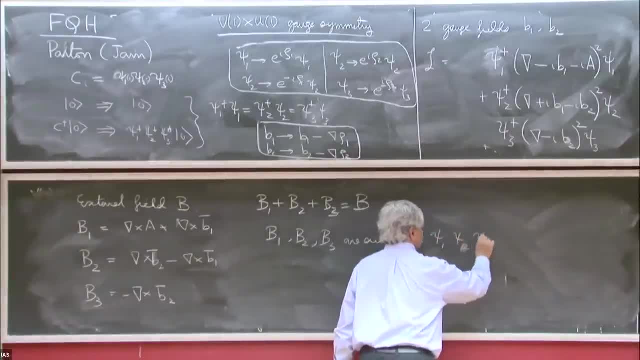 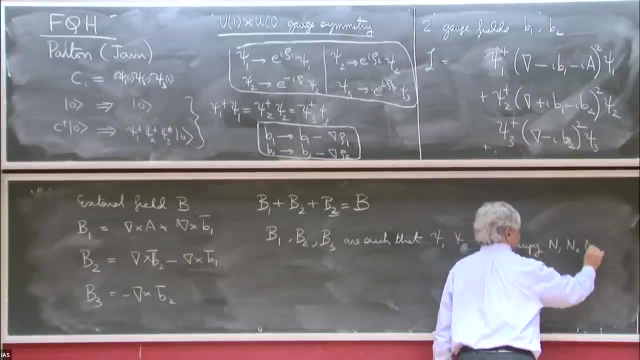 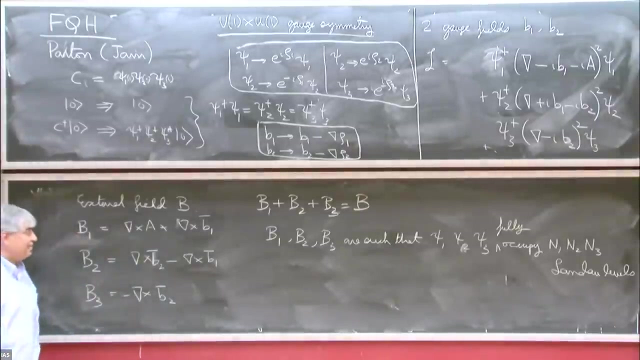 psi 1, psi 2, psi 3 occupy n1 and 2 and 3 landau levels. they fully occupy their own landau levels and then you'll have a gap. so then there's a gap to all the excitations of psi 1, psi 2, psi 3. 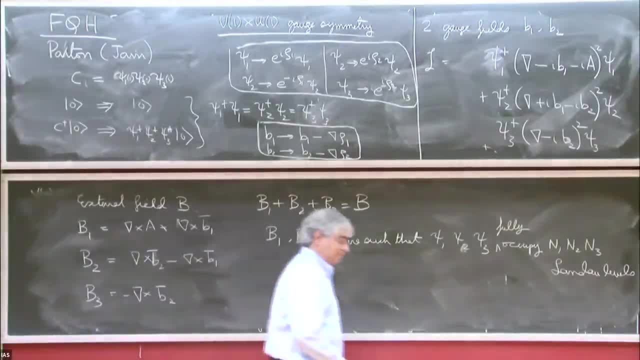 and there's a hope that this very drastic decomposition is like stable. there's no gapless excitation. anyway, you may have to worry about other things, but this is a good starting point. so what is this? so what does this imply? so now let me make sure I get this right. 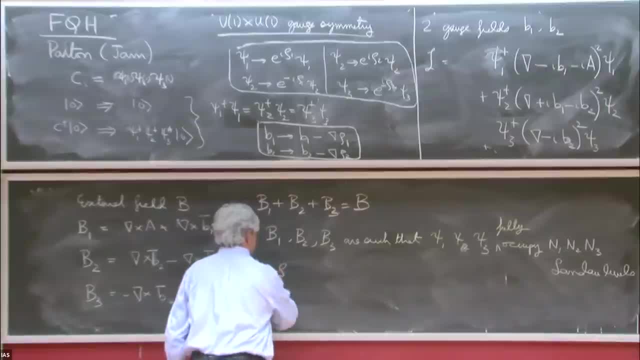 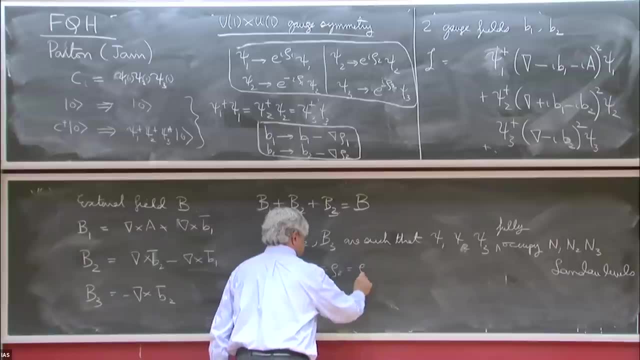 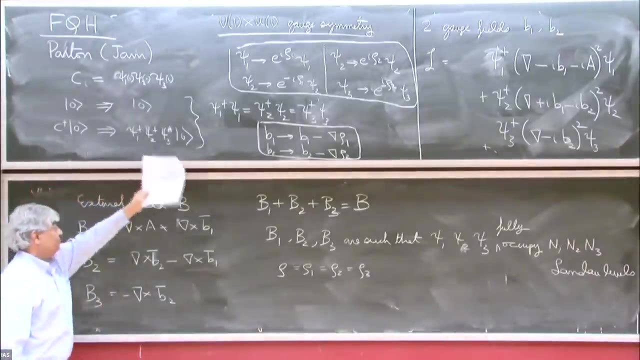 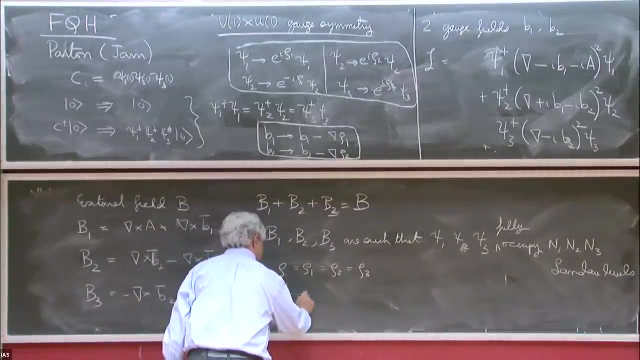 uh, the density of the electrons is the same as the density of all. three of them have the same density because of the constraint. this constraint right here. the density of the electrons is the same against the psi 1, psi 2, psi 3, So the filling fractions of each of them, so one over nu, is equal to where did it go? 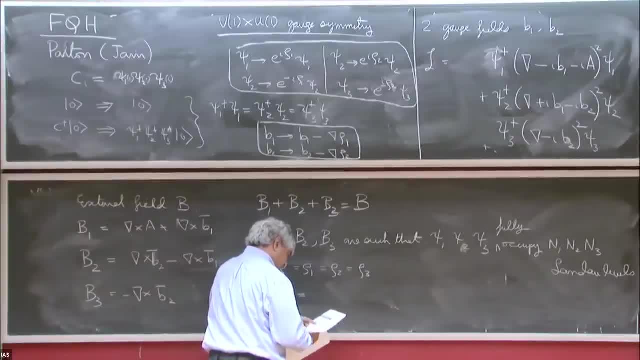 That's the magnetic field. what is it? That's the density. rho one. so rho over B, over phi naught. that's the filling fraction of this Filling fraction of the first fermion, which now is going to be n, it's going to be an integer. 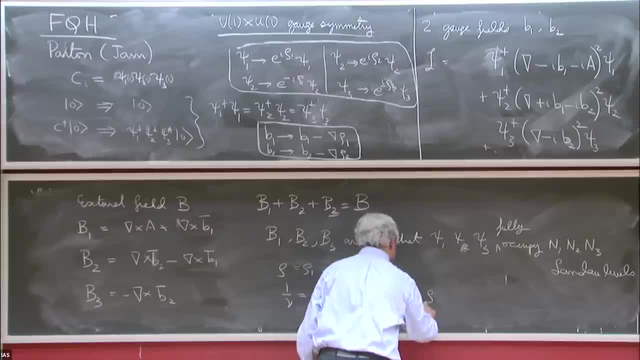 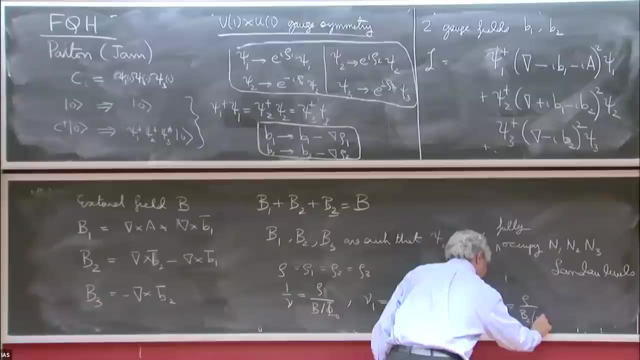 is rho, which is the same as rho, one over B, one over phi naught, and so on. Nu two will be an integer and two which will be rho over B, two over phi naught, and similarly two goes to three. 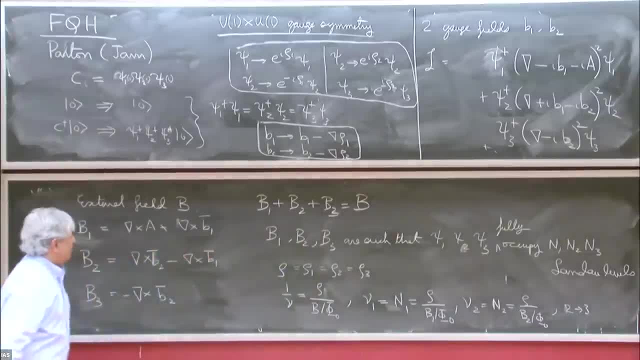 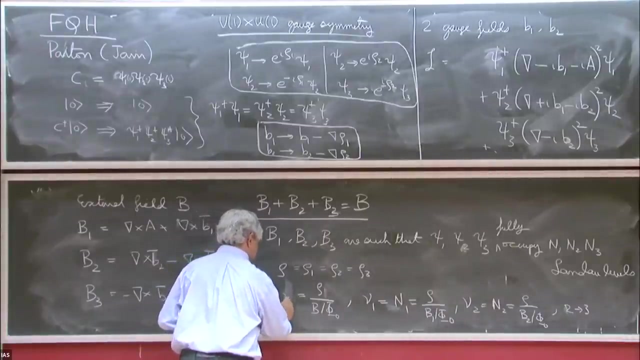 Okay, so I have this equation here, I have these equations here and you combine them and you get a very simple expression. Sorry, The first one is nu. Oh, thank you, This is nu. Yeah, Does flux. quanta are all the same. 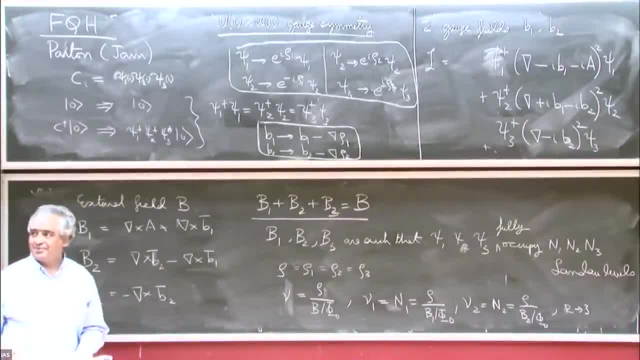 Oh yes, E is one, Yeah, and H is one. Flux quanta is H over E, and I put time equals one. So there may be factors of E that you have to carry through, but okay, E is one. You can always measure B one in units of E. 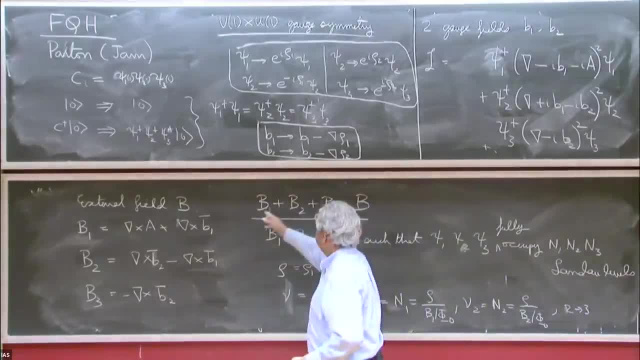 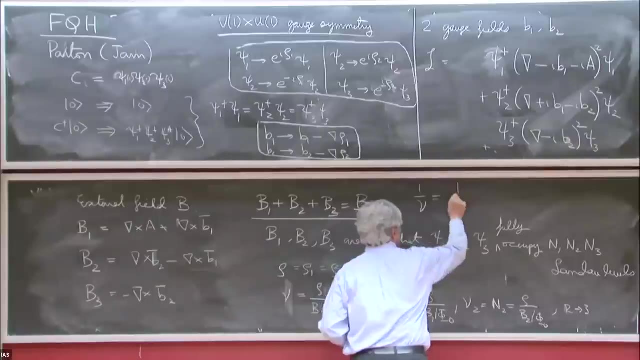 Okay, Yeah, which is obviously what we're doing here too. So we put: E equals one, All right. so if you combine all these relations, you get a very elegant looking relation for the filling fraction of the electrons, which is one over nu. 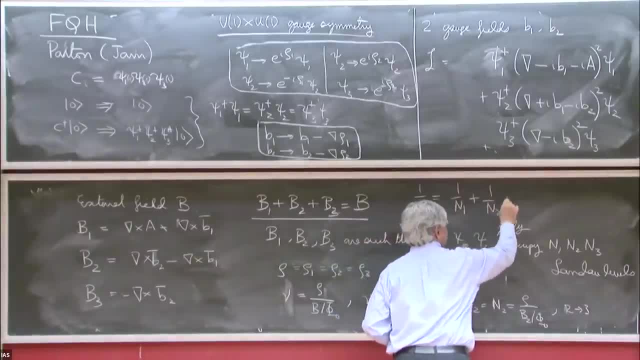 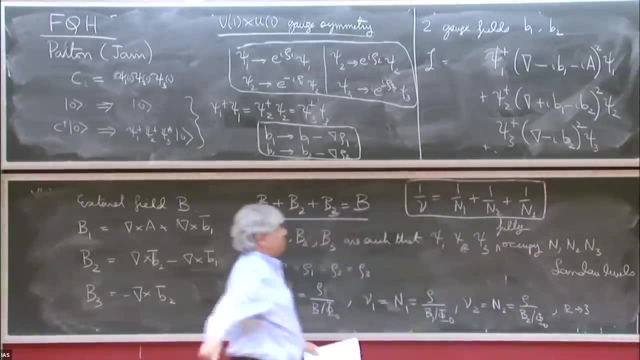 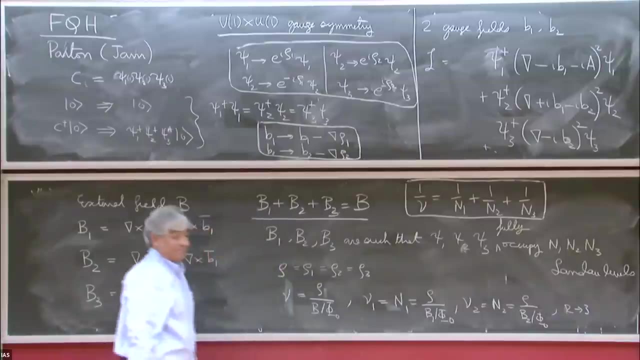 is one over N one, one over N two, that's one over N two. So for this three-part construction to work, N one, N two, N three are positive integers. In fact they can even be negative. You can put the field in the other direction. 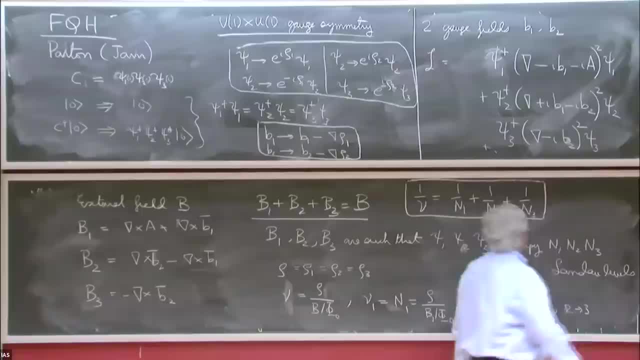 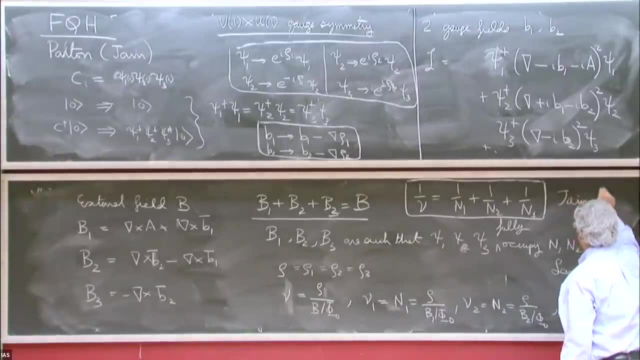 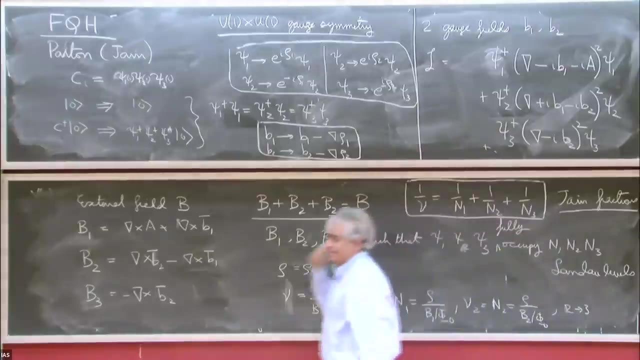 We won't consider that. Then this is the special filling fractions, And these are, you know, special case of what I call the J-interactions, And in fact essentially all of those states are of this type. Okay, All right. 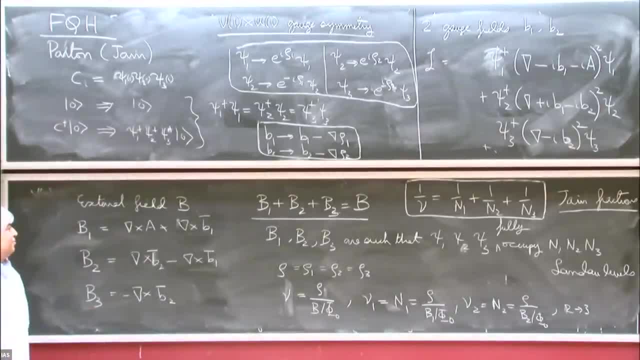 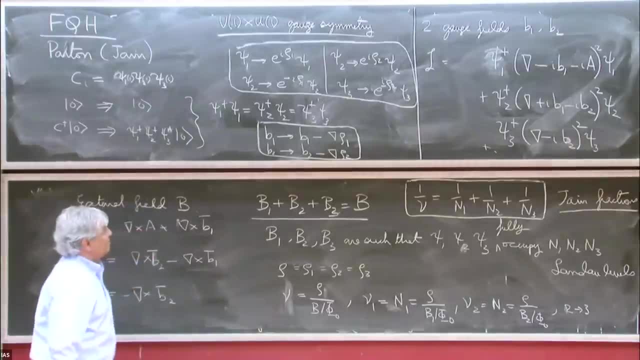 All right, So that's it. So now we have a saddle point which has a gap, Then we can do all kinds of fluctuations about it And you know, you'll get Chern-Simons theory, edge states. But we've done enough of all of that. 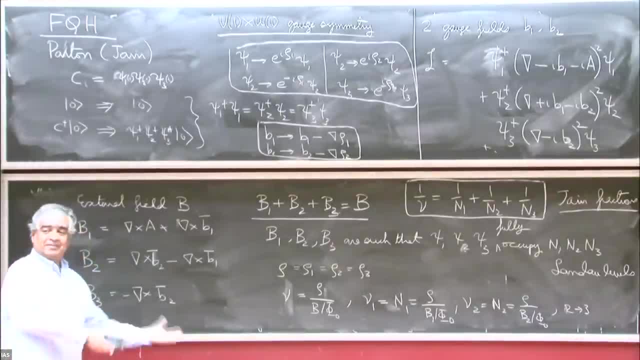 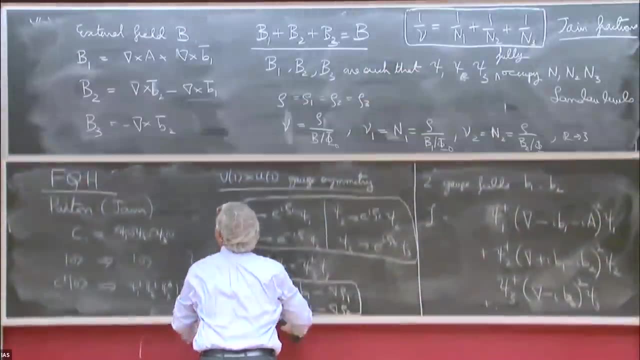 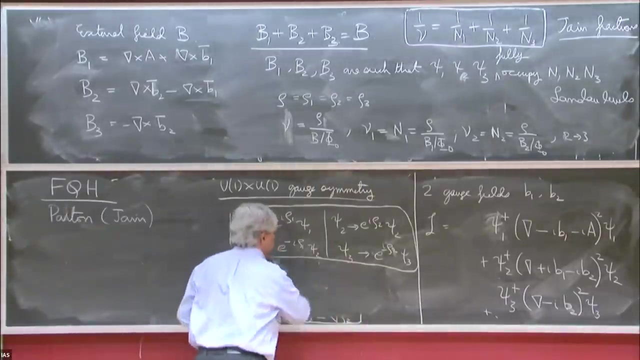 In fact, the whole analysis would be identical to things we've already talked about, Just the different cases of that. Okay, So what's the simplest case? The simplest case is N. one equals one, equals two equals three, So all of them equal to one. 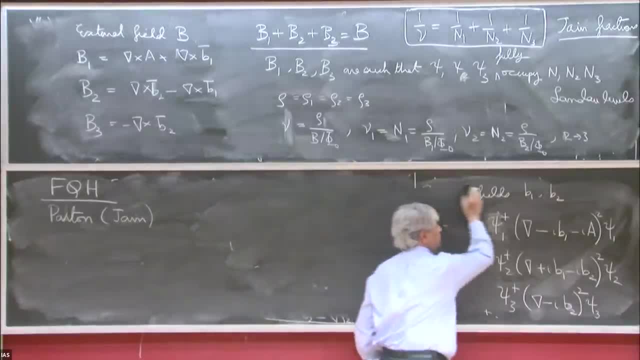 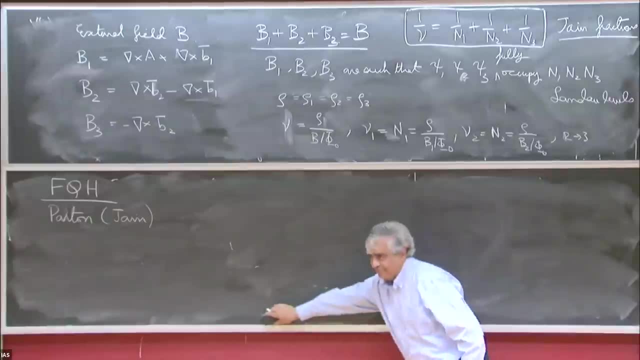 Is there a simple formula for the Chern-Simons levels in terms of these integers that you use? Yes, But I'm not good at it, So it's a bit of a mess. I think I've only done one. It's not a special case. 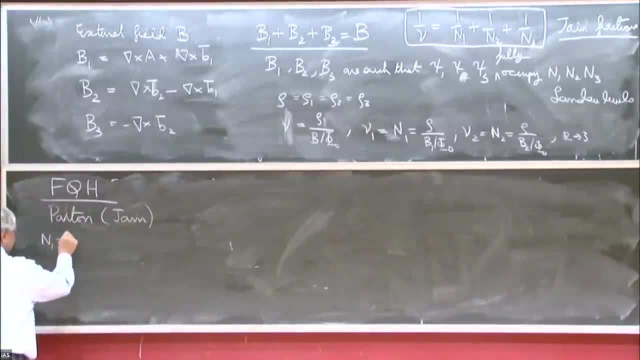 So we're going to look at the case First of all. the most important case is N. one equals one equals N, two equals N, three equals one When, of course, nu is one third. That's the famous Laughlin state. And now, to go back to the beginning of the lecture, I can write down the wave function of this state. 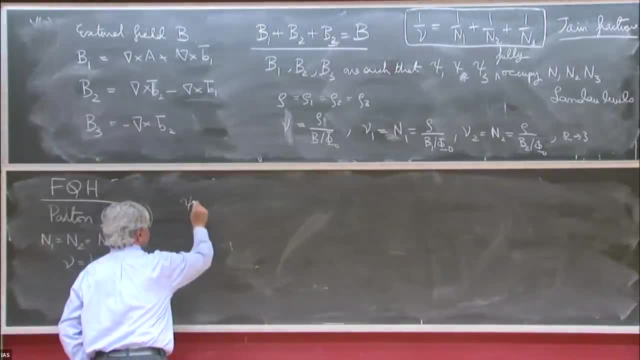 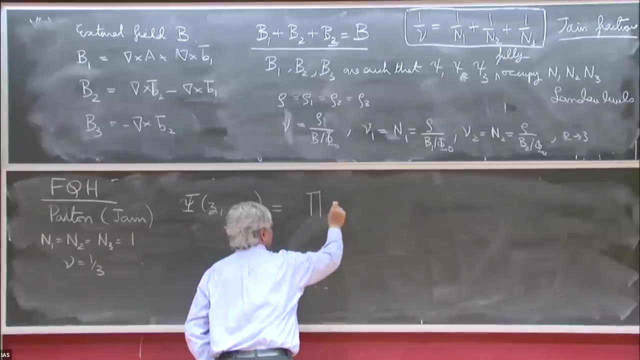 So the wave function of the electrons. So this is the capital psi Of z one to z n. It's a product of three wave functions. It's the product of, let me say, wave function of psi one, And this will have some coordinates. 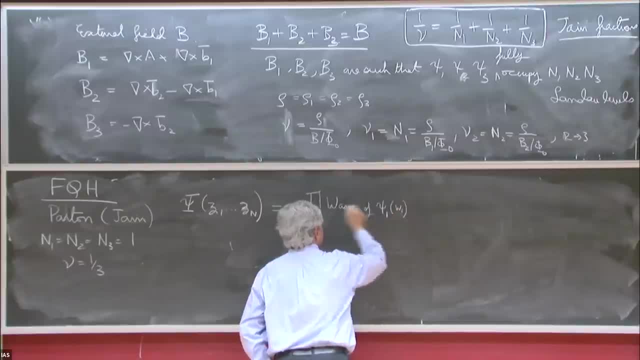 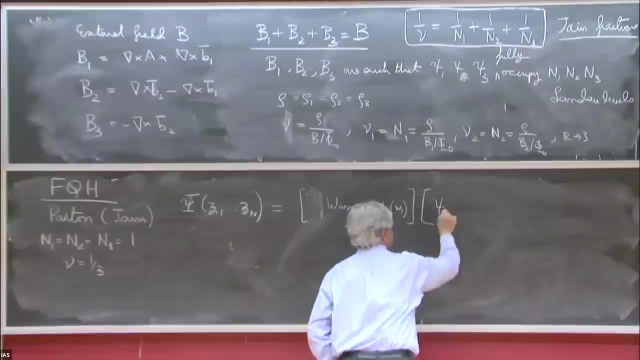 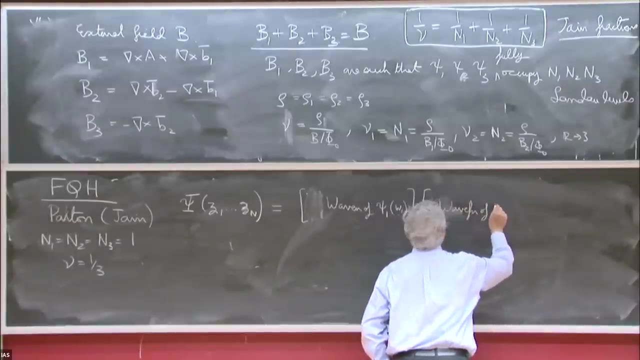 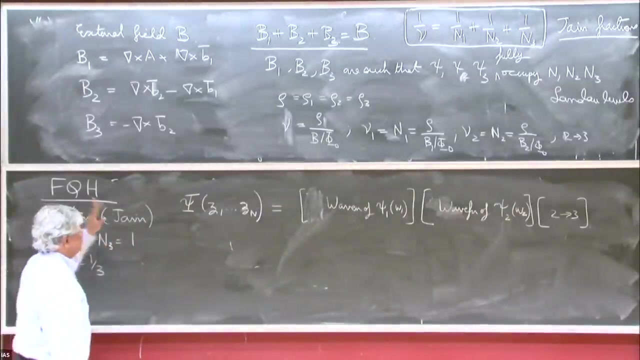 Let me call them w one, Similarly for the other ones, But the product is outside The function Of the field. psi two With coordinates, w two And two goes to three. Okay, Now, what are these wave functions? Well, these wave functions, we already know that there was a single Landau level. 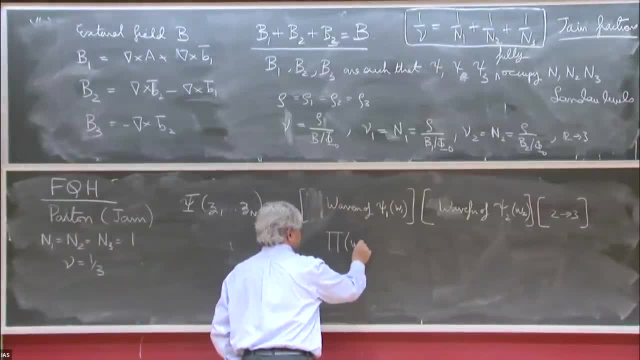 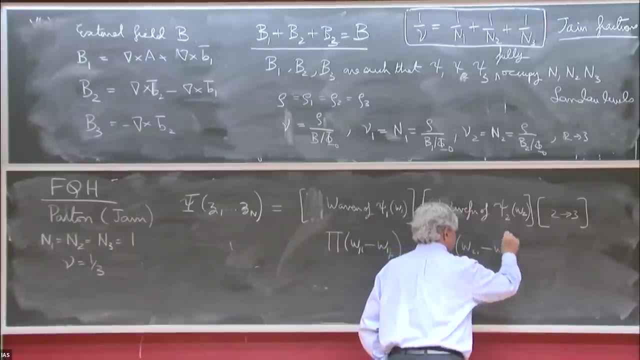 So this is product of w one i minus w j. Let me not worry about these. W one i minus w one j, And this will be product on w two i minus w two j, And this will be product of w three i minus w three j. 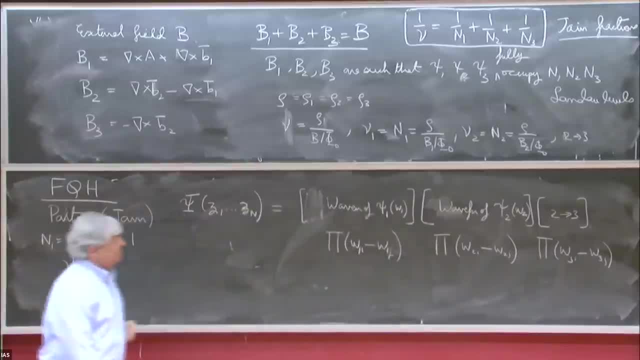 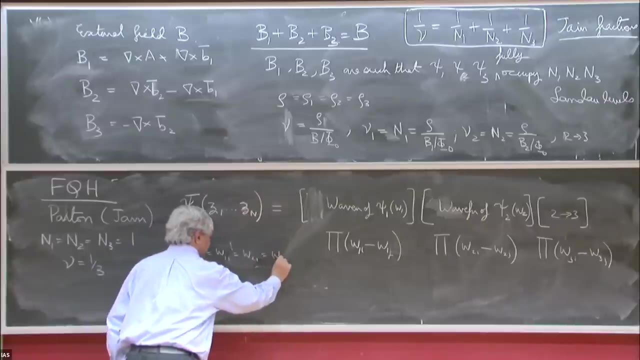 This is the fully filled Landau levels, The vector-borne determinant. And then you have a constraint that the densities are the same. So we have the constraint that z? i equals w one, j, Z i equals w one, i equals w two, i equals w three, i. 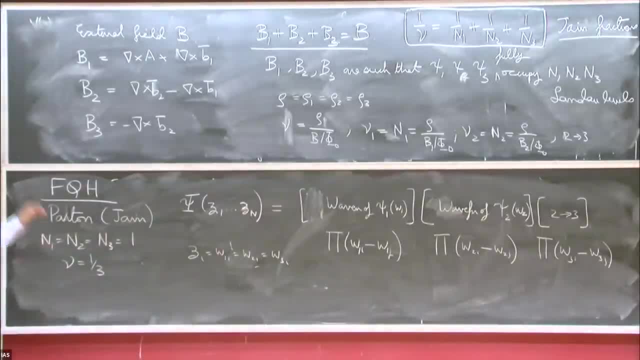 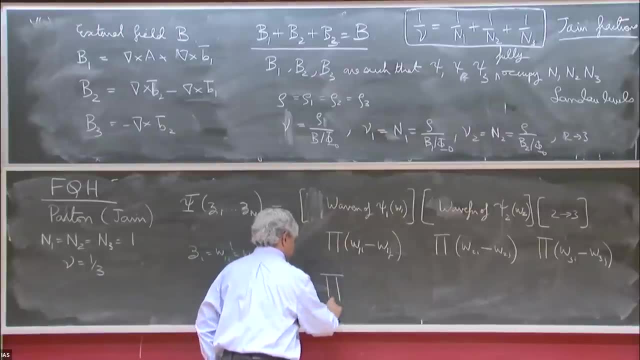 That's the original constraint that you had. Then we started out the part on construction And of course, then this is the famous Landau-Loughlin wave function, And I'll leave off the exponential factor. You could satisfy the constraint with extra phase factors. 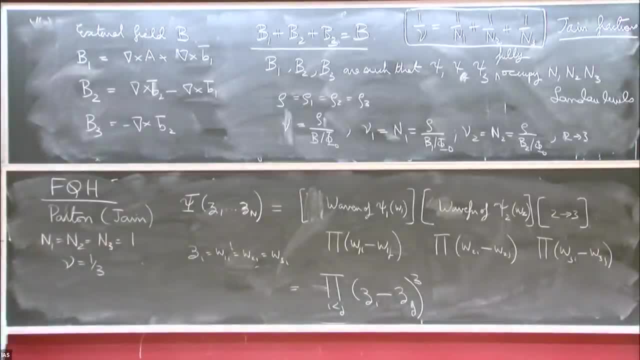 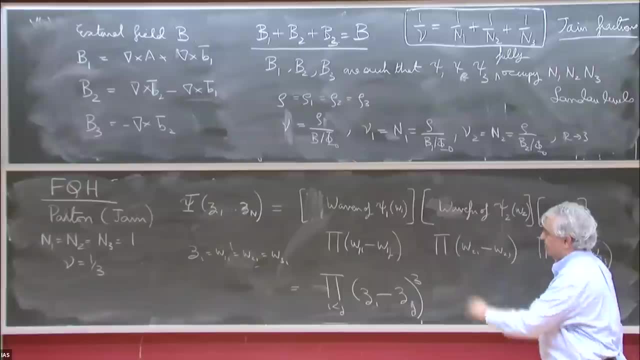 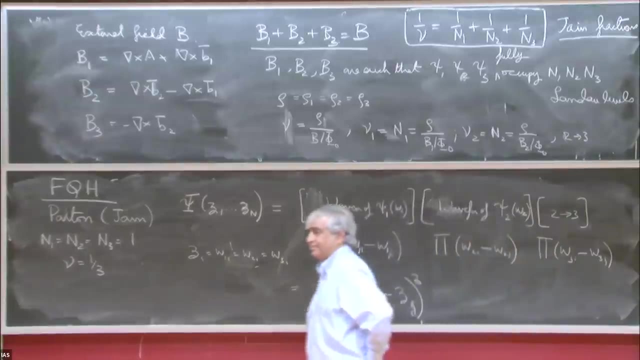 Okay, All right. Well, these are the coordinates. The position of the particles, wherever they are, have to be the same, But the real constraint is that the densities are the same. If you apply that at every point, then the coordinates- the first point does represent the coordinates of the particles- have to be the same. 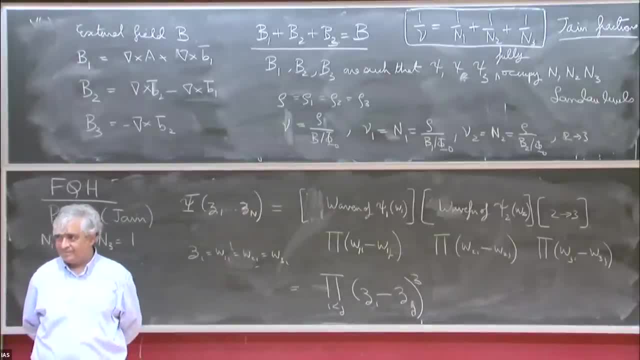 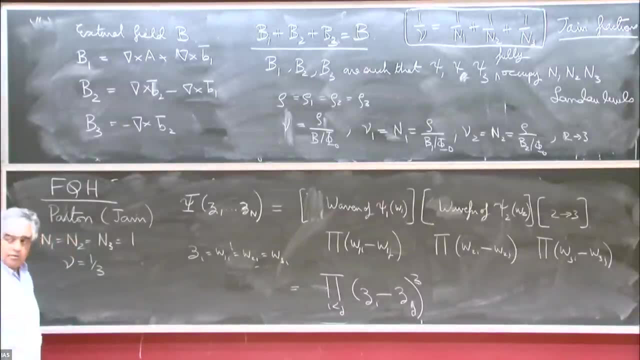 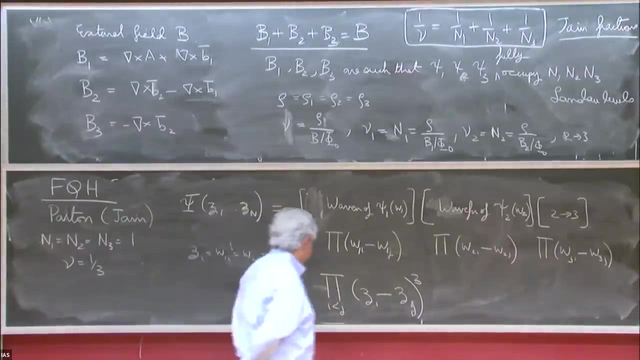 I'm kind of going back and forth with the second point. I'm just saying the individual wave functions could have factors that would disappear when you enter the density Mm-hmm. Okay. Okay, I'm not sure which factors you're referring to. 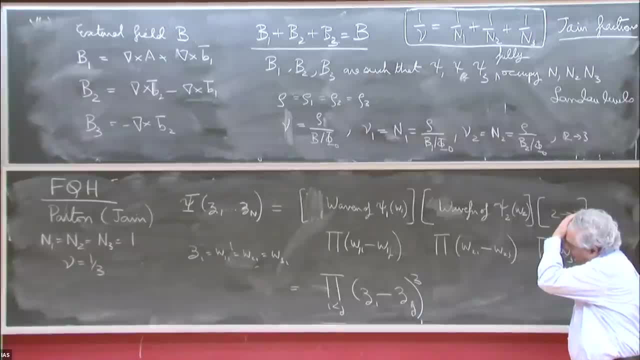 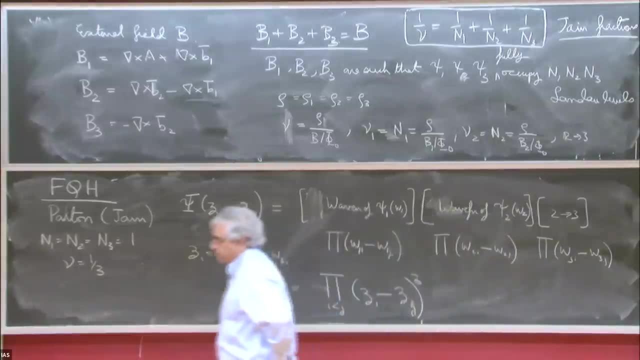 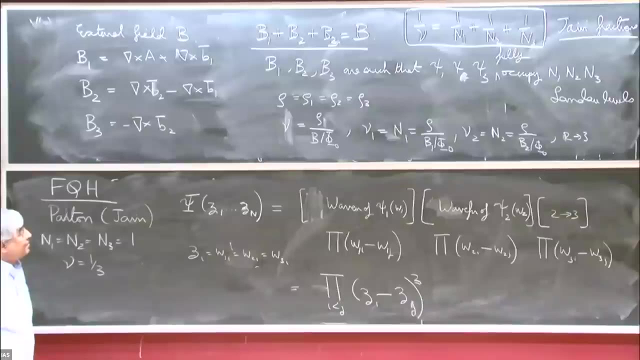 Some things that appear up here. I think this is fine. I don't think there's any arbitrary less here. Okay, Yeah, Okay. So that's of course, the Loughlin wave function that started this whole analysis, And then later on, Jane pointed out that in fact, 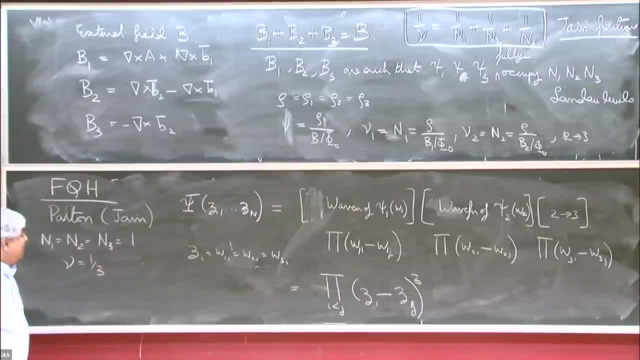 this is one very simple way to do it, This is a simple way to think about it. But then the power of Jane's approach. And so, after Loughlin's wave function, there was a very complicated theory- I should say, at least complicated for me- of what's called the hierarchy. 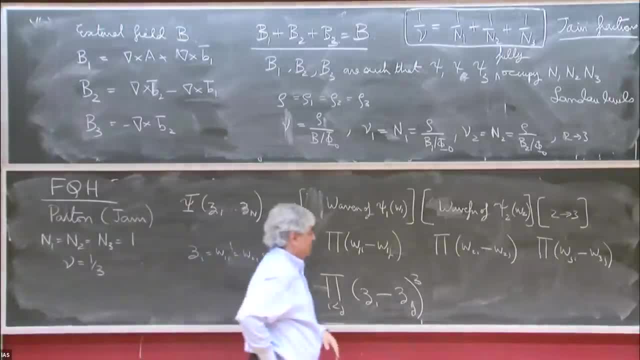 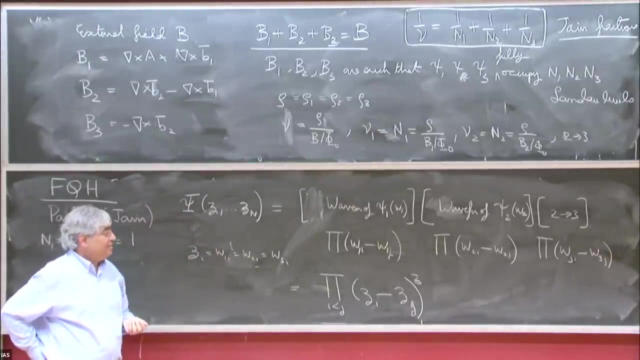 Because the experiments showed many other fractions, And so people developed a hierarchy, And the basic idea of the hierarchy was: well, you have the Loughlin state and it has certain quasi-particles which have fractional statistics Very similar to the chiral spin liquid. 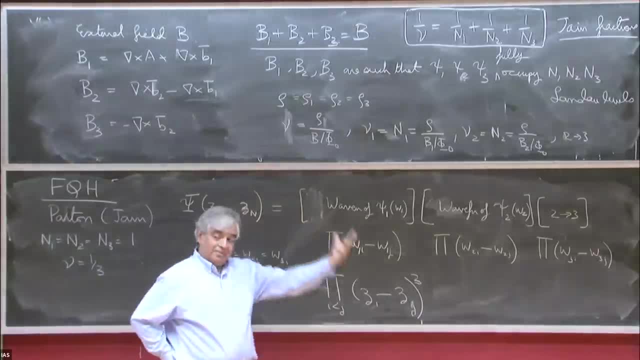 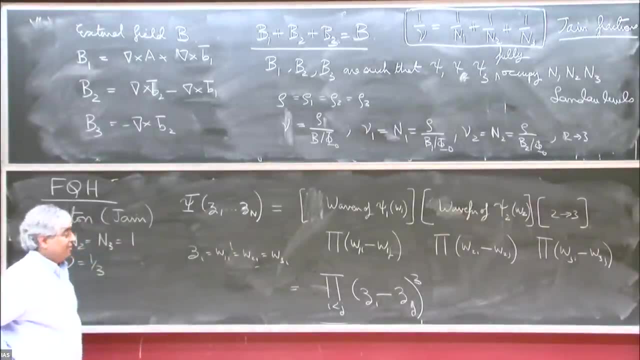 And then those fractional statistic particles can form states of their own Fractional point of hold states and other densities. So you get a finite density of quasi-particles about the Loughlin state and then you get a hierarchy. But the hierarchy, there's nothing wrong with it. 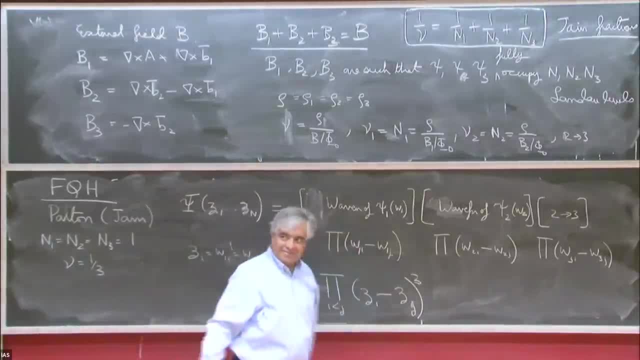 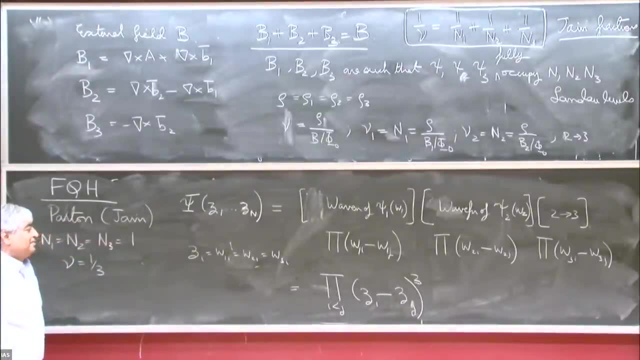 But it predicts all kinds of fractions, only a small fraction of which are actually seen. And also there's the question that the hierarchy assumes- you know, the whole structure of the hierarchy, at least initially assumes- that the quasi-particles are dilute. 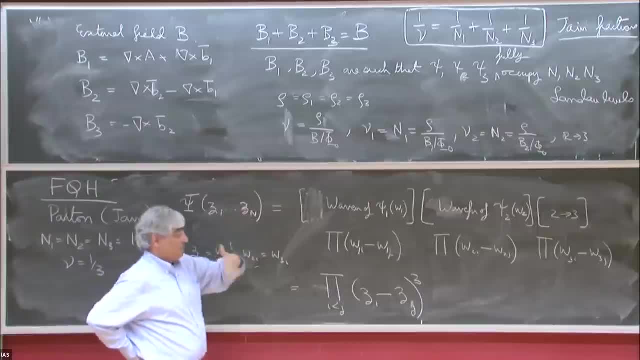 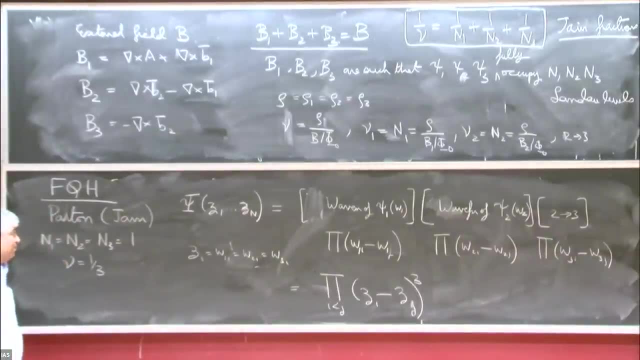 But to get the higher states and the hierarchy, you're making them quite dense. So should you really believe it? At least qualitatively you could, But quantitatively it may not be the right way to think about it, Anyway. so what Jane showed was that if you did this approach, 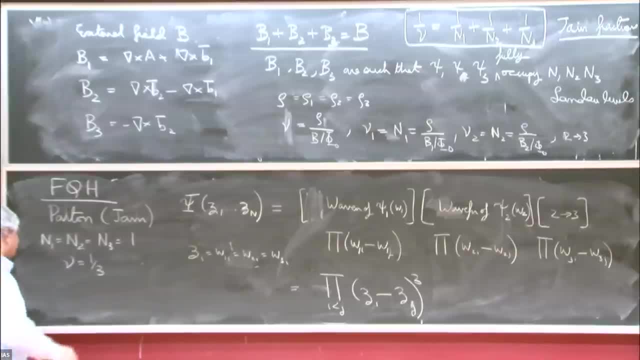 in fact, it was highly predictive in the sense that the most important fractions are the ones where you just take one of these integers and make them not equal to one. So, more precisely, the other important cases are: n1 equals 1, n2 equals 1, and n3 equals n greater than 1.. 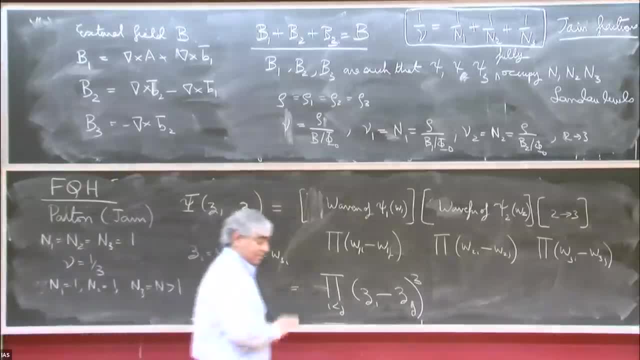 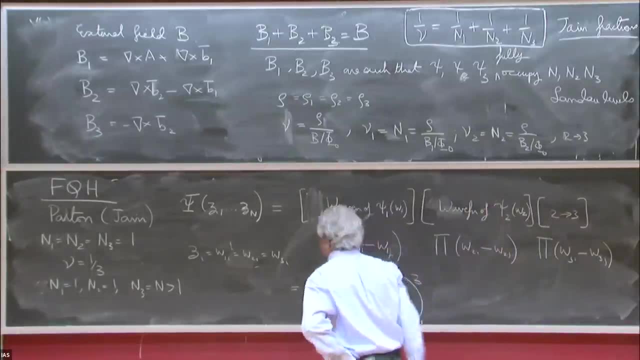 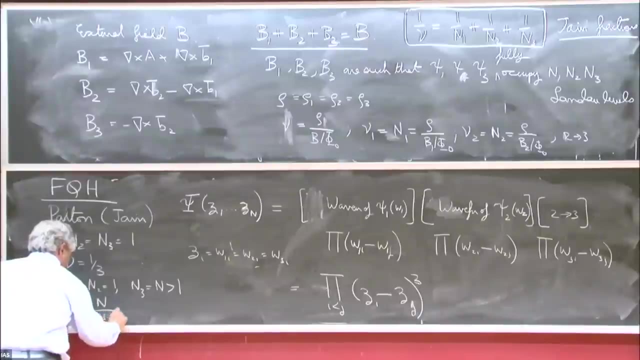 So you put two of the protons in the lowest Landau level and the others in some higher Landau level, Then if you take that famous expression and work it out, you get: nu is equal to n over 2n plus 1.. 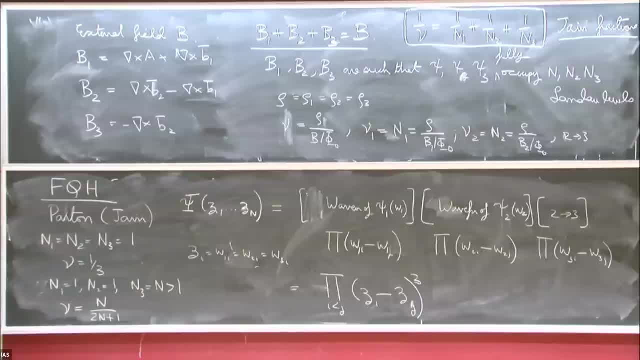 And these are by far the most important quantum model fractions. The next one will be n equals 2,, which will give you two fifths after one third and so on. OK, so much time I have, So probably I'll have to say a bit more next time. 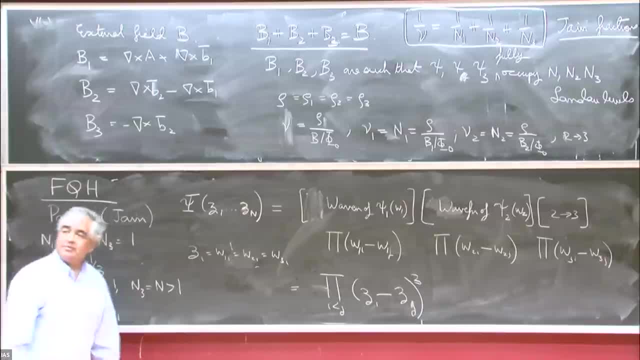 So now there's Intuit to get nu equals one fifth. Do we get the five cartons or do we get The one fifth? yes, five cartons, But that's a relatively hard fraction to see. It's pretty close to Wigner-Crystal. 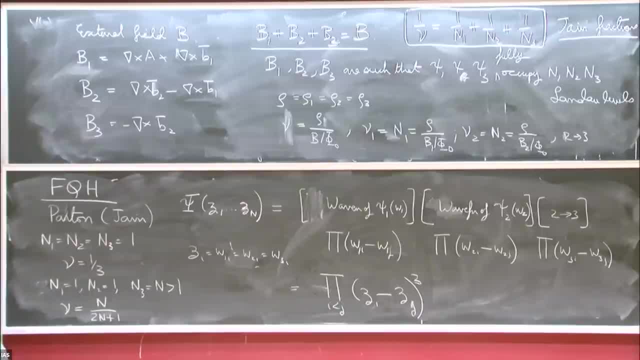 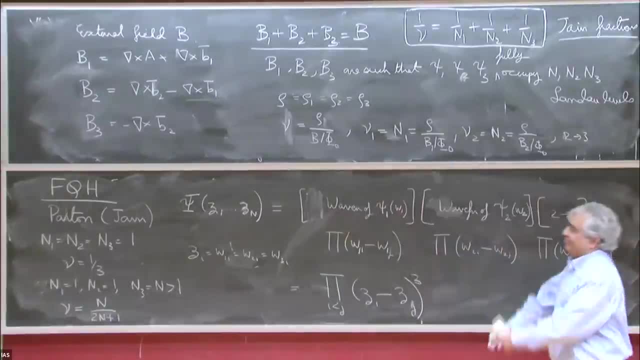 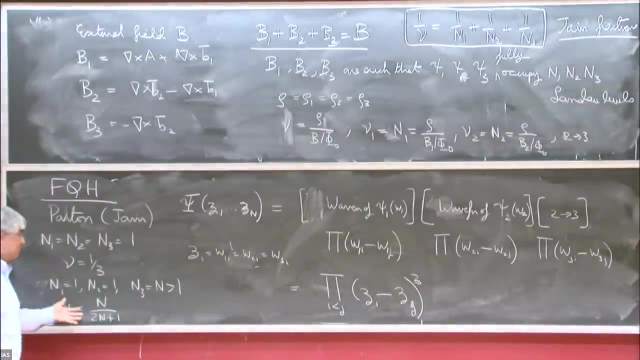 Most of the ones that you know, experiments that are wrong. nu equals one half, Yeah, Yeah, but in principle right. This also has its, you know, lateral possibilities. But what's nice is that the very simplest possibilities, the three, is the smallest thing you could do. 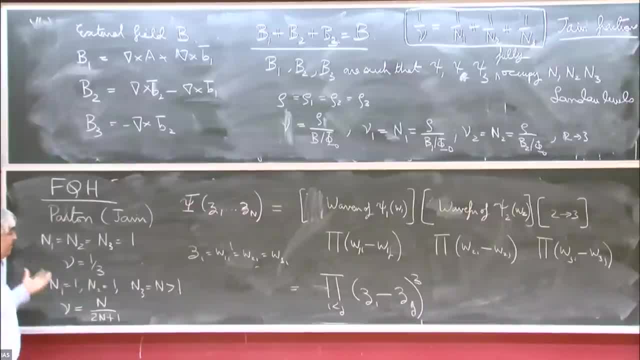 And you can't do, can't go to one, then there's nothing to do. Three is the smallest allowed number And you just make one of them greater than one. that's sufficient to give everything. So there's a certain economy here. 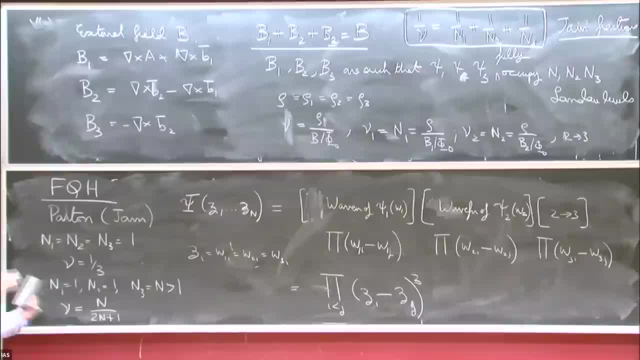 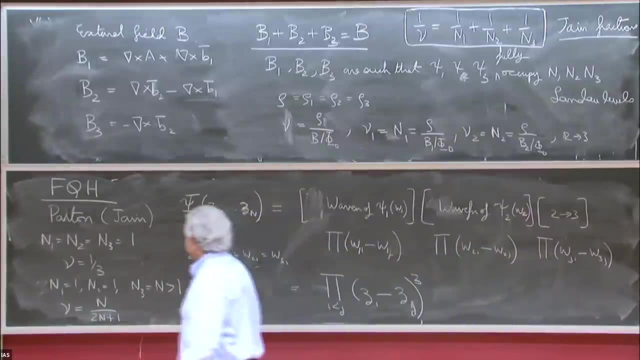 But of course it's in fact all of the states in the hierarchy can also be obtained by this approach. Yeah, Yeah, So I think we have 15 minutes. So what should I talk about? Okay, maybe I'll talk about edge states next time. 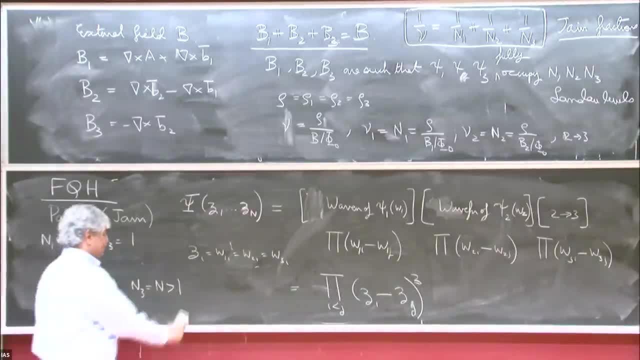 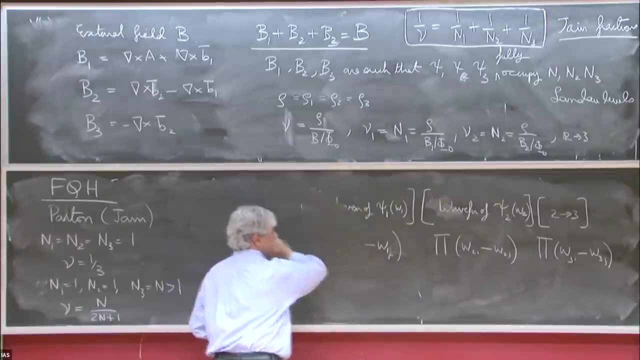 Let me talk about one very important case, but in a slightly different type of topology. So at this point you know if you've been following my lecture so far- you just have to turn the crank and do everything we did for the chiral spin liquid. 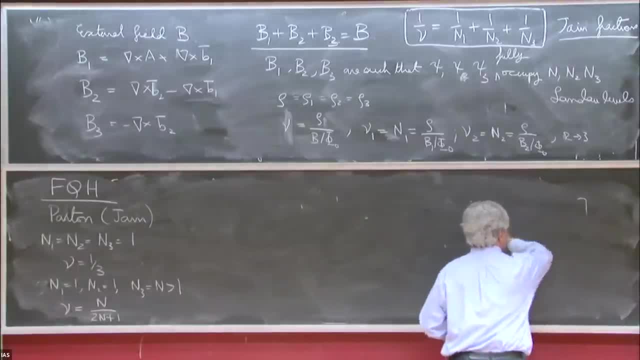 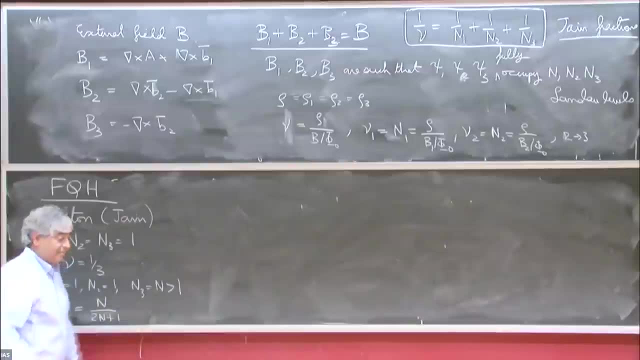 and figure out the edge state theory, the statistics of the bulk quality particles and all of that. Just take that theory, look at the fermions and look at the edge states, just repeating what we did for the integer quantum Hall state, but now with this gauge fields and so on. 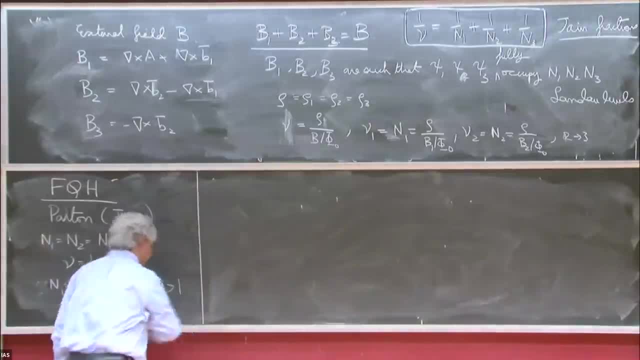 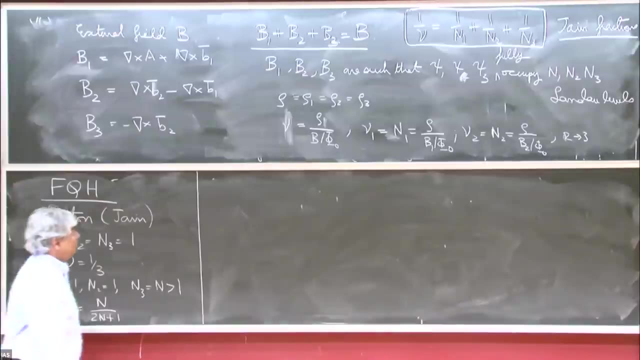 But let me mention here- maybe I'll say a little bit about that next time and then we'll be done- But let me mention here another very interesting case where you get some new types of states which have no analog really what we've talked about so far. 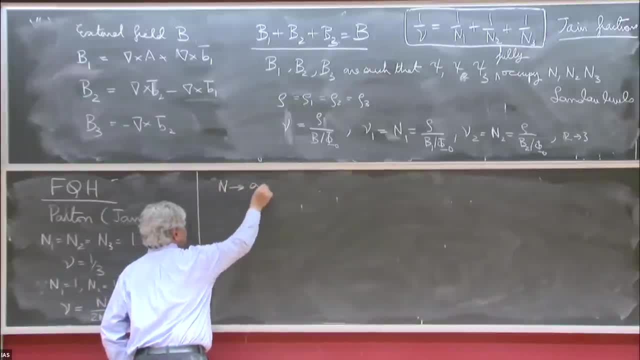 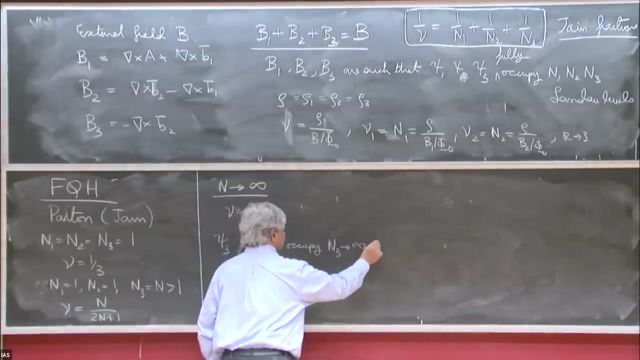 So the point case is: n goes to infinity. What does that take? The n goes to infinity, And so your nu then becomes one half, And what this means is that the side three fermions occupy n3 infinity Landau levels. And what does that mean? 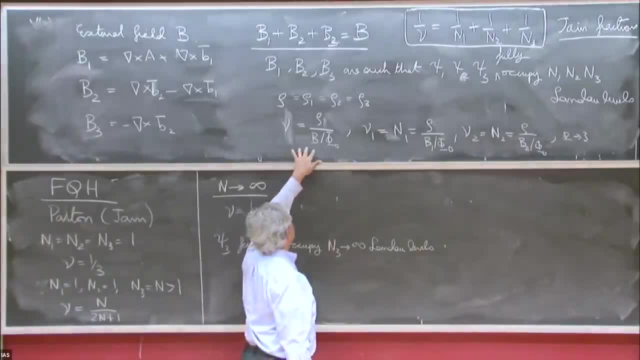 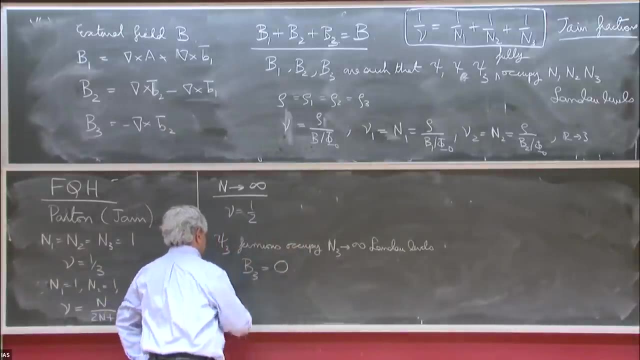 Well, really, if you look at this formula here, if you're filling integers going to infinity, well, the way it goes to infinity for a fixed density is your B field is going to zero. So that means B3 is zero, And so the side three fermions. 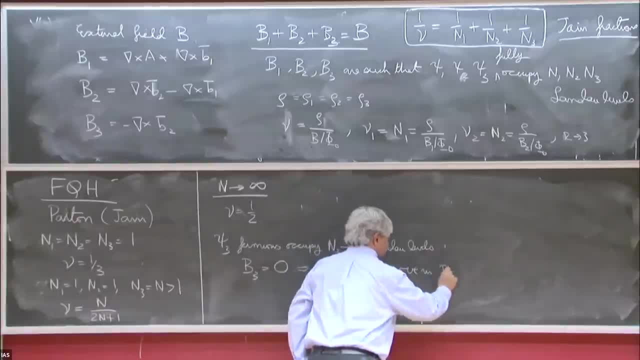 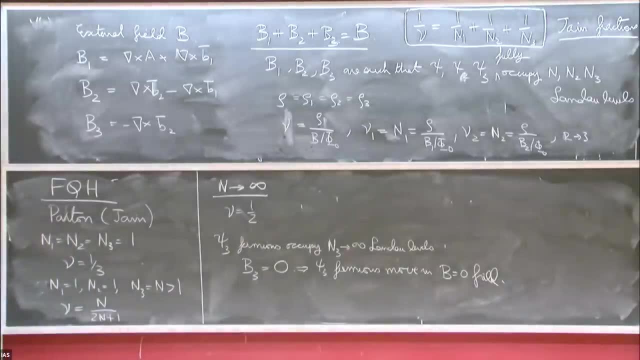 move in zero field, And so the side three, fermions, move in zero field. This is a whole new ballgame. What do fermions, when they move in zero field? do They form a Fermi surface. That was chapter one of the course. 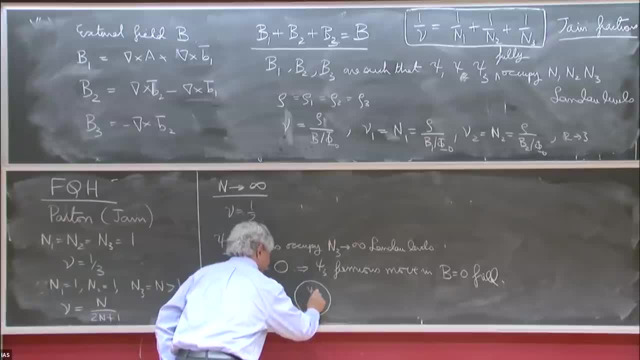 So we would expect the side three fermions to not fill Landau levels but will form a Fermi surface. So this is some Fermi vector here, kx and ky, And the volume enclosed by the Fermi surface. these are spinless. 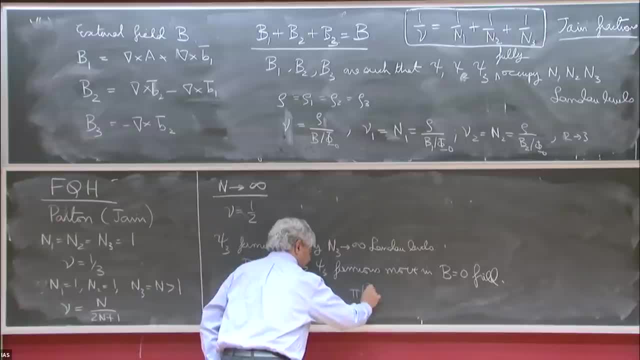 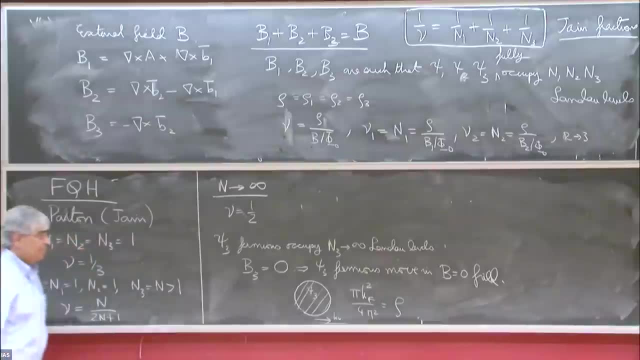 Well, that's pi kf squared 4. pi squared is going to equal the density of electrons, because the density of electrons will equal the density of side three fermions. So this is potentially a dangerous thing with the logic of what we've been talking about. 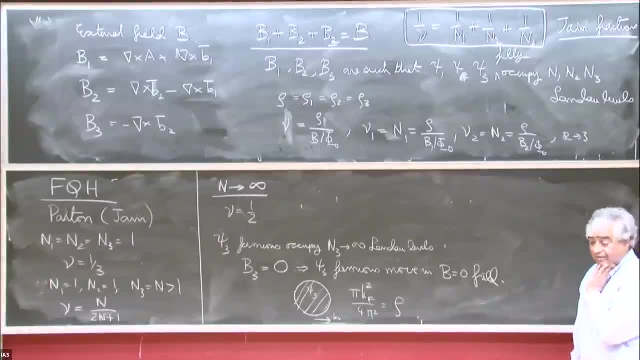 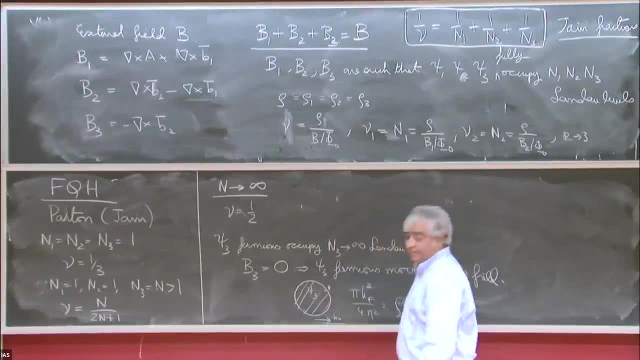 in the sense that the side three fermions no longer have a gap. So now you can take a fermion from inside the Fermi surface and put it outside with arbitrary low energy, And so it's a gap. that's unlike all the states we've talked about so far. 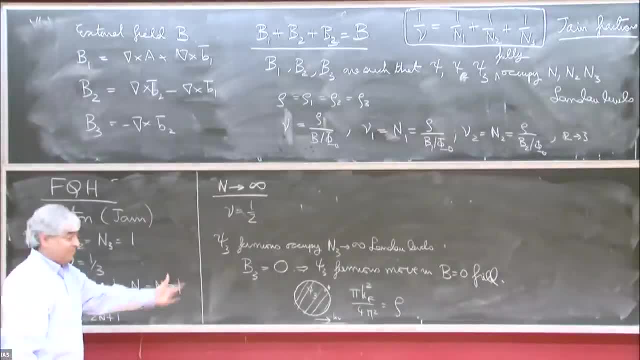 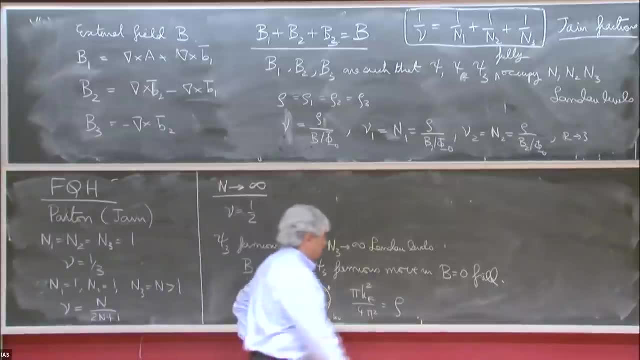 but at least in the bulk had a gap. This doesn't have a gap in the bulk, Okay, but now there's actually quite a lot of good evidence that this state is seen in experiments of the Halpern-Lee restate to the HLR state. 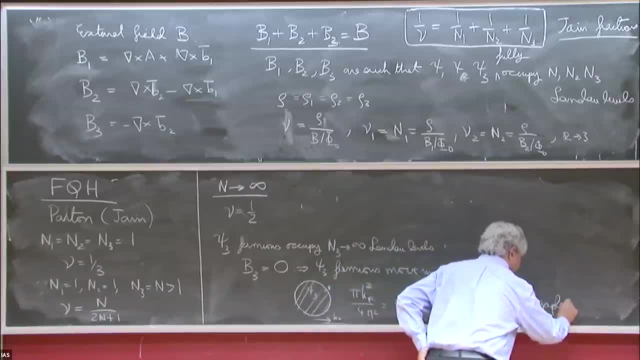 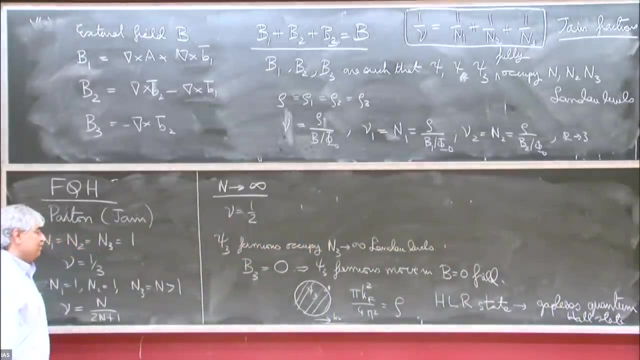 And it's a gapless quantum Hall state. Well, the whole procedure of edge states and so on doesn't really quite work here because you have gapless expectations in the bulk. But nevertheless, the gauge field approach, you know, has seen a lot of. 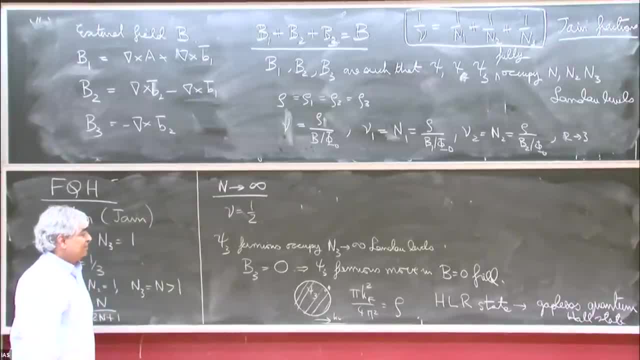 in fact does work as we understand today. The gauge fields do have very strong effects now on the bulk and they change the spectrum of these particles And you get what we call a non-Fermi liquid. It's not a Fermi liquid like we started out with. 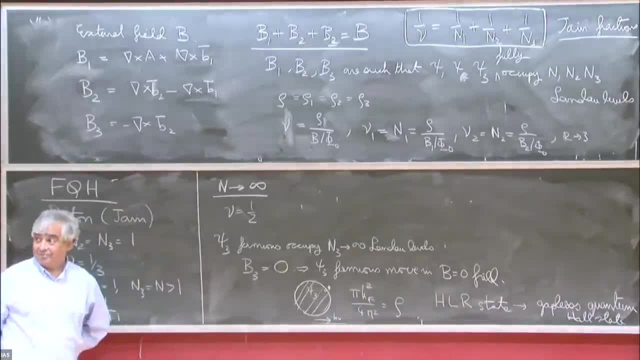 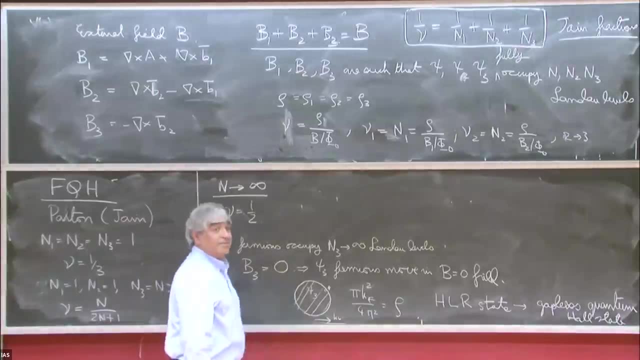 And this is a topic that I will cover towards the end of the course, But this is one way. you get a problem of fermions coupled to a gauge field. The gauge field here is what you call B2? Yes, So what will happen is: 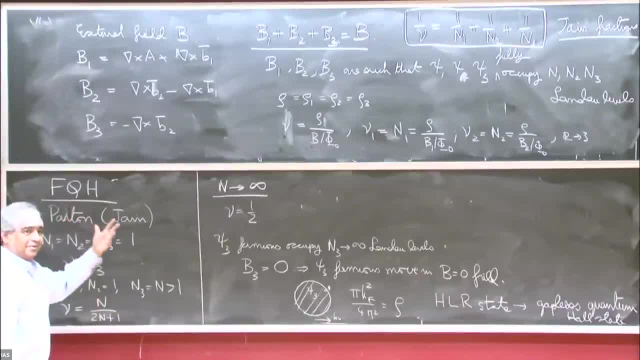 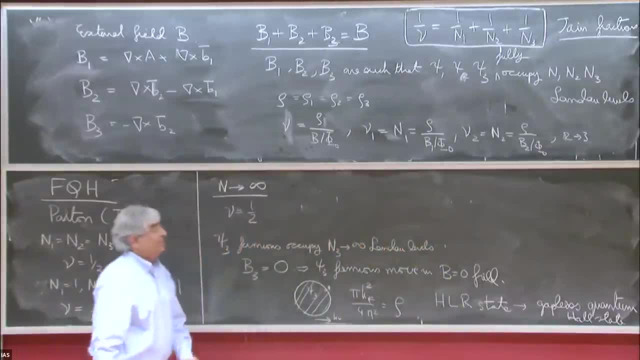 yeah, the B1, you can integrate it out, OK, so this is another important point. In reality, there's really two gauge fields: B1 and B2. And they have- B1 will have- a Chen-Simons term. 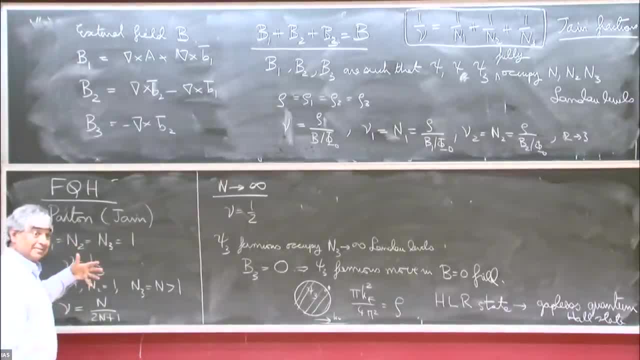 that you can get from integrating out N1, the psi 1 and psi 2 fermions. Now, if you integrate out B2, which formally you can- then you'll end up getting Chen-Simons term with the improperly quantized in the bulk. 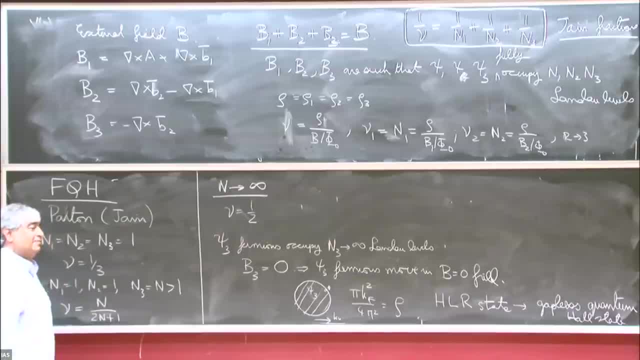 So if you want to work with just one gauge field, then you have a Chen-Simons term. they're not properly quantized. But you can fix that, as you and others have shown, by keeping more than one gauge field, And this formalism automatically gives you. 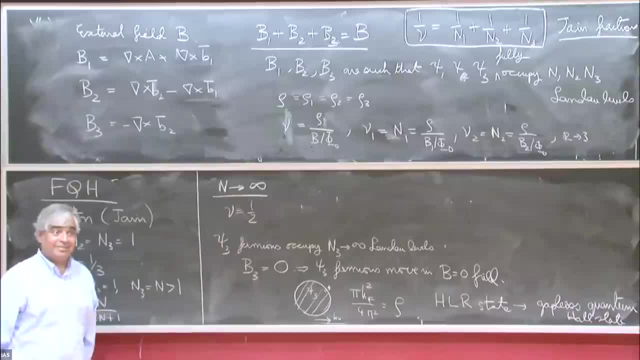 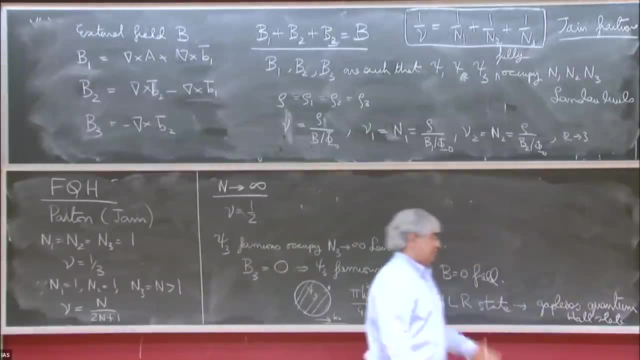 the right number of gauge fields. you need to get everything properly quantized. Well, for this problem. since there's no charge, there's no gap in the bulk. maybe it's not such a big sin to just work with one gauge field, because you never have eight states. 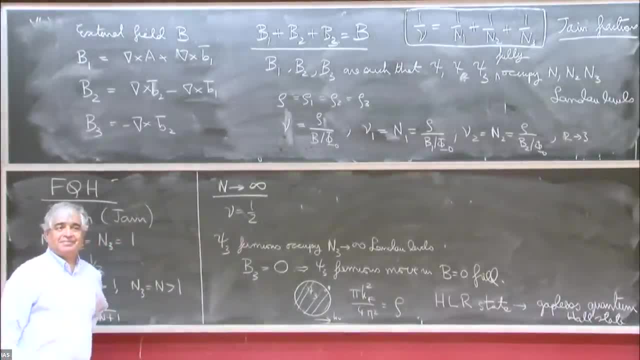 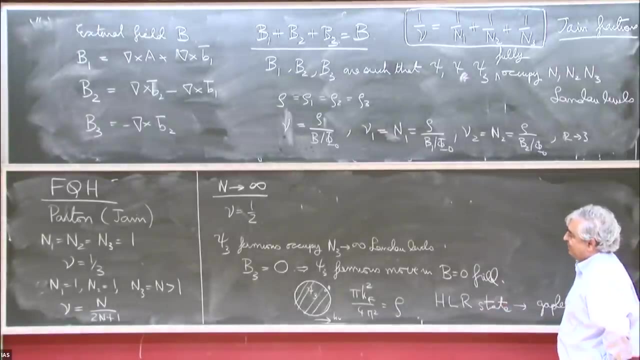 or anything like that. Everything's really in the bulk. I don't know. Did you disagree with that? No, Okay, All right, Great Okay. So you have fermions in a zero magnetic field here which clearly form a Fermi surface. 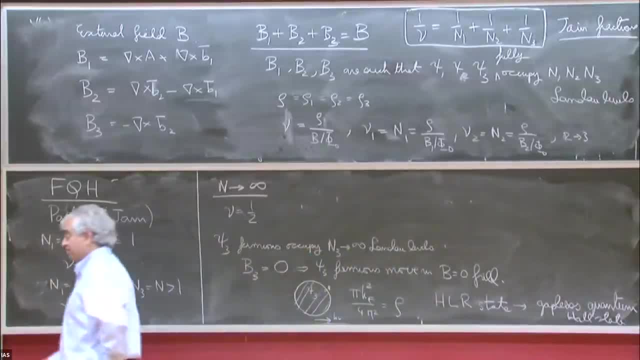 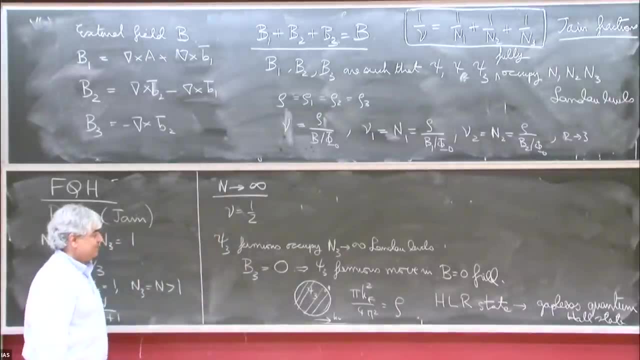 And then you see something you know. there are very good indications, in fact, of this particular Fermi wave vector, measured in various experiments. In fact, here at Princeton, this equation is observed to be okay, rather accurately in observation in this state. 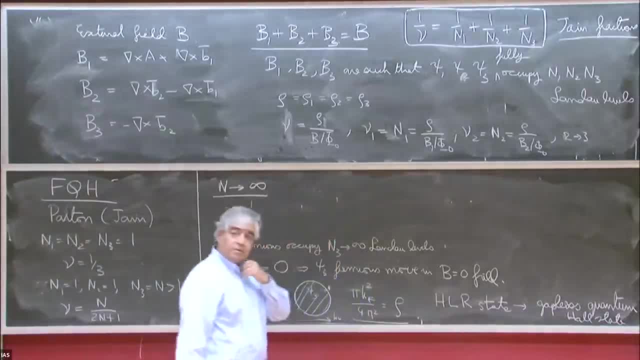 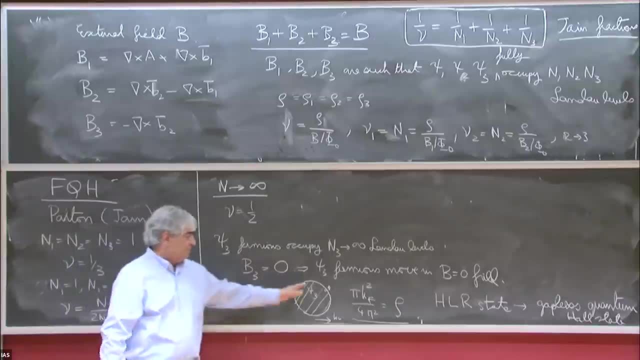 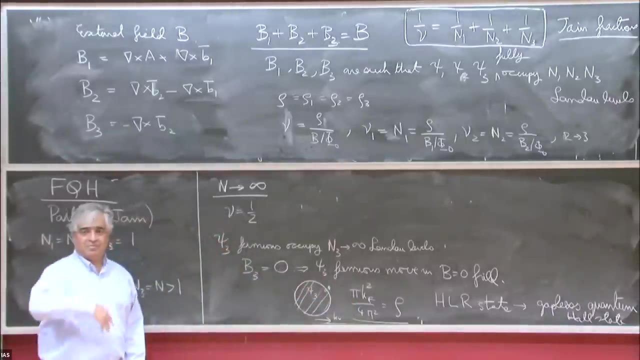 How do you see the Fermi vector? So you have to put an external perturbation which oscillates in space And if it has a wavelength which matches this gap, you observe some sort of resonance. So you do a surface acoustic wave which has a certain wavelength. 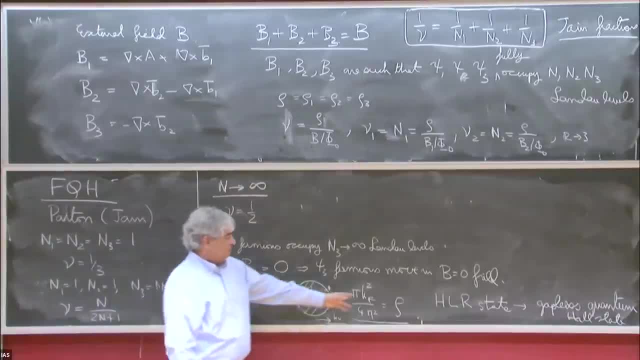 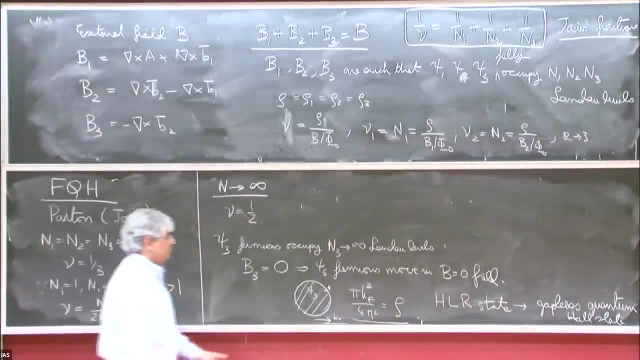 and the wavelength of the wave matches this wave vector, you see an instant response, and so on. Yeah, they're very clever experiments and you can. The point is that these KFs are relatively small, because the density in these 2D electron gases is quite small. 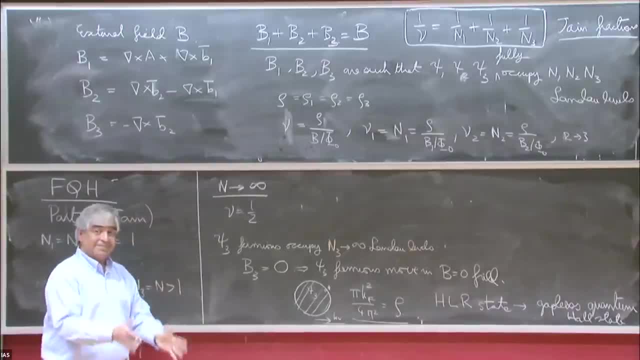 For a KF and an electron gas. in the real material. that kind of experiment would be impossible, because the KF is way too large, The wavelengths are very short, But these densities, these wave vectors are, you know, thousands of atomic spaces. 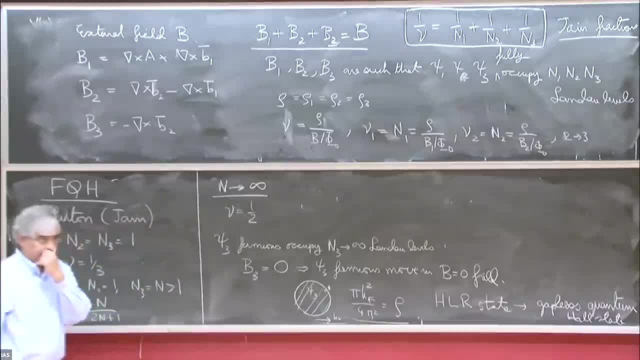 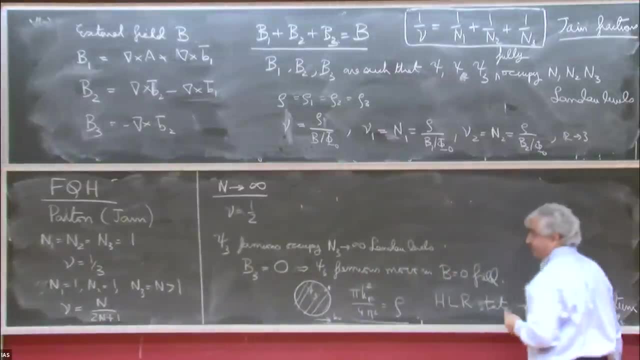 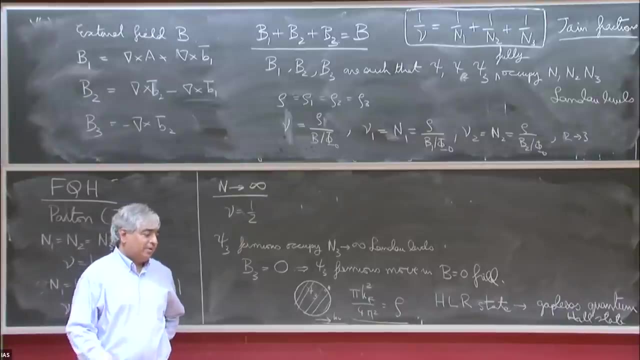 so it's easy to measure them Because of the way these 2D eggs are created. Maybe 100, sorry, That's driven by the applied physical dynamics, right? Yes, but also the way you create these 2D eggs is by doping: gallium arsenide. 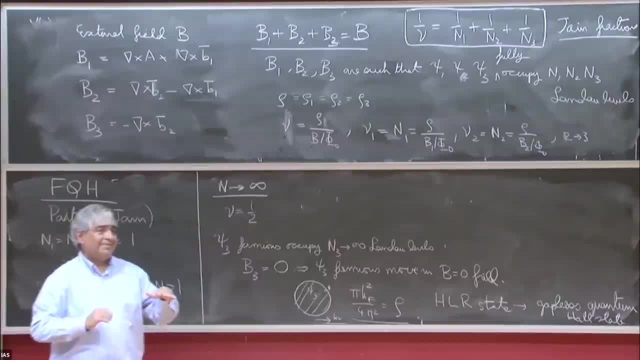 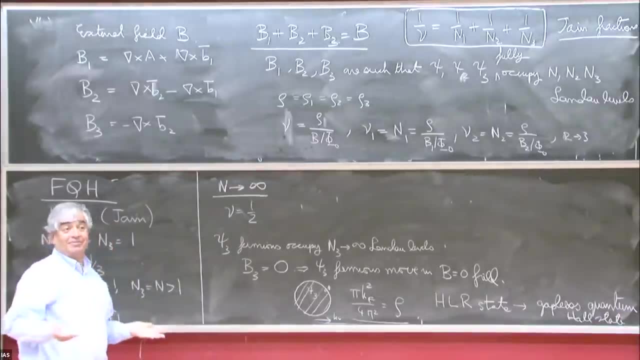 and the dopant density is rather low. It's a very small set of dopants, so the density of the electron gas is small. And then you need that also to fill the nitrogen number of landowners, Because if you took electronic densities that you would get in a crystal like cuprates. I think you would need hundreds of Teslas- No one can achieve those- to get anywhere close to the quantum origin. So all of those go together to make this experiment possible. The low density and the relatively small magnetic fields that you need to impose to see highly quantum effects. 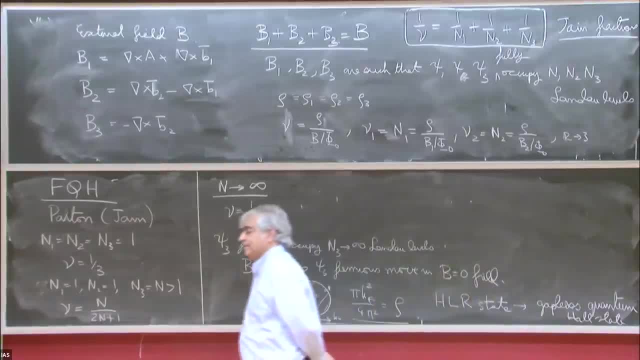 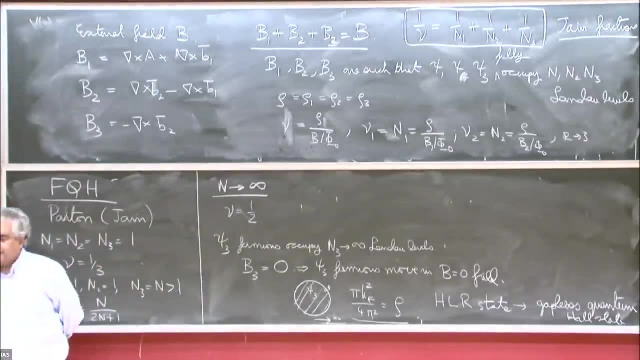 Did I understand? Yeah, You said that the Fermi liquid picture of this stage is not exactly correct, because the interactions are important, Absolutely. yeah, So that's right. So that's a good question. So what do I mean by a Fermi surface? 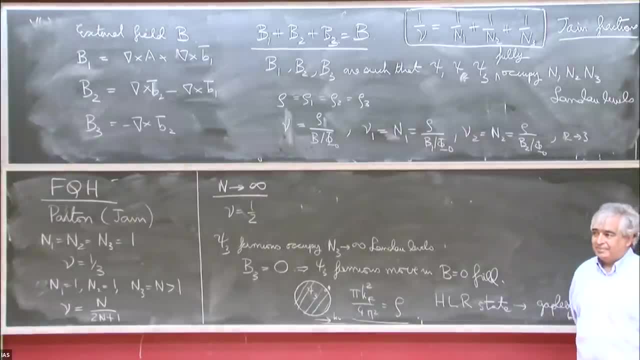 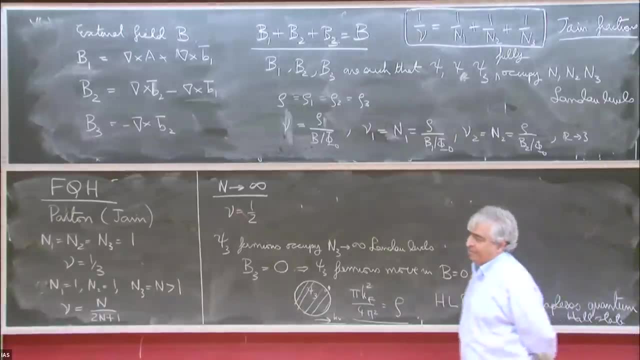 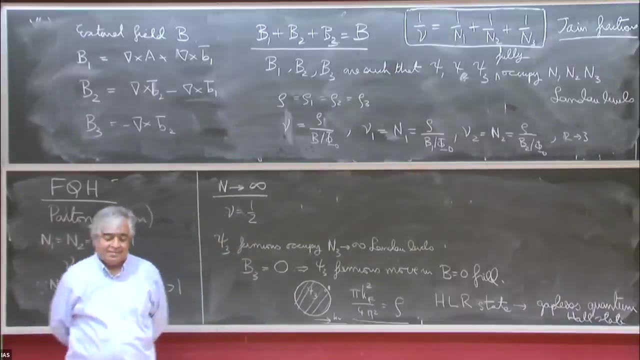 Well, we introduced a Fermi surface for a free electron gas as a jump in the momentum distribution function. Then we found it's also specified for an interacting gas. It's just the size of the jump becomes smaller. In this case there is no jump. 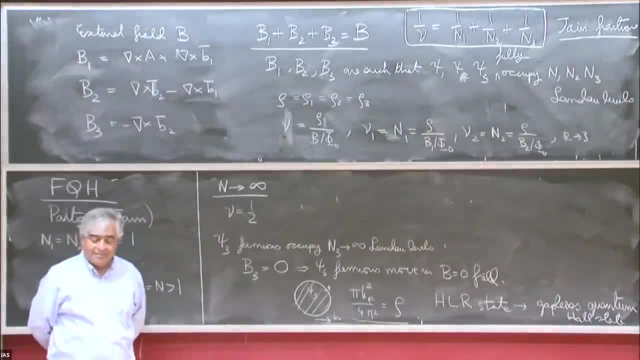 in the electron momentum distribution function. But there is a kink, There's a non-analyticity. So what happens is that, roughly speaking, the gauge fields leads to a breakdown of the quasi-particle idea in energy space, sort of like. 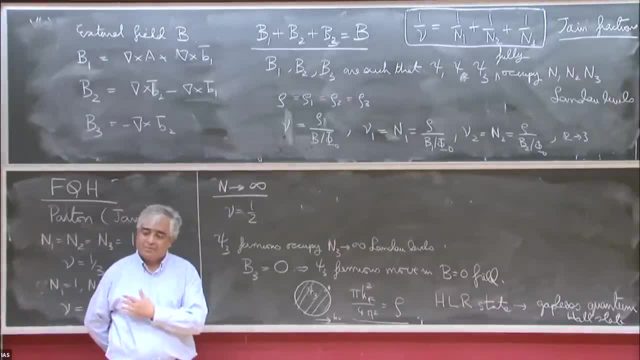 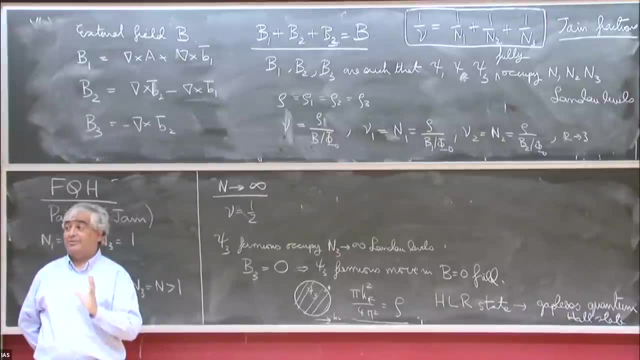 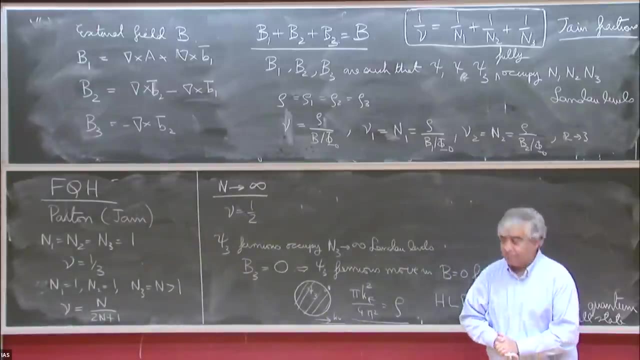 very much like the SYK model. You get no quasi-particle excitations, But nevertheless they're sharp enough. The idea of a Fermi surface is still well-defined, Because what happens is you have these excitations that are not well-defined. 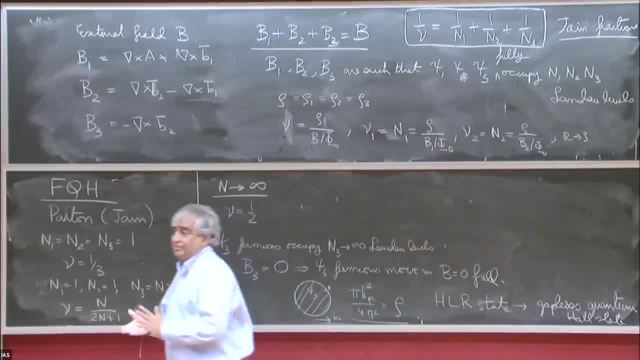 but they do have a definite charge. They're either quasi-particles or quasi-holes, And the locus of points in momentum space where the excitations change from quasi-hole-like to quasi-particle-like is the Fermi surface, Even though there are no particles. 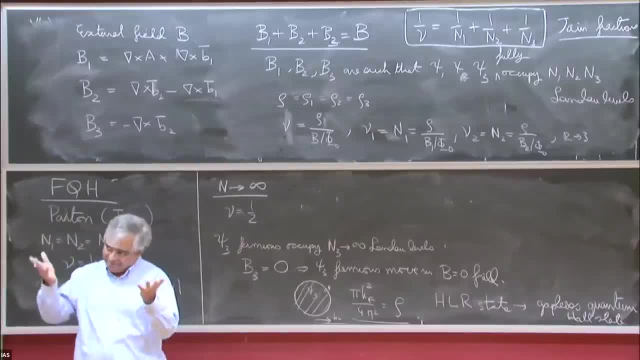 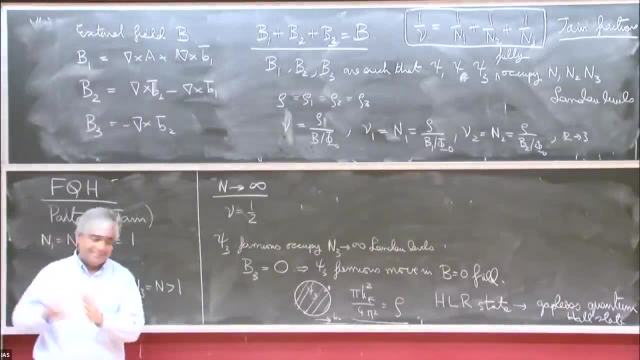 the Fermi surface is sharp. Yeah, This is going to be a topic that I will say much more about. Yes, That's why I want to move on to other things, to eventually get to this. Yeah, I once heard that this state. 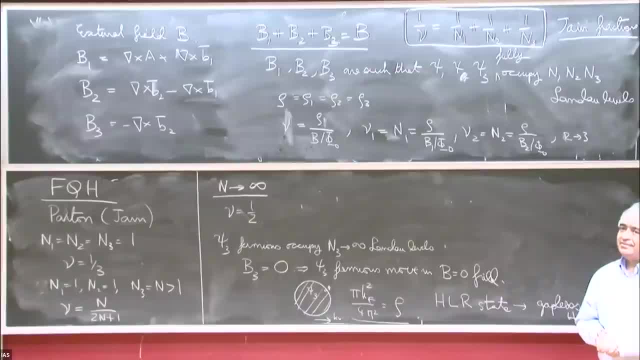 is supposed to be described by a free, massless fermion, Is that No? Well, I mean, you know you can make an approximation and just treat it as free, but no, ultimately the quasi-particles are. I mean. 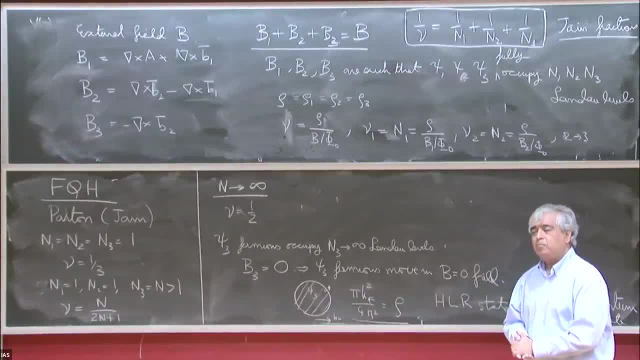 Ah, okay, But it's a statement that there was some CFT and then the CFT was Maybe I'm just remembering. No, No, I don't think so. This is definitely. The closest thing to this is an SYK model, actually. 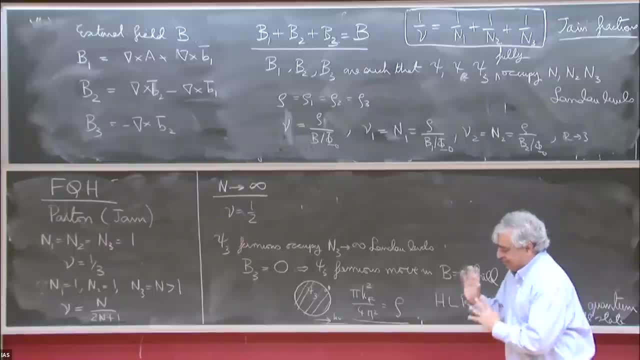 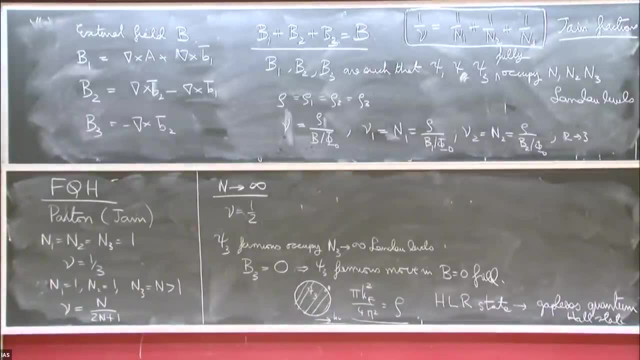 It's strongly interacting, as strongly interacting as the SYK model, But it nevertheless has some sharp structure in momentum space which you can investigate experimentally. Okay, Well, I guess I will have to talk more about this. Okay, Thank you. 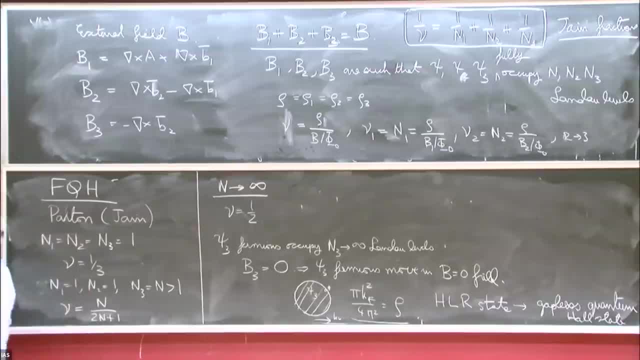 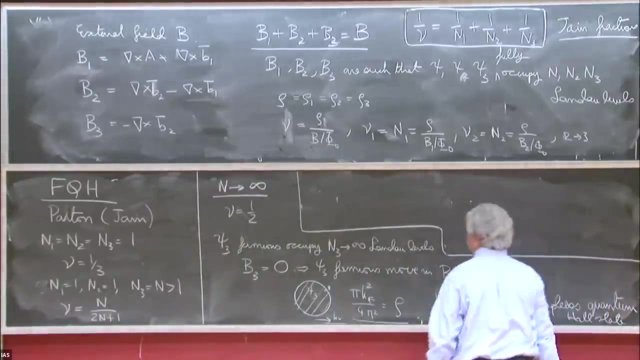 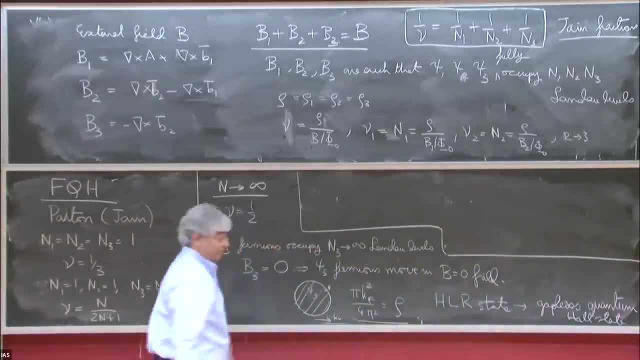 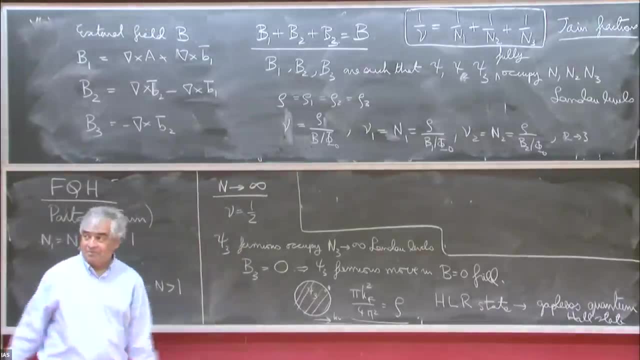 Okay, So one of the things that I wanted to talk about next, which is also a lot of fun, but it's something we can do next time. So another possibility for fermions when we go back to the beginning of the course. 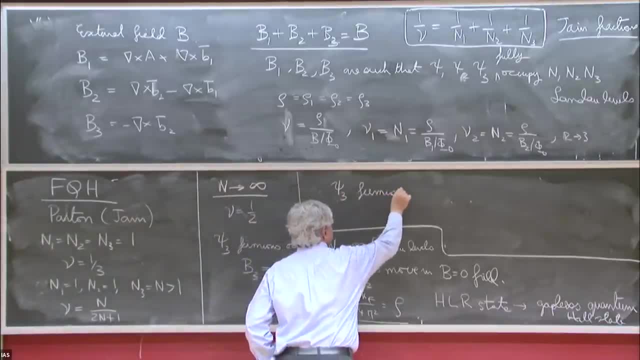 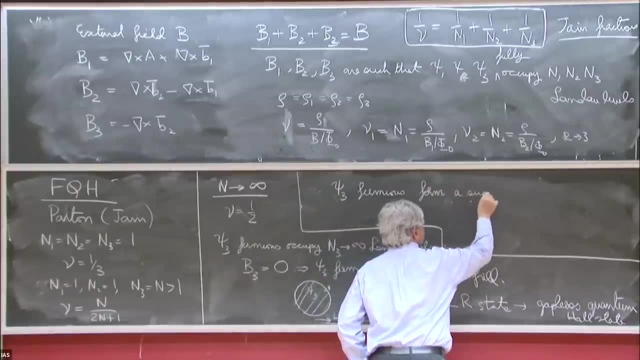 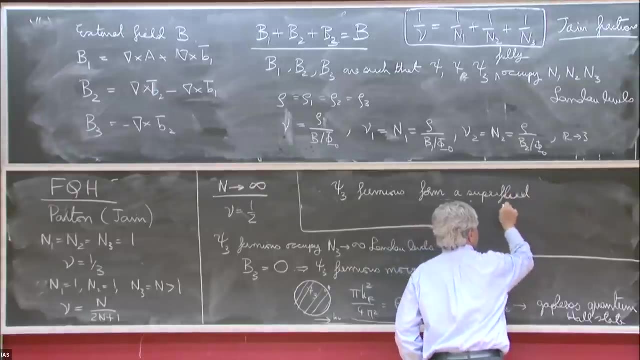 they said: fermions form a Fermin surface. Great, But what else do they do? Well, Let me call it a superfluid, because, yeah, I'm a superfluid. Which means that psi 3 of p, then the condensate of psi 3 of minus p, which is not equal to. 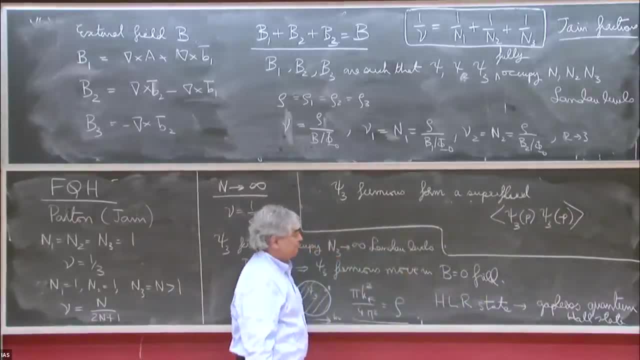 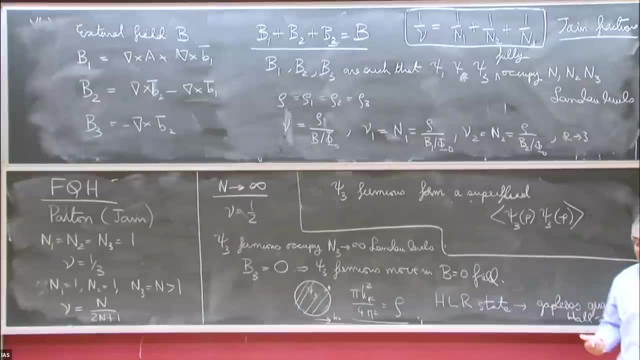 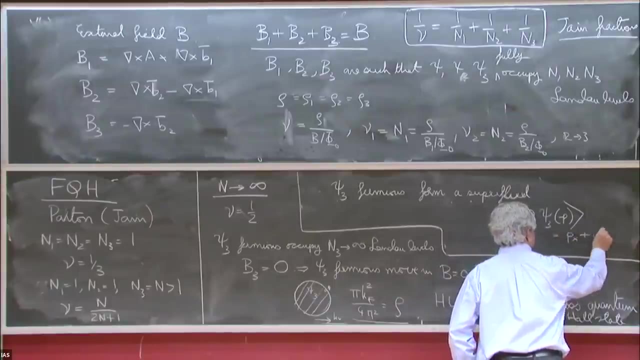 zero. Now, since there's no spin, this has to be an odd function of p. So it's not a d-wave superconductor, which is even function of momentum. it has to be a p-wave superconductor And, in particular, if you take what's called a px plus py superconductor, it's of this. 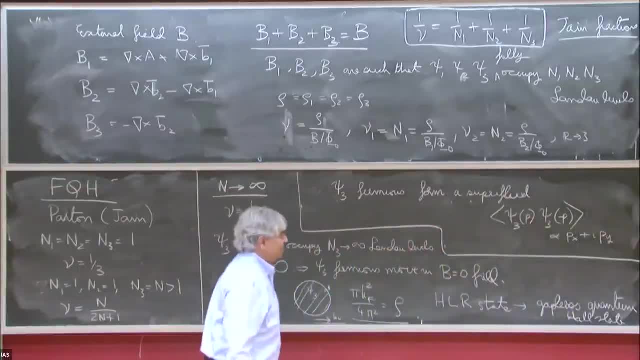 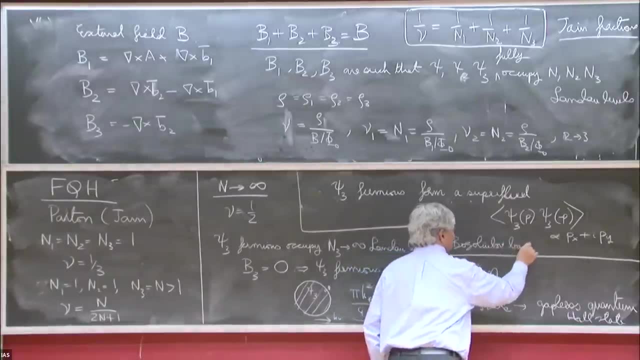 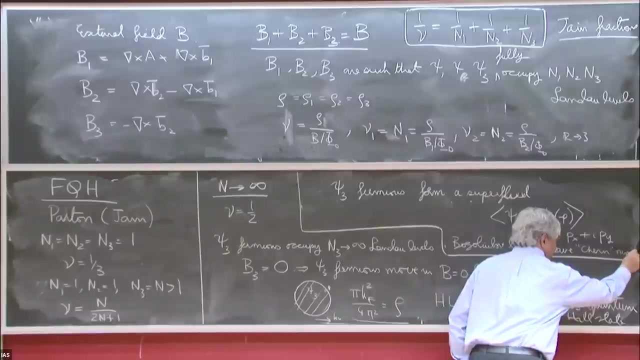 form, then the Poincare bond bands of this superconductor, which, again, you determine them exactly like you've done in previous chapters. They turn out to have a charge. I'll put churn in quotes, but it's really like half a churn number and I'll talk about 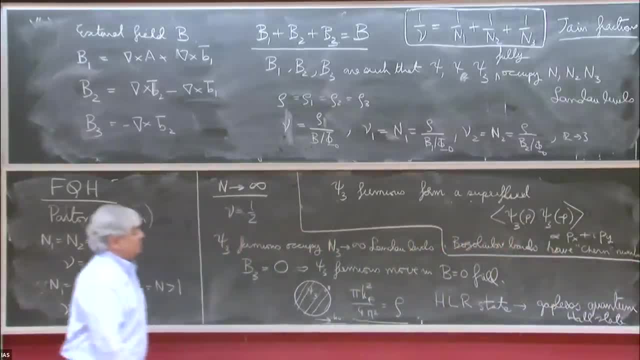 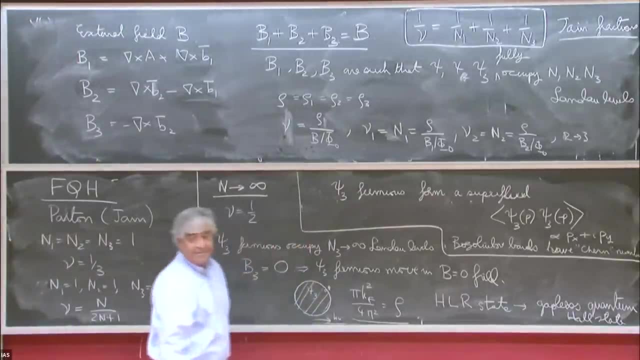 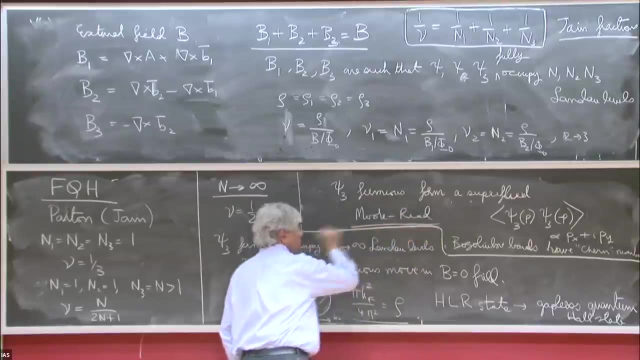 this next time. So now you get a different type of topological state, but you're pairing of these four neurons and the bands have a churn number And that's what leads to a non-abelian state, in this case, the more real state. 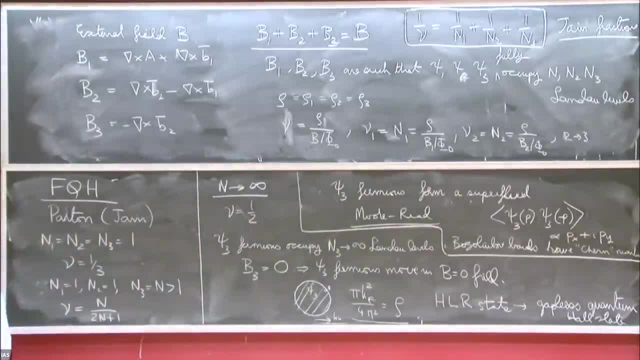 Okay, and you can get again. put this in And you just go through all the tricks you have learned. you will get all the right properties in the more real state. I'll say a bit more about that next time. What determines whether it's superconducting or not? 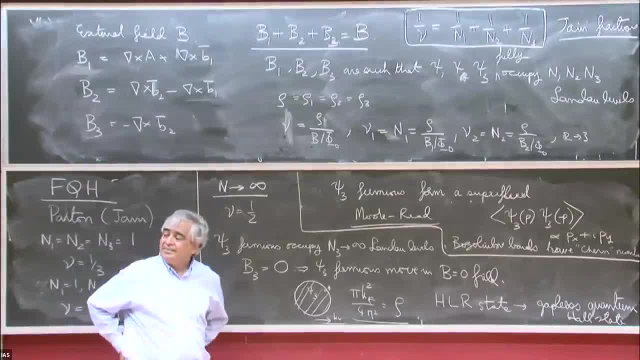 Okay, It's definitely not a superconductor in the sense that you won't see a persistent current. Yeah, yeah, These things, Yes, You know. again, that depends on details. So there's some interactions between the fermions. 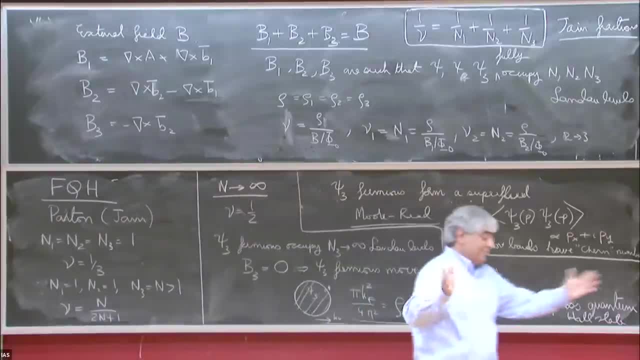 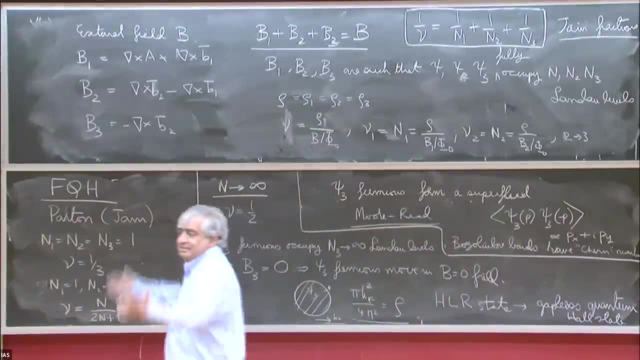 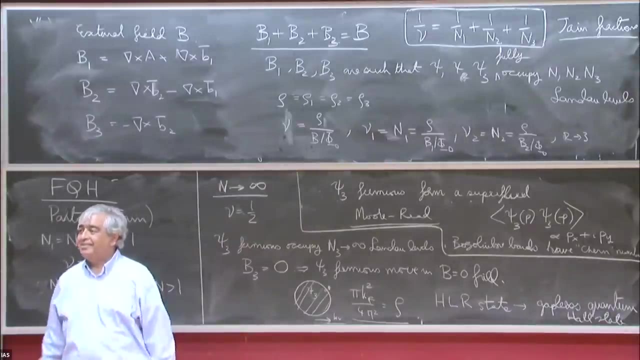 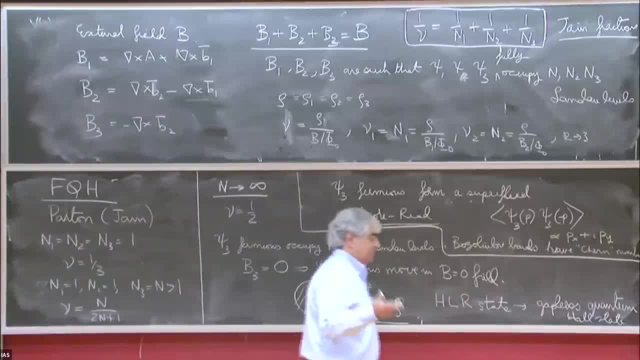 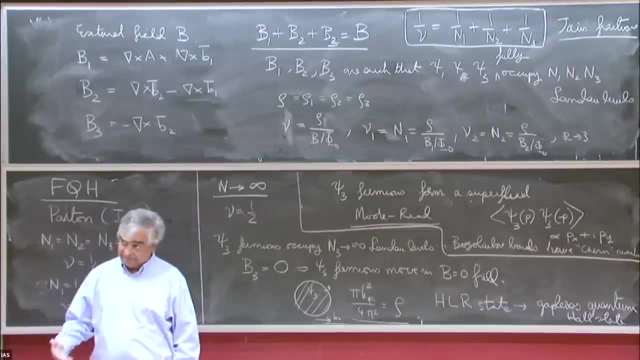 Is, there is an attractive interaction. So there is something called the PCS in stability that you know what we learned about, which applies for S wave pairing when you have time. reversal symmetry When, no matter how weak the interaction, as long as there's one, there's an instability. 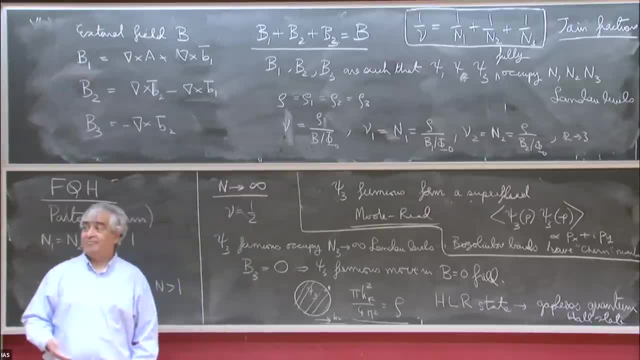 to surfactant state. There's no such theorem here. but when you're broken, time reversal, So you need some appropriate interaction. So okay, And in fact it seems to happen in certain situations, not just in Gallimard site but also in graphene in recent years. 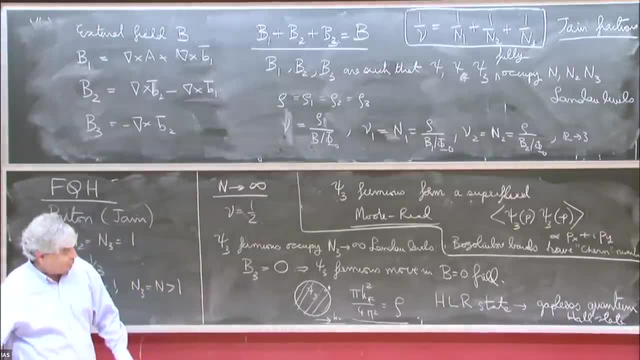 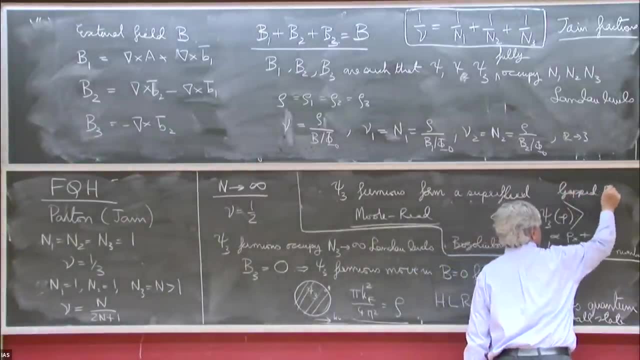 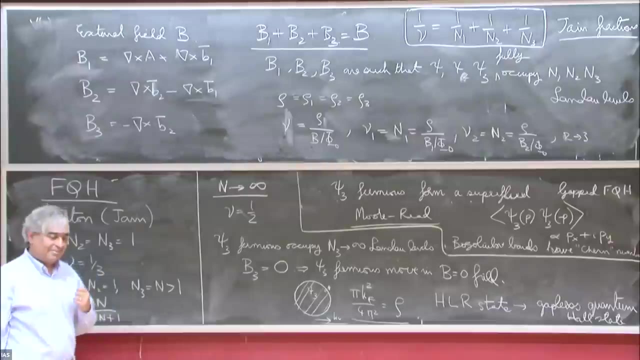 We do see. so this is now a regular fractional quantum Hall state in the sense that it's gapped. So this is a gapped FQH, It's fully gapped. There will be edge states and the edge states, because of this boggle above churn number, have Majorana fermions. They're not complex fermions, they're real because of this pairing. essentially, 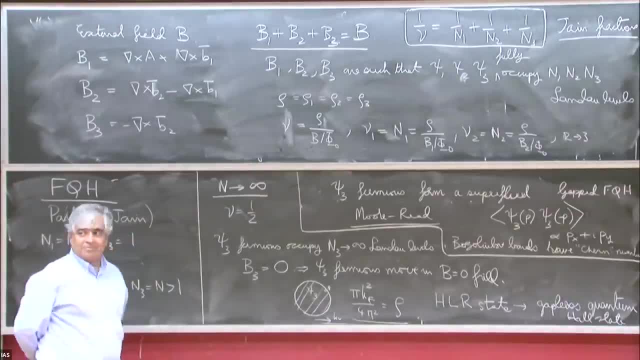 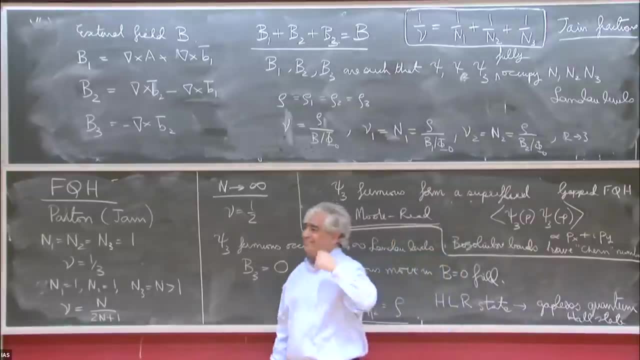 And the Majorana fermions is what leads ultimately to more, to knowledge of the non-obedient statistics appears from the fact that once you have a superfluid, you also have a vortex. So the vortex in the superfluid is a non-obedient. 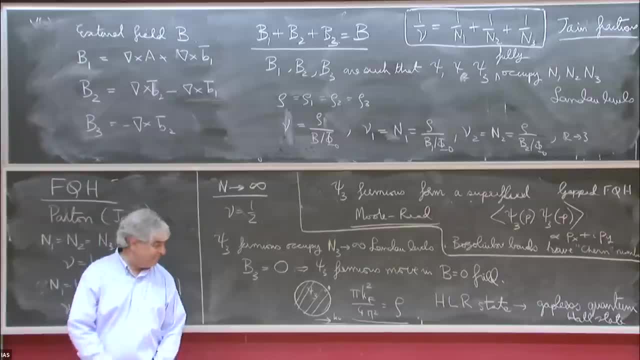 So the vortex in the superfluid is a non-obedient quasi-particle. Has this state been observed experimentally? Yeah, well, okay, There is a fractional quantum Hall state observed at nu equals one half. The more reach state is the simplest possibility, but there are about three or four others. 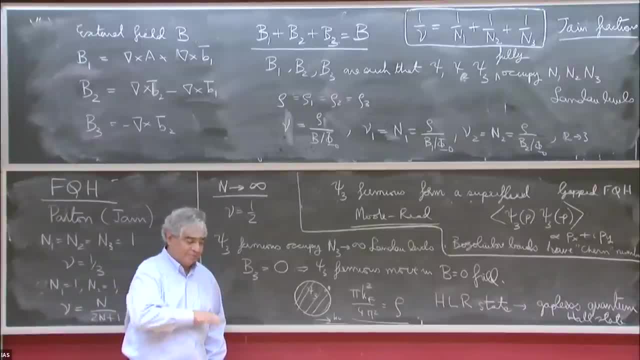 And I think I'm not an expert on this. this is a topic of, you know, very hard current research. I don't think it's particularly been decided Which one This is the right one. It may be more read. it could be something else. 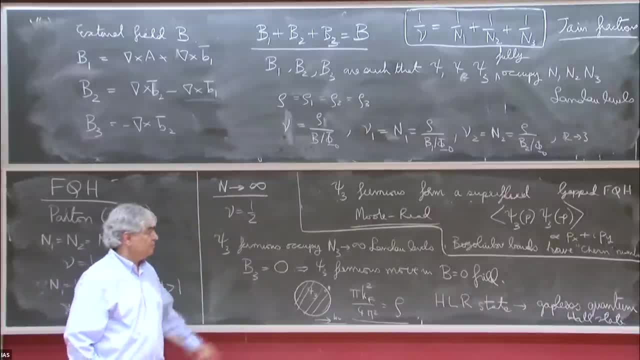 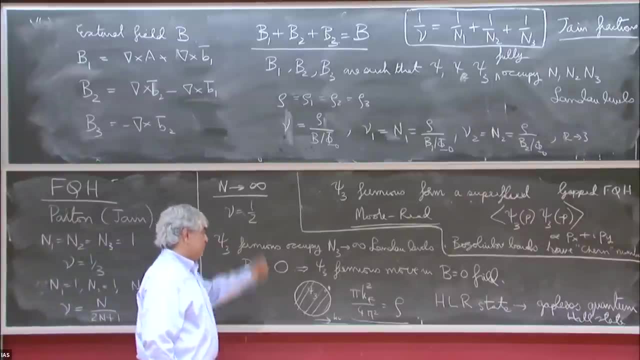 I see. So some materials will give you the new one half that you said before with master: Yeah, And other materials will give you the new one half- Yeah, I mean, it could also be that you went to very low temperatures. every material will go to this. Or some temperature range. you could ignore the pairing and you see the HLR state. But at low enough temperatures it could well be everything will be compared at somewhat tangle. But yeah, There are a bunch of other states, more complicated states, which have also have Majorana edge states. 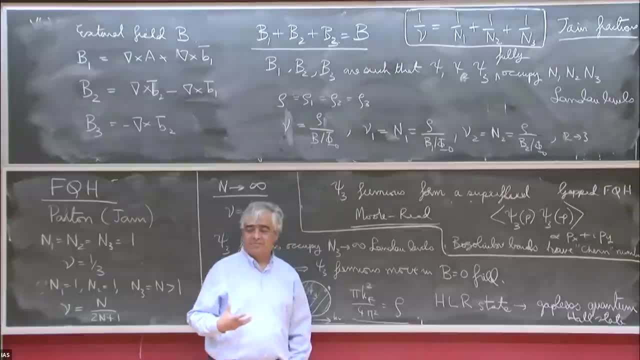 And there's evidence for increased Majorana edge, because that gives you a half quantized thermal conductance, which is been seen. This is a claim. Yeah, It's been seen. But there are also other edge states coming from the Cy1 and Cy2 fermions. 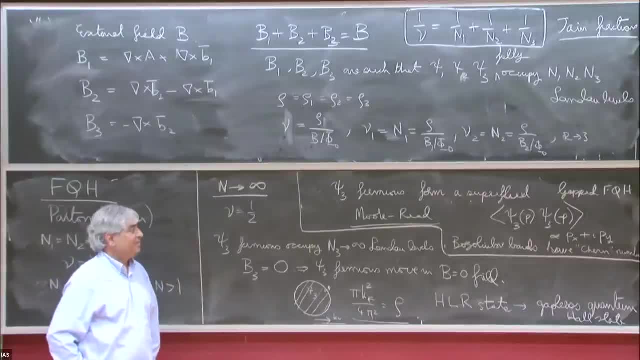 So in this case it's more complicated. You've got a lot of stuff going on And there are other states- Yeah, I am not an expert by them any means, And when I take the current state, As it's not yet clear which one of them has been seen, 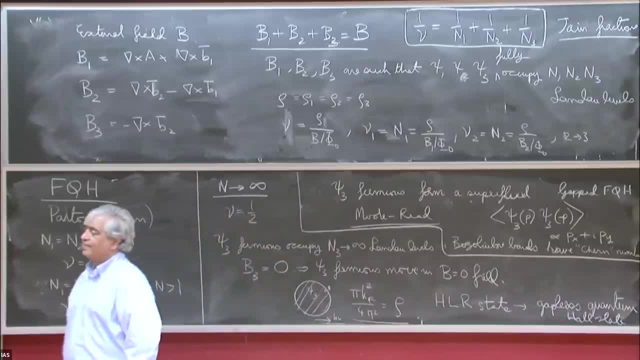 I know that a short while ago, I saw a paper that talked about the half-integer thermal conductivity. Yeah, And I asked Greg whether this was proof that they found the Maurice state and he said no, Yeah, Okay, Yeah. 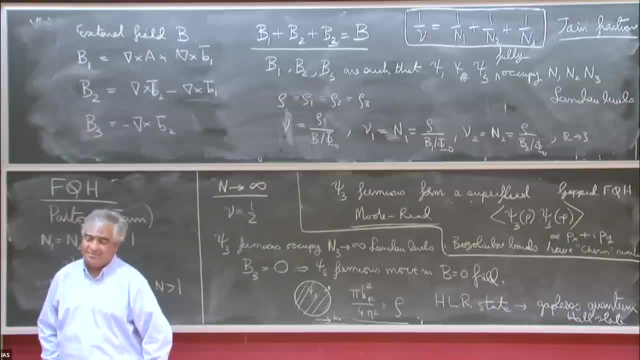 So he's being honest. That's correct. Yeah, That's my understanding too. Yeah, There's also analogs of the pairing in spin liquids, where you take a Z to spin liquid And you've paired this epsilon particles in this P plus IP state. 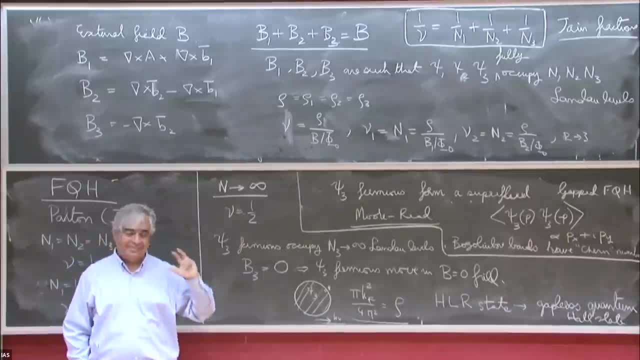 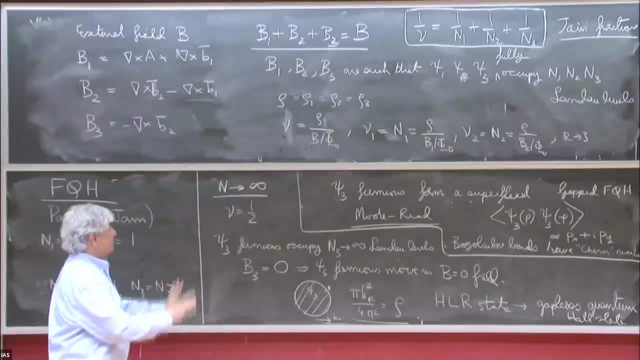 And that's the Keter of non-ABN state, which is similar, but it's edge states are slightly different. Yeah, But everything can be, you know, very compacted, At least these ones, The more complicated ones maybe. 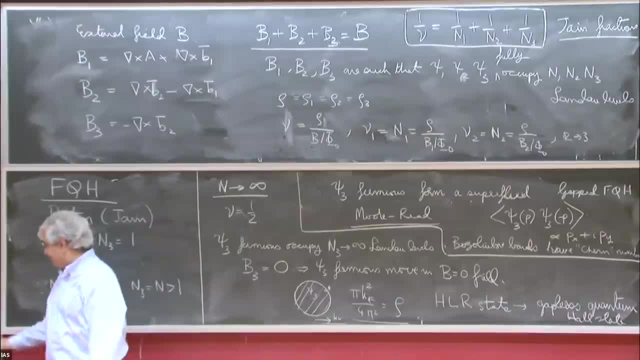 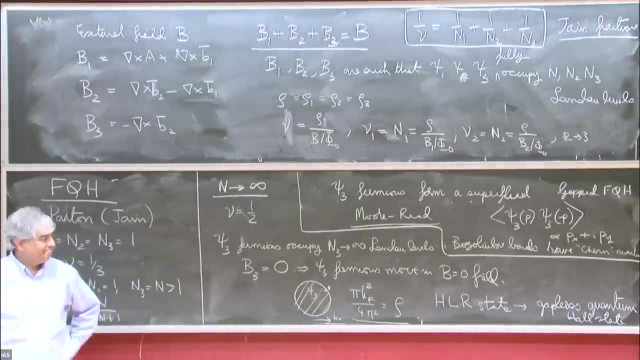 I'm not sure how to get them from the part of the course. Yeah, People are very fancy performing with thin theory ways of thinking about it. Okay, So I've got? yes, go ahead. I just wanted to make a comment. slash question. 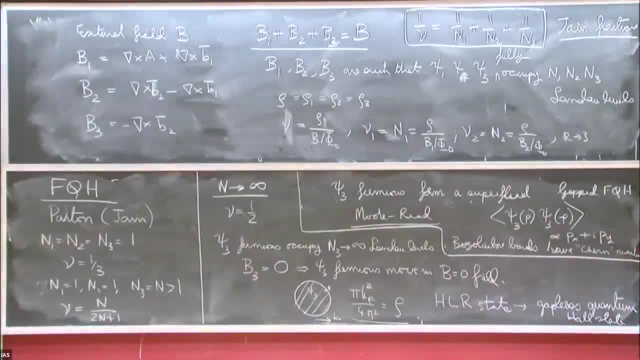 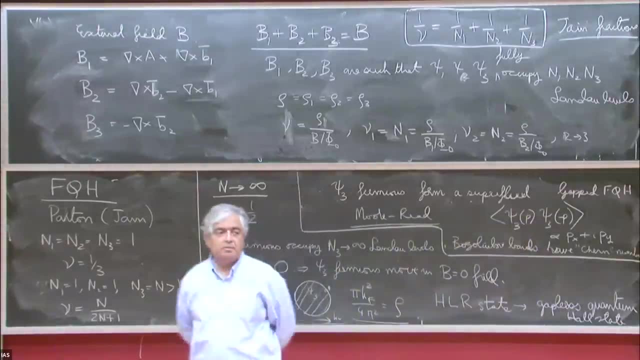 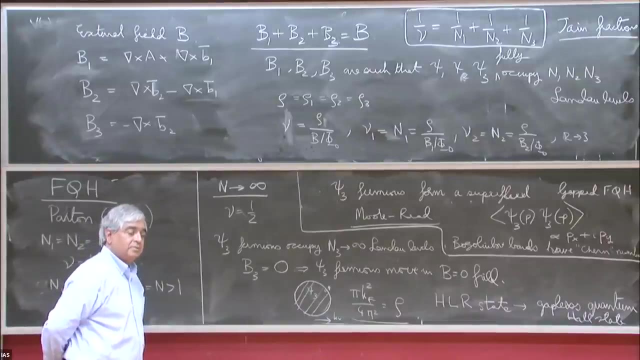 Sure, When you hear you said that the size fill of Ni Landau levels. Yes, I was confused for a bit, but in the spirit of your derivation you could say that if you did, this mean field theory. Yeah, By popping Hamiltonians for the size which would have term numbers. 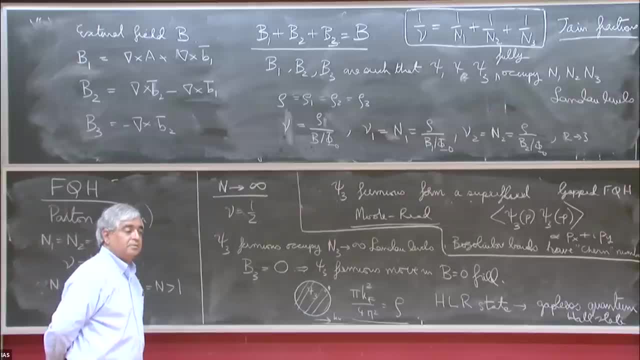 Yes, Ni's could be interpreted as the term numbers of those filled bands, Correct. And then that would answer Tom's question about what the Transignments levels are, because we would deduce them in precisely the way you said the other day, from the numbers of filled bands and from the gauge fields that couple to each species of family.